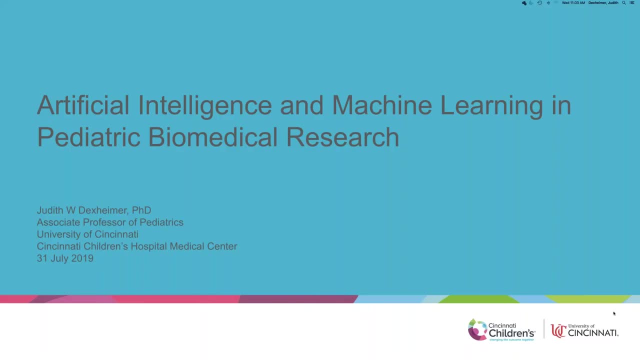 Good morning and welcome to the AWS Education Research Seminar Series. This morning we're going to be discussing artificial intelligence and machine learning in pediatric biomedical research with Professor Judith Dexheimer. Dr Dexheimer is an associate professor of pediatrics at Cincinnati Children's Hospital Medical Center and the University of Cincinnati. 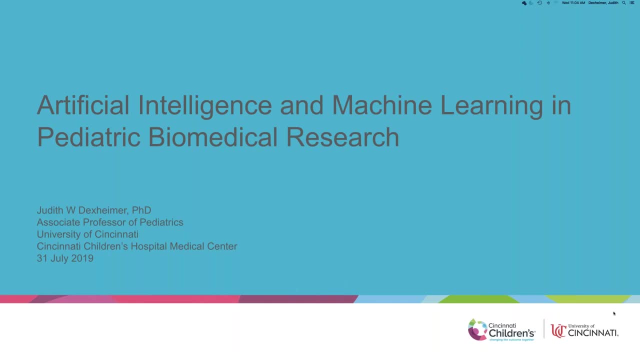 She is a clinical informaticist working on the development implementation of machine learning applications into clinical care. Her research focus areas include machine learning techniques, real-time patient identification systems, disparate data merging and applications of clinical data. If you have any questions for Judith, as she likes to be addressed during, 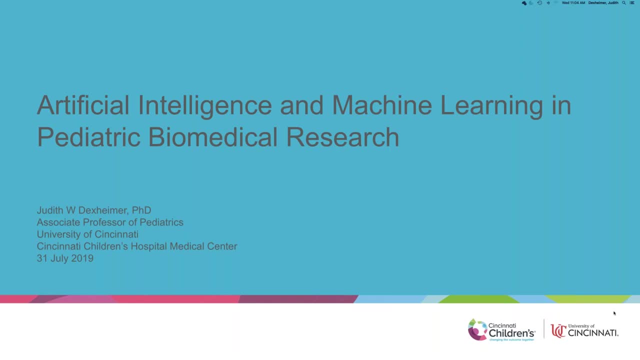 the session. please feel free to enter them into the questions queue on the GoToWebinar tool. We will reserve the last five to ten minutes of the session for a Q&A And, without further ado, I'm going to hand it over to Judith. 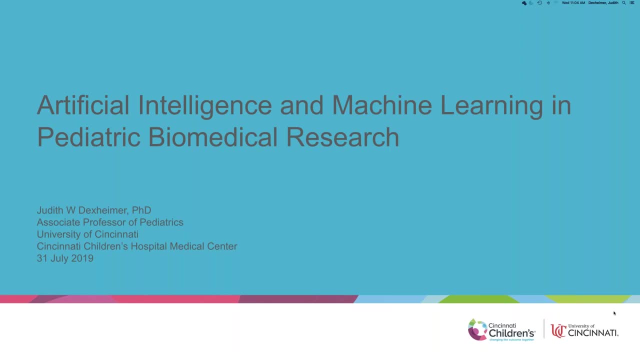 Thank you very much, Marcie. I'm happy to be here today and I'm happy to talk about things. So my goal over the entire presentation- so 45,, maybe 50 minutes- is basically to get you, as the audience, interested in machine learning and informatics. It's a rich field. 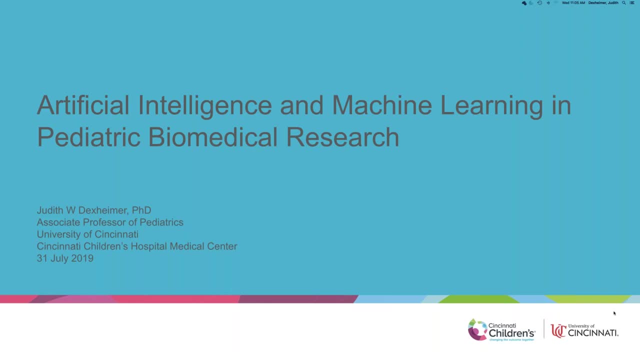 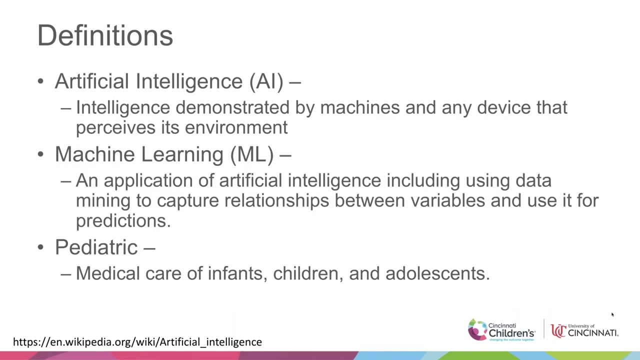 It's got a lot of future with a lot of different innovative possibilities, And I want you to see that it could be a lot of fun and that it would be a great thing to start researching it. So I want to start with basically some definitions. Perfect, So I'm going to start. 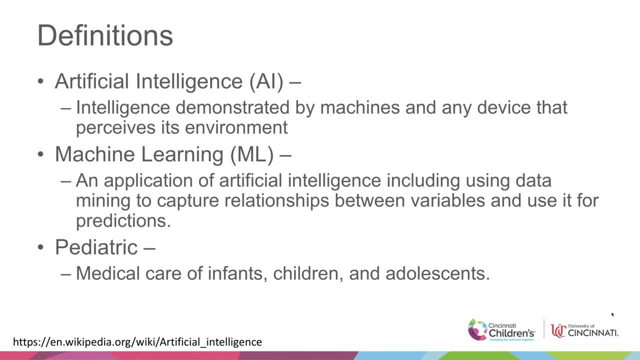 with the title and I'm going to define all of the key terms in the title just to make sure we're all on the same page. So the first thing I want to define is artificial intelligence, So it's basically intelligence demonstrated by machines and any device that perceives. 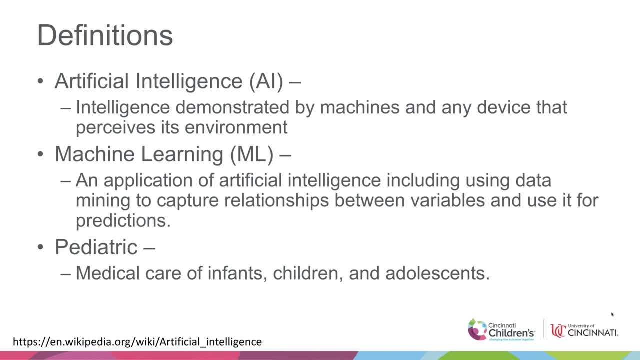 its environment. Machine learning, which is an application of artificial intelligence, including data mining, to capture relationships between variables and use them to make predictions, And these are kind of the main technical terms that we'll go through. And then, of course, there's 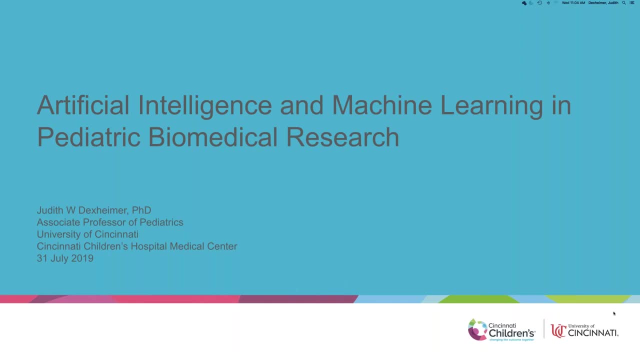 She is a clinical informaticist working on the development implementation of machine learning applications into clinical care. Her research focus areas include machine learning techniques, real-time patient identification systems, disparate data merging and applications of clinical data. If you have any questions for Judith, as she likes to be addressed during, 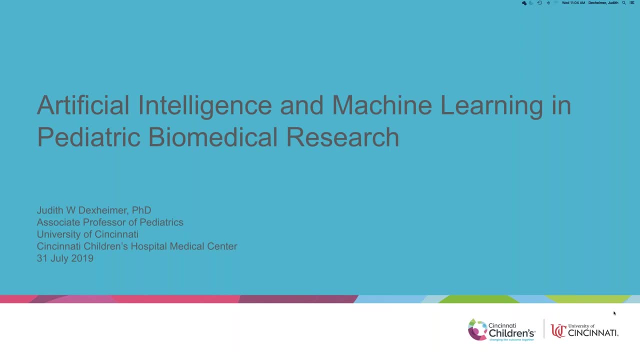 the session. please feel free to enter them into the questions queue on the GoToWebinar tool. We will reserve the last five to ten minutes of the session for a Q&A And, without further ado, let's get started. Thank you very much, Marcie. I'm happy to be here today and I'm happy to talk about. 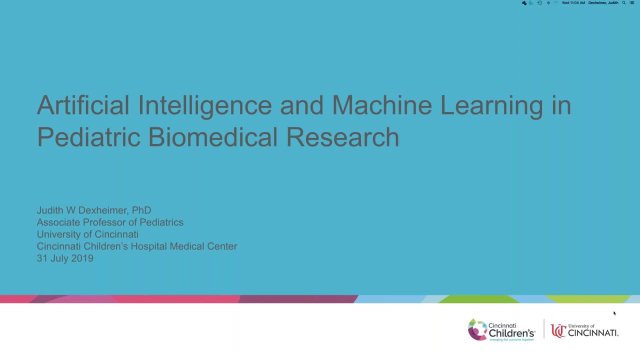 things. So my goal over the entire presentation- so 45, maybe 50 minutes- is basically to get you, as the audience, interested in machine learning and informatics. It's a rich field, It's got a lot of future with a lot of different innovative possibilities, And I want you. 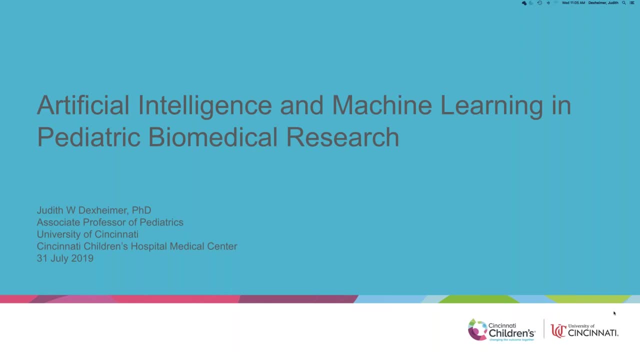 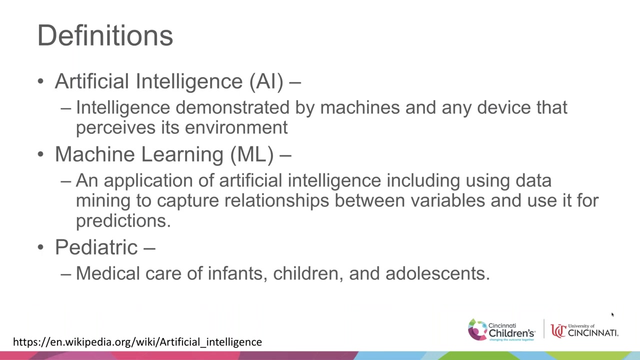 to see that it could be a lot of fun and that it would be a great thing to start researching it. So I want to start with basically some definitions- Perfect. So I'm going to start with the title and I'm going to define all of the key terms in the title, just to make 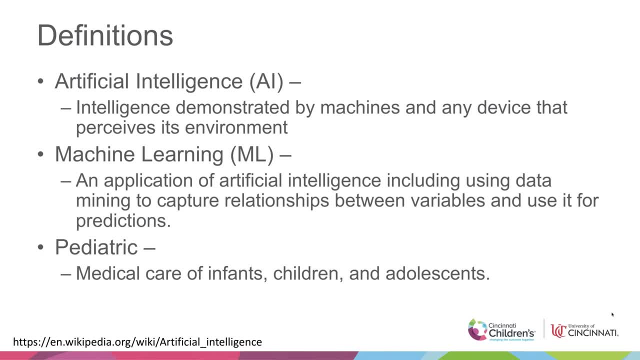 sure we're all on the same page. So the first thing I want to define is artificial intelligence. So it's basically intelligence demonstrated by machines and any device that perceives its environment. Machine learning, which is an application of artificial intelligence, including data. 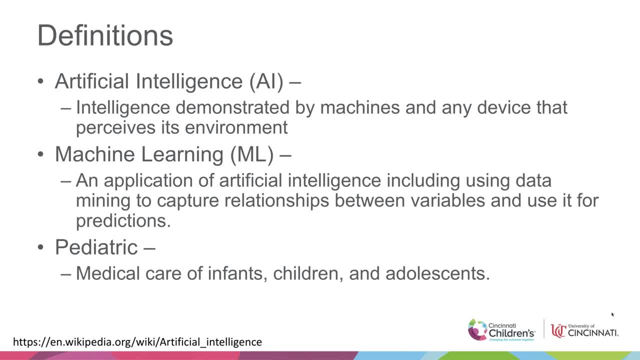 mining to capture relationships between variables and use them to make predictions, And these are kind of the main technical terms that we'll go through. And then, of course, there's pediatrics, which could colloquially be described as everybody under the age of 18.. But really, 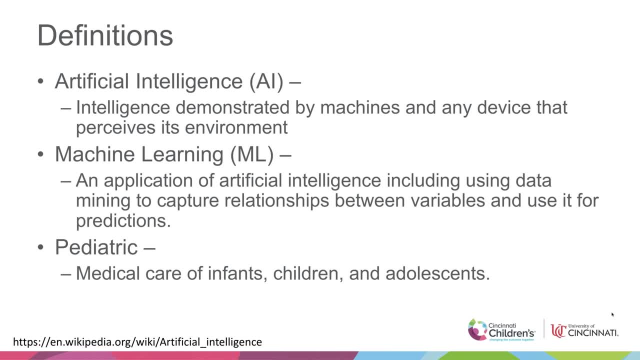 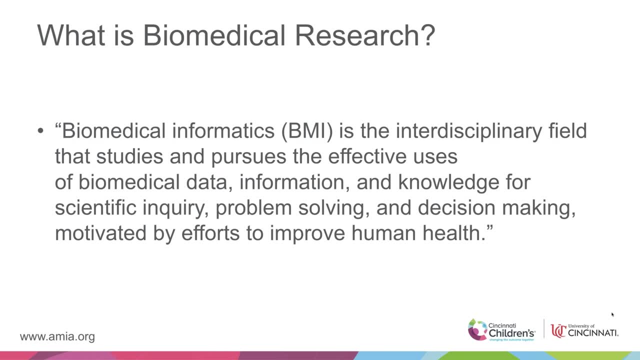 it's a medical field that practices the care of infants, children and adults, And then adolescents, And so then the big last term is really biomedical informatics research. So I took this definition from the American Medical Informatics Association's official definition of informatics. So biomedical informatics is the interdisciplinary field. 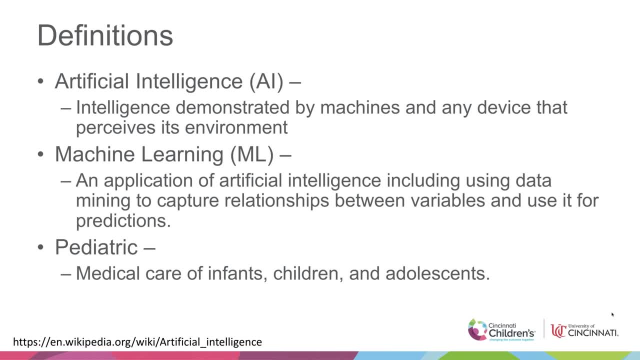 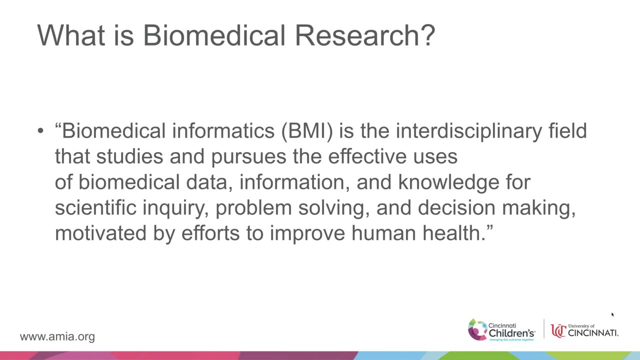 pediatrics, which could colloquially be described as everybody under the age of 18.. But really it's a medical field that practices the care of infants, children and adults. And then the big last term is really biomedical informatics research. So I took this definition from the 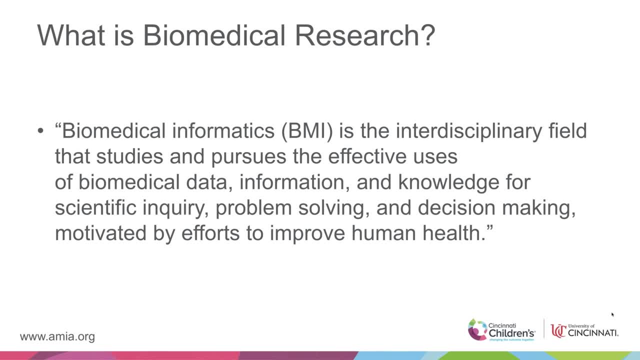 American Medical Informatics Association's official definition of informatics. So biomedical informatics is the interdisciplinary field that studies and pursues the effective uses of biomedical data, information and knowledge for scientific inquiry, problem solving and decision making. But what we're going to talk about quite a bit is the field that is really 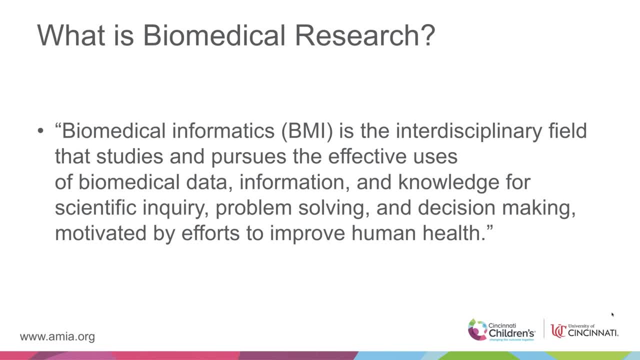 motivated by efforts to improve human health, but this isn't what you really say when you talk to people about informatics. so the first thing to know is that biomedical informatics research covers bioinformatics, clinical informatics, medical informatics, health informatics- pretty much everything you. 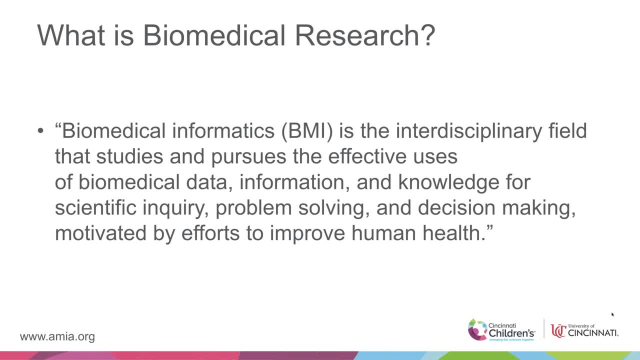 could put under this general umbrella. but I think the question really is like the: what do you answer at a party when someone asks what you do? and so, in the simplest terms, I say that I work with the hospital medical record system and health care providers to improve patient care and to help improve the use of the. 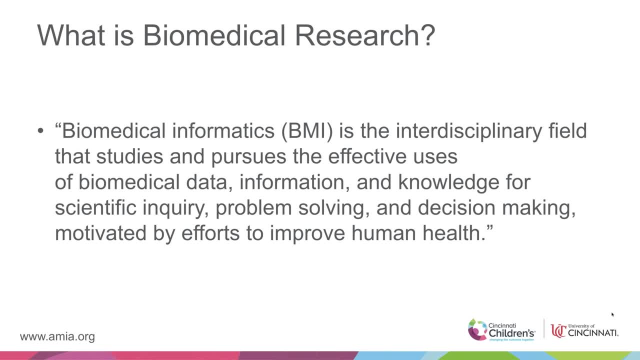 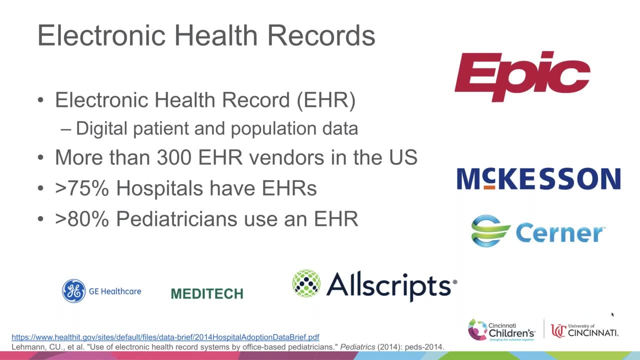 hospital medical record system. so which leads to the next most obvious question, which is: what's the hospital medical record system? well, that's an electronic health record, and that's okay, because then you can ask: what's an electronic health record? so the electronic health record is basically a digital. 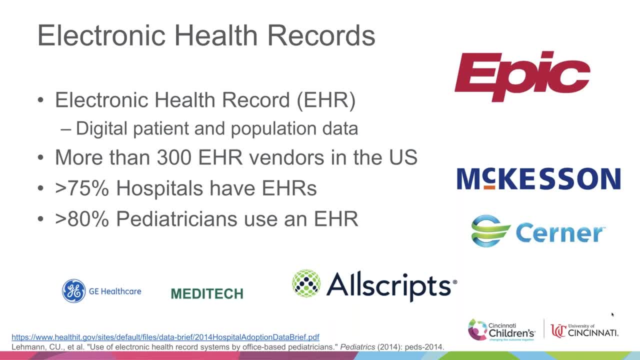 repository of information that you can use to monitor your patient's health, patient and population data. so on the large overview side, there are more than 300 EHR vendors in the United States. I've listed some of the main ones here: between Epic, McKesson, Cerner and Allscript. that covers about 80% of the 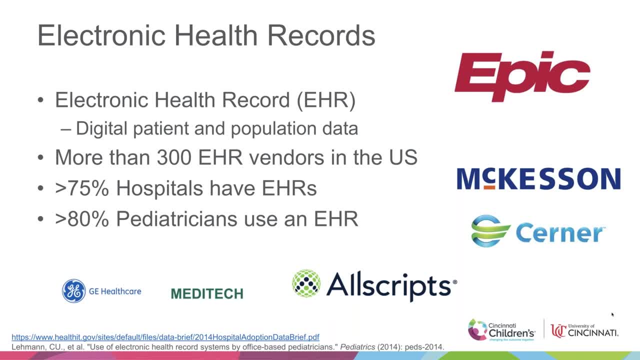 EHRs in the United States, and so they're very widespread. more than 75 percent of hospitals have an EHR in use and more than 80 percent of pediatricians report using an EHR, so that's a very broad and comprehensive overview of the health of hospital population and population data. so on the 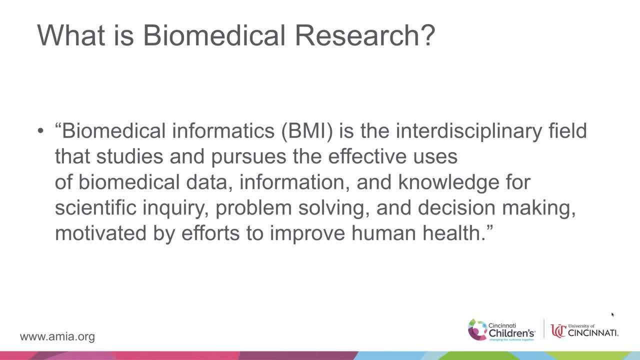 that studies and pursues the effective uses of biomedical data, information and knowledge for scientific inquiry, problem solving and decision making for the health and safety of children. And so it's a field that studies and pursues the effective uses of biomedical data, information and knowledge for scientific inquiry, problem solving and decision making. 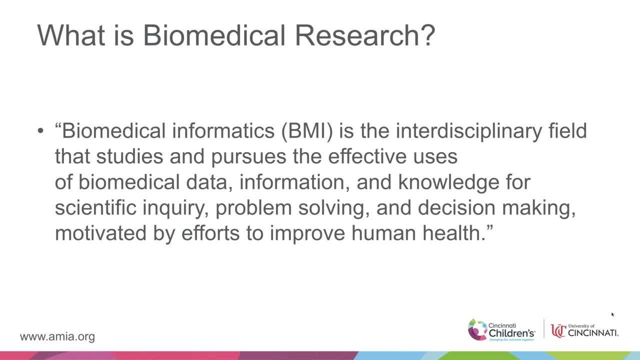 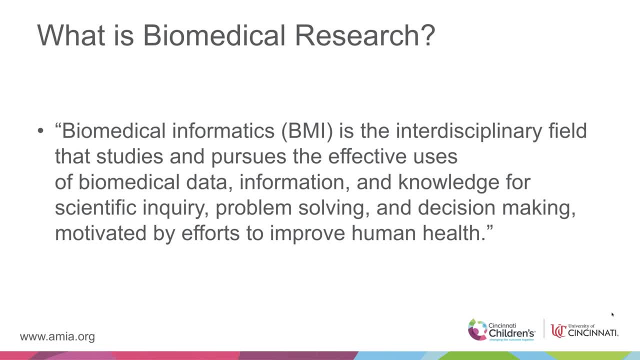 So the first thing to know is the biomedical informatics research covers bioinformatics, clinical informatics, medical informatics, health informatics, pretty much everything you could put under this general umbrella. But I think the question really is like the: what do you answer at a party when someone asks what you do? And so, in the simplest terms, 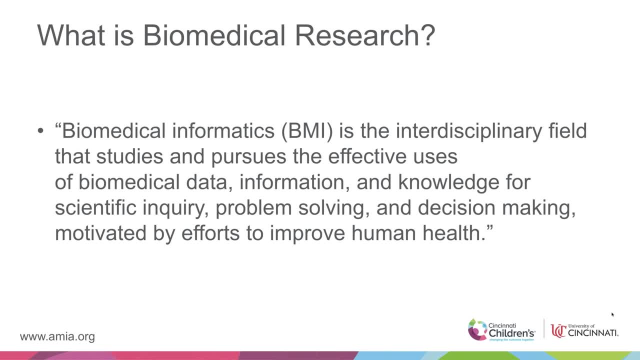 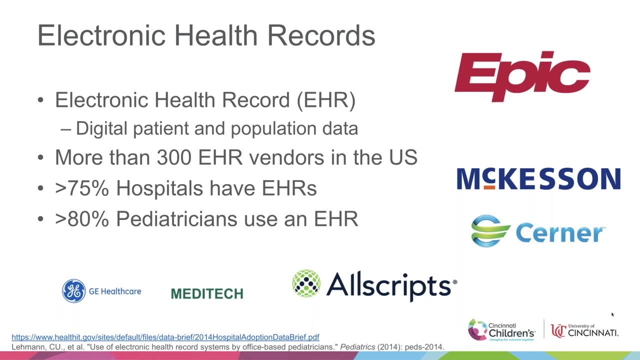 the hospital medical record system and healthcare providers to improve patient care and to help improve the use of the hospital medical record system. So which leads to the next most obvious question, which is: what's the hospital medical record system? Well, that's an electronic health record, and that's okay, because then you can ask: what's an electronic health record? 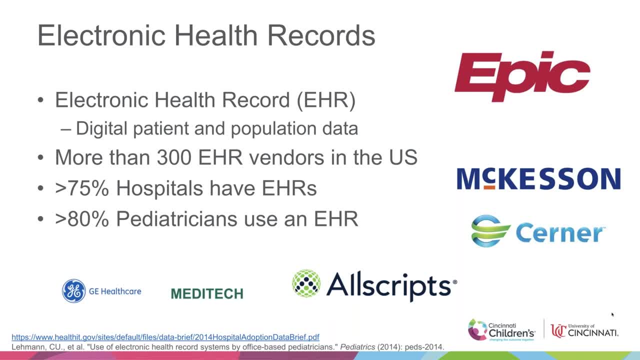 So the electronic health record is basically a digital repository of patient and population data. so on the large overview side, there are more than 300 EHR vendors in the United States. I've listed some of the main ones here. between Epic, McKesson, Cerner and Allscripts, that covers about 80 percent. 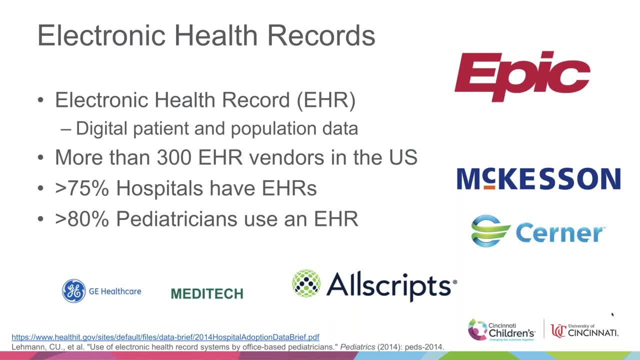 of the EHRs in the United States, and so they're very widespread. more than 75 percent of hospitals have an EHR in use, and more than 80 percent of pediatricians report using an EHR in their practice, and for us, it's our primary source of data for studies. 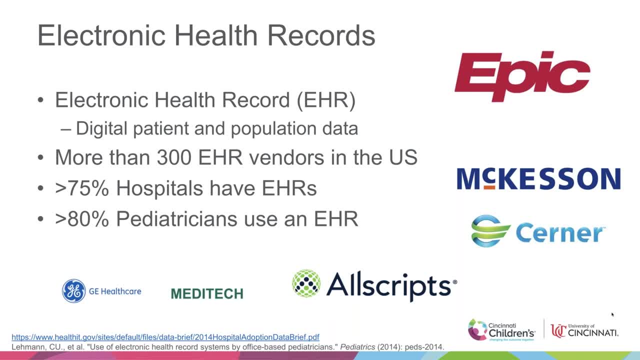 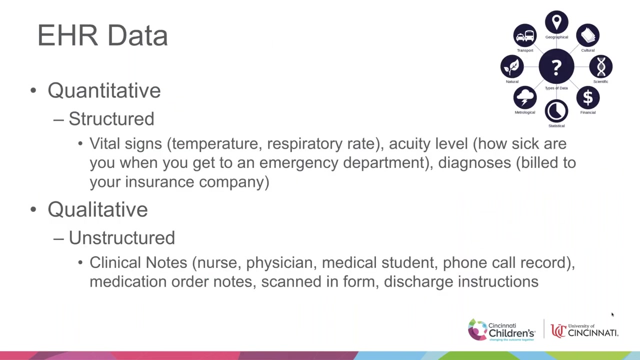 However, it was really designed for clinical care, documentation and billing purposes, and it is used for all those things, but it's also used for research and some of the administrative functions. And so what's in all of this information besides the? I looked at my own record. I saw how I did that day. I saw what I'm supposed to do after my visit. So there's two main 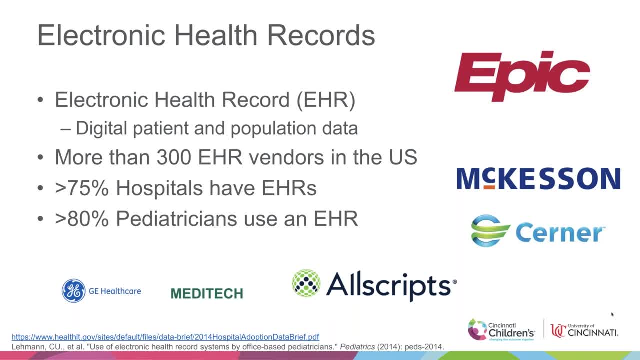 in their practice and for us, it's our primary source of data for studies. however, it was really designed for clinical care documentation and billing purposes, and it is used for all those things, but it's also used for research and some of the administrative functions, and so what's in all of this information? 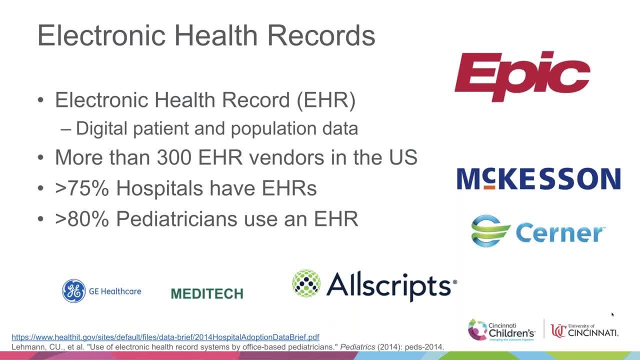 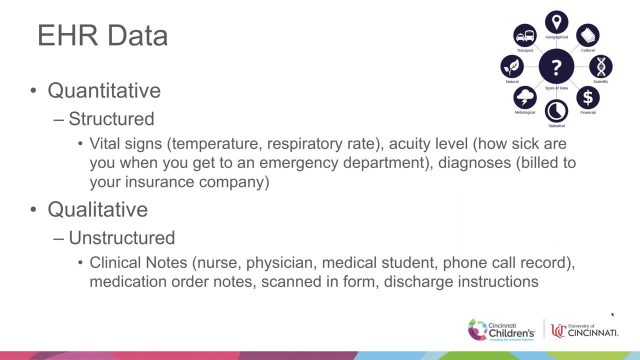 besides the, I looked at my own record. I saw how I did that day. I saw what I'm supposed to do after my visit. so there's two main types of data in the EHR and the first one of those is quantitative data and these are structured data, so things like vital signs. so when you go in and you have 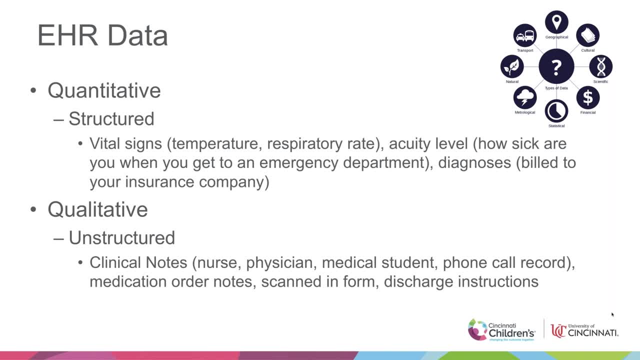 your temperature taken and your blood pressure to take in. these are stored in your EHR. these are structured. another is your acuity level. so when you visit an emergency department you typically get a score of one to five about basically how sick you are when you walk through the door. 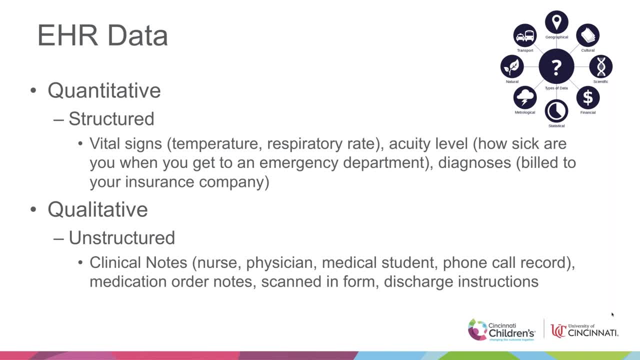 one being the sickest, five being the less sick, least sick, and then, finally, another example of structured data are your billing diagnoses. so why was it you were really there that day? what was billed to your insurance company at the end of the day? the other piece of data in the EHR, which is what I primarily 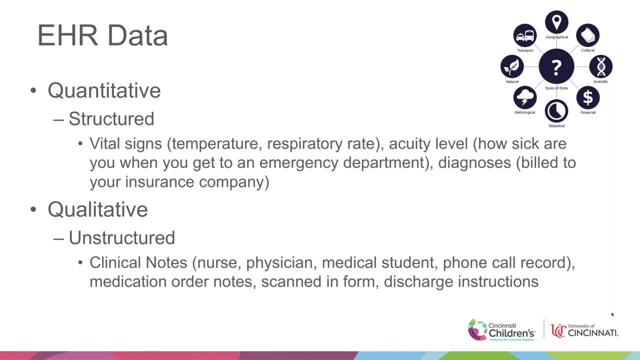 work with, with machine learning, is the qualitative data and it's your unstructured data, and there's a lot of this. it represents- which I'll actually tell you two or three times- about 80% of the data in the EHR and the first set of 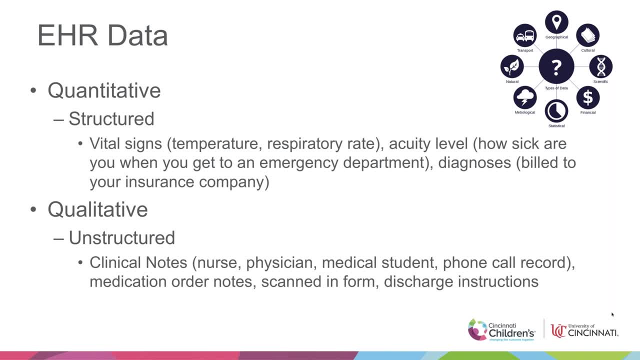 these are your clinical notes. so anytime someone talks to you when you visit the hospital, they write a note to document what they did. so when your nurse comes in your room to check on you, he or she goes back and writes a note and documents what they did and why. at the end of your visit, your physician or your 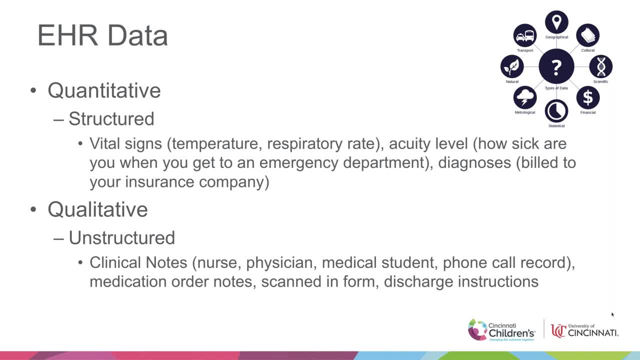 provider writes a note saying: this is what we talked about today. this is what we recommended. here are the things that you can do to make sure that you're not going to miss out on any of the data that you're going to be receiving in the next few days. so here are some of the structured data, but this is how my 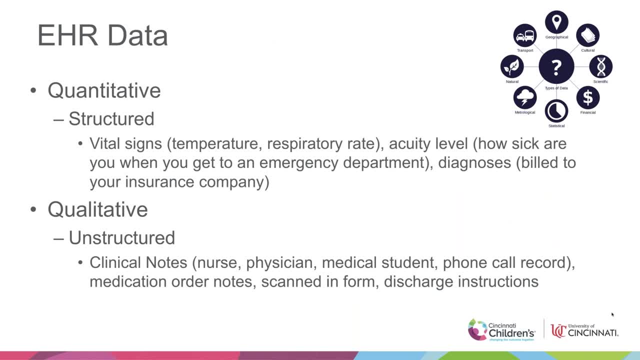 types of data in the EHR, and the first one of those is quantitative data and these are structured data, So things like vital signs. so when you go in and you have your temperature taken and your blood pressure taken, these are stored in your EHR. These are structured. Another is your acuity level. 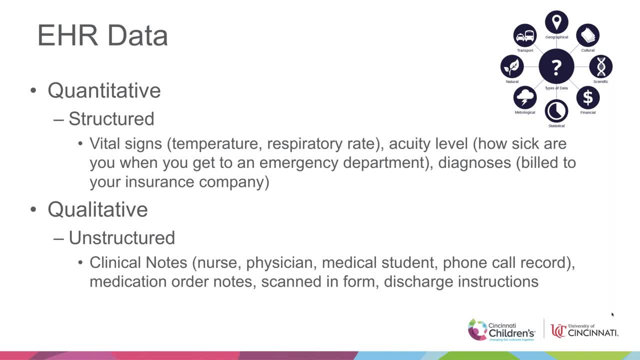 so when you visit an emergency department, you typically get a score of one to five about basically how sick you are when you walk through the door, one being the sickest, five being the less sick. And then, finally, another example of structured data are your billing diagnoses. So why wasn't? 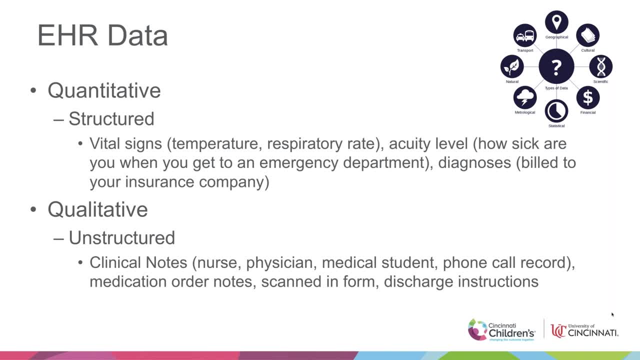 you were really there that day, What was billed to your insurance company at the end of the day? The other piece of data in the EHR, which is what I primarily work with with machine learning, is the qualitative data, and it's your unstructured data, and there's a lot of this. It represents. 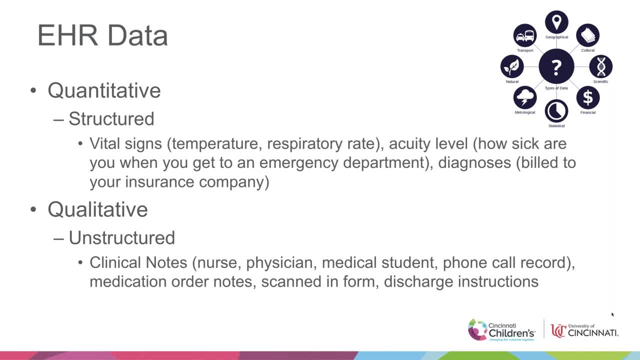 which I'll actually tell you two or three times. about eighty percent of the data is structured. The first set of these are your clinical notes. So anytime someone talks to you when you visit the hospital, they write a note to document what they did. So when your nurse comes in your room to check, 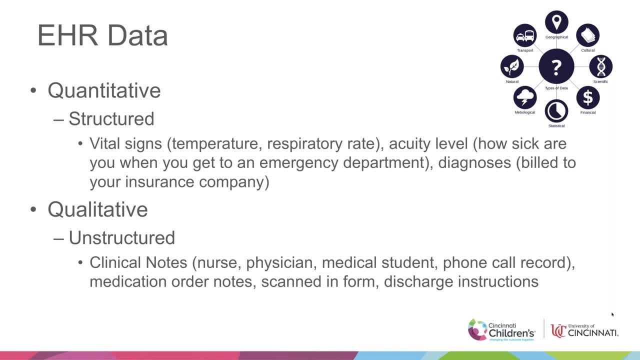 on you. he or she goes back and writes a note and documents what they did and why. At the end of your visit, your physician or your provider writes a note saying this is what we talked about today. this is what we recommended. here are some of the structured data, but this is how my patient's doing. 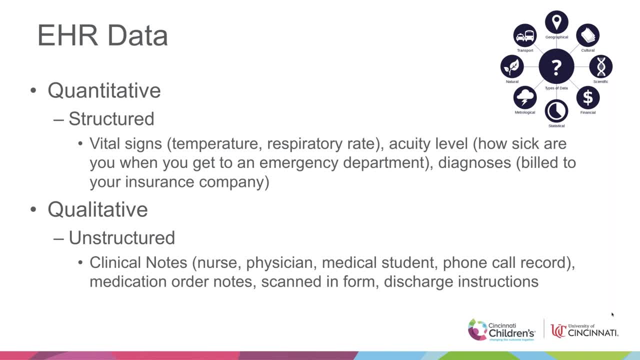 and this is how I'm going to do it. So the other piece of data is the clinical notes. So the clinical notes are the logical next steps. If you call the hospital, you get yet another one of these recorded and free text sheets of information. So then it's not just clinical notes that way, but also if you have a medication order for any medication and your provider types in extra information about it. there's another piece of unstructured data If you have a pdf form scanned in from a prior hospital visit. there's some more unstructured data and those discharge instructions where they provide you with a PDF form and a PDF document. 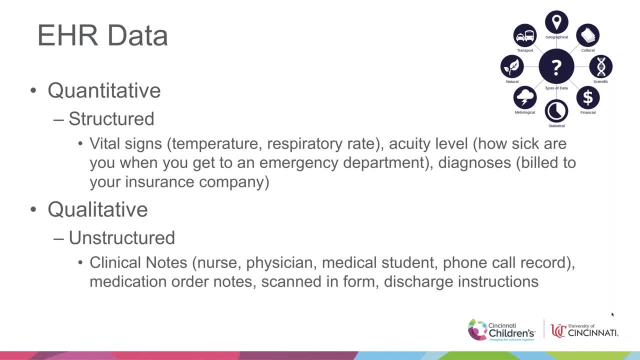 So what we see here is that if you are going to take a pdf form and you are trying to get your medical records or you have a pdf form of this, you have to take a pdf form and you have to take a pdf form of this, Then you need to get a pdf form in your medical record. So that's a pdf form that you can provide. and they say: please take these medications, please follow up with the following people. All of these are actually free text when they're stored in your medical record. 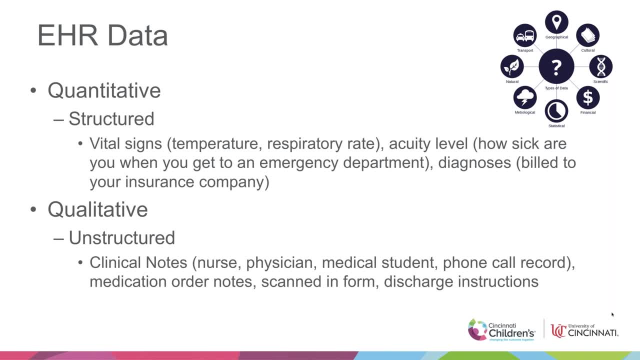 patient's doing. and here are the logical next steps. if you call the hospital, you get yet another one of these recorded and free text sheets of information. so then it's not just clinical notes that way, but also if you have a medication order for any medication and your provider types in extra information. 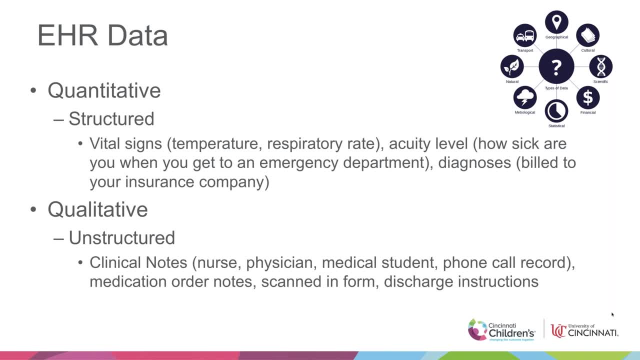 about it. there's another piece of unstructured data- if you have a PDF form scanned in from a prior hospital visit. there's some more unstructured data and those discharge instructions where they provide and they say: please take these medications, please follow up with the following people. all of these are: 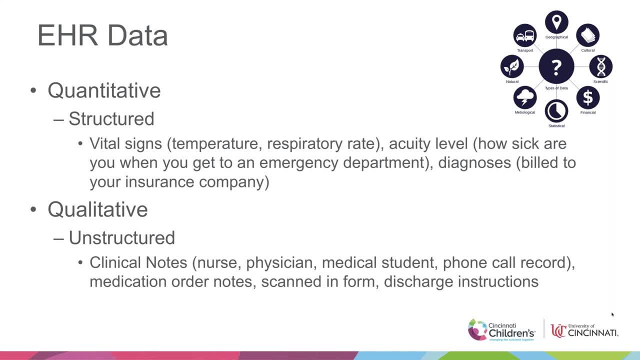 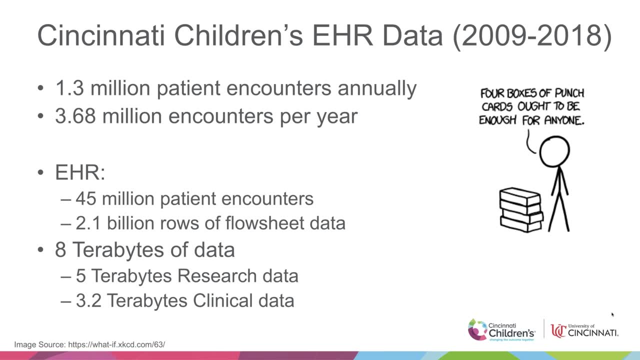 actually free text when they're stored in your medical record. so how much data is it really? we are one institution and we are a pediatric institution. we have on average about 1.3 million patient encounters. we have about three point 68 million encounters per year. so the 1.3 are distinct patients And in our electronic 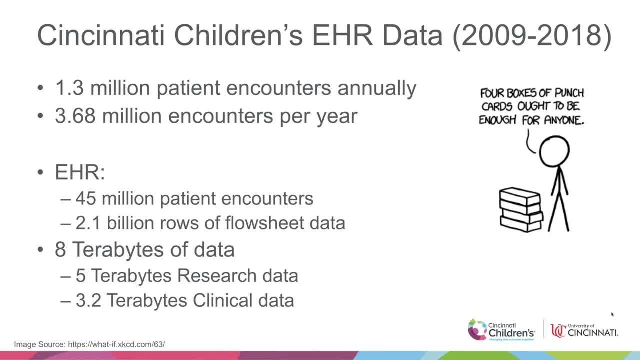 health record. we have a total of about 45 million patient encounters listed. Of those, we have 2.1 billion rows of flow sheet data And our EHR. these data are from 2009 to 2018.. Flow sheet data are typically your structured data And these are all stored in the EHR. 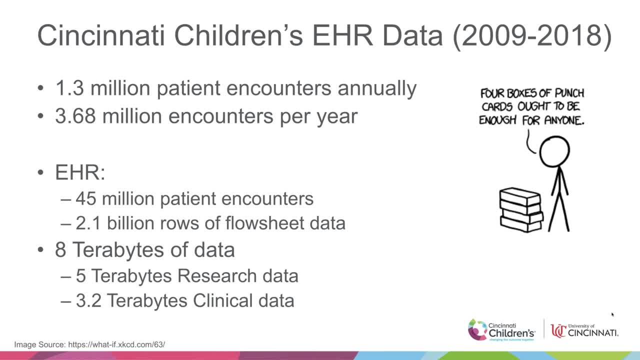 In total, we have eight terabytes of data being stored. 3.2 terabytes of those are for clinical data only and represent clinical care and things that are happening, And the other five terabytes of data are research-based and they represent studies. they represent 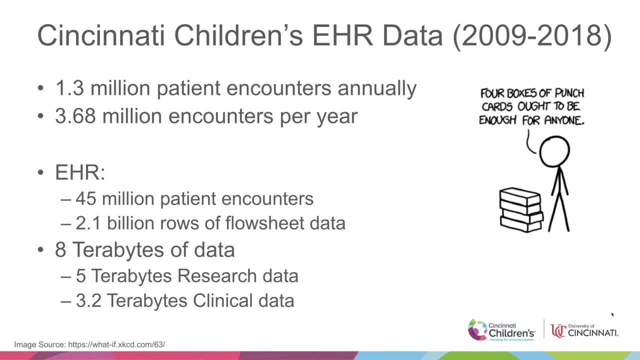 research that is across different institutions, but they are all things we are storing, we are maintaining and that we are able to access. What's important to note here is that we are only one hospital and we serve the greater Cincinnati area, but this is only one hospital. 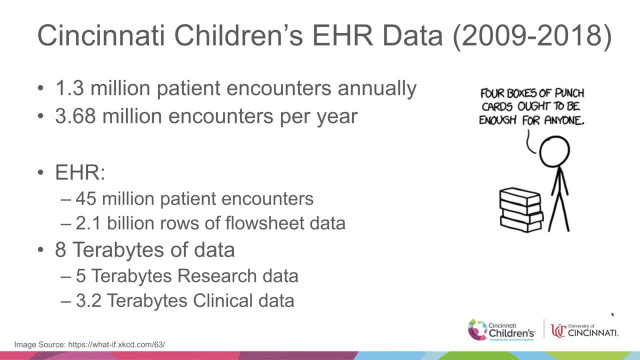 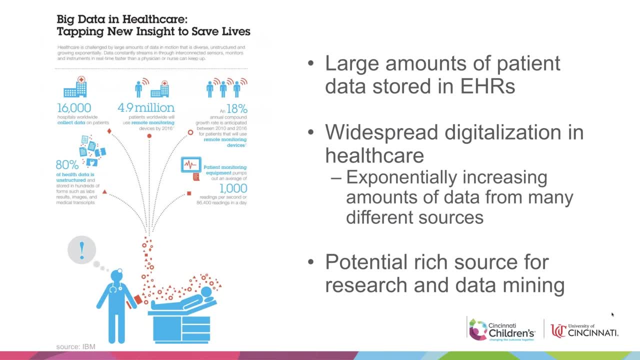 one state and there are several other children's hospitals in our state. So the take-home message from the last couple of slides is that there's a lot of data out there in the world, So there's large amounts of patient data stored in an EHR And with 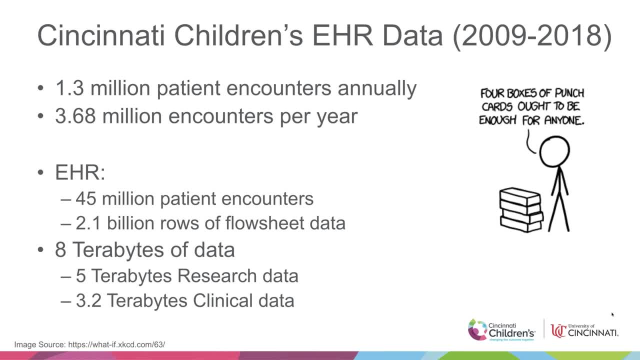 So how much data is it really? We are one institution and we are a pediatric institution. We have, on average, about 1.3 million patient encounters. We have about 3.68 million encounters per year, So the 1.3 are. 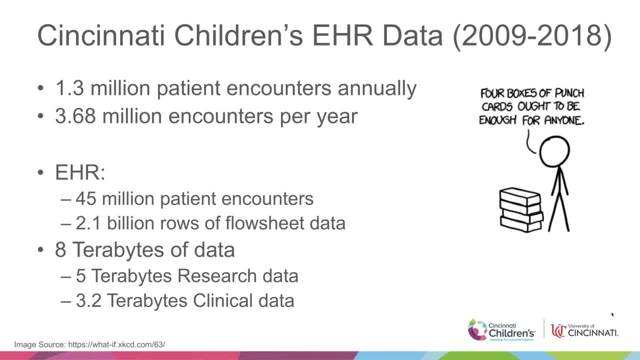 distinct patients and in our electronic health record we have a total of about 45 million patient encounters listed. of those, we have 2.1 billion rows of flow sheet data and our EHR. these data are from 2009 to 2018. flow sheet data are: 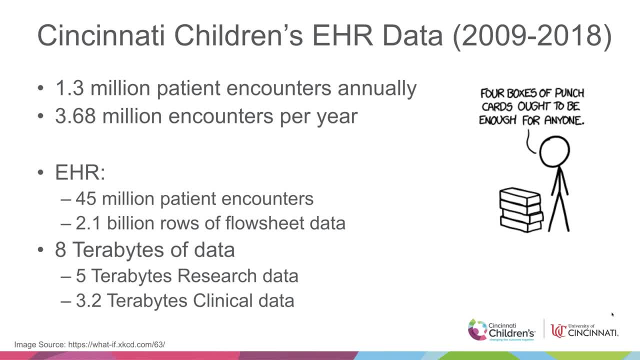 typically your structured data, and these are all stored in the EHR. and total we have 8 terabytes of data being stored. 3.2 terabytes of those are for clinical data only and represent clinical care and things that are happening, and the other 5 terabytes of data are research based and they represent studies. they 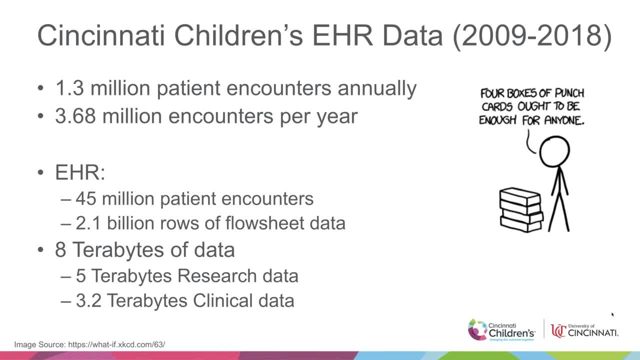 represent research that is across different institutions, but they are all things we are storing, we are maintaining and that we are able to access. what's important to note here is that we are only one one one a hospital, and we serve the greater Cincinnati area, but this is only one. 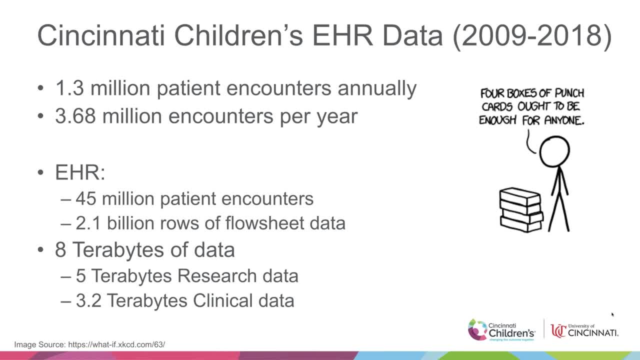 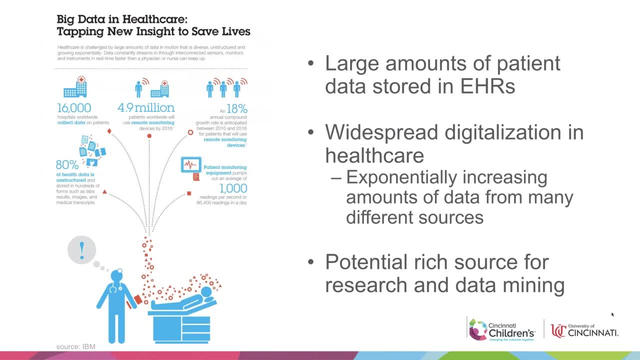 hospital one state and there are several other children's hospitals in our state. so the take-home message from the last couple of slides is that there's a lot of data out there in the world. so there's large amounts of patient data stored in an EHR and, with the rat, widespread digitalization of health care. 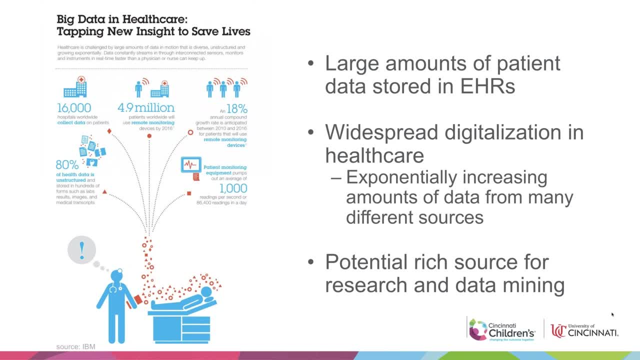 we actually have an exponentially increasing amounts of data from a bunch of different sources, and it's a potentially rich source for research and data mining. an important thing to remember that I've already brought up once before here: on the left hand side, 80% of health data is. 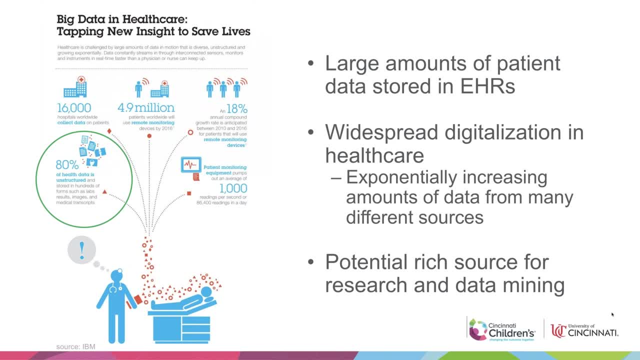 unstructured and that's stored in those clinical notes and while you can sit and read all the information. that's a lot of data. so why aren't we already doing a lot of big data projects with all of these data and why aren't we already analyzing all these data and changing patient care and making the world a 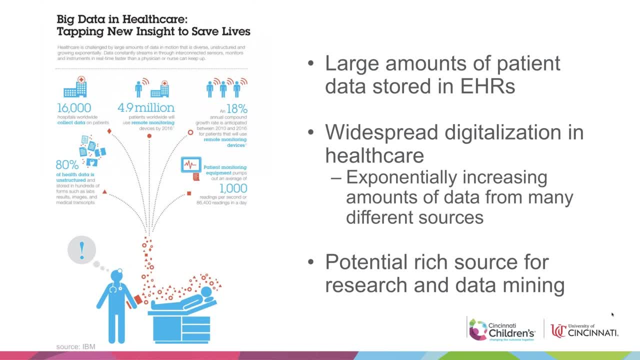 the widespread digitalization of healthcare. we actually have an exponentially growing amount of data from a bunch of different sources, And it's a potentially rich source for research and data mining- An important thing to remember that I've already brought up once before here. on the left-hand side, 80% of health data is unstructured And that's. 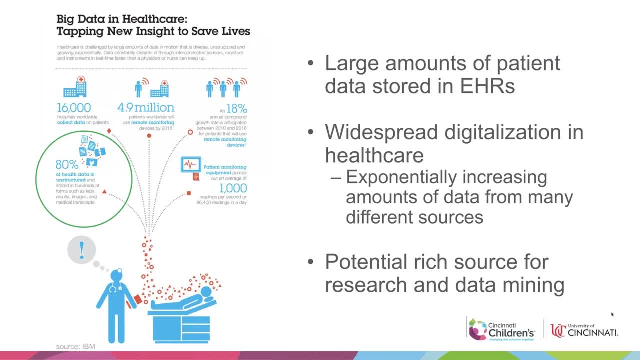 stored in those clinical notes And while you can sit and read all the information. that's a lot of data, So why aren't we already in the EHR? So we are already in the EHR, So why aren't we? 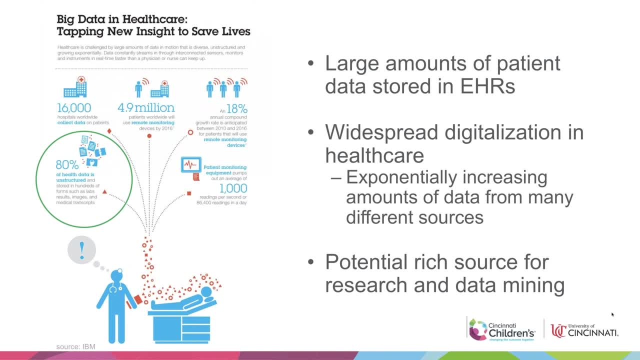 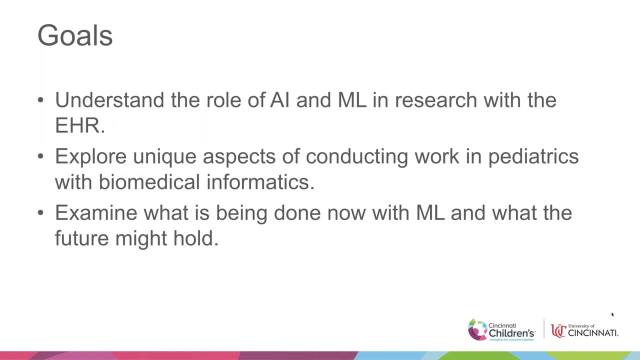 doing a lot of big data projects with all of these data, And why aren't we already analyzing all these data and changing patient care and making the world a better place? Well, the short answer is that we are. We're just doing it piecemeal as we go through things. So the 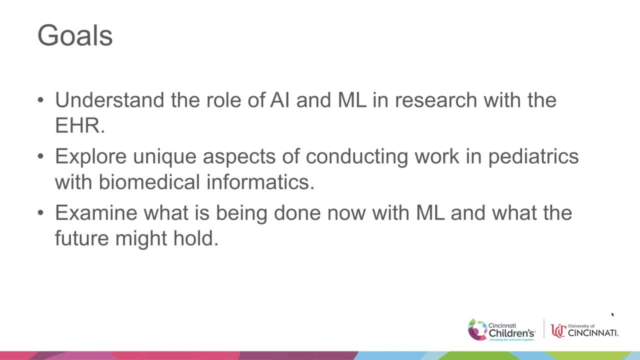 goals, kind of is. the overarching for the rest of the talk is to understand the role of artificial intelligence and machine learning in research with the EHR, to explore some of the unique aspects of conducting research and work in pediatrics with biomedical informatics. and 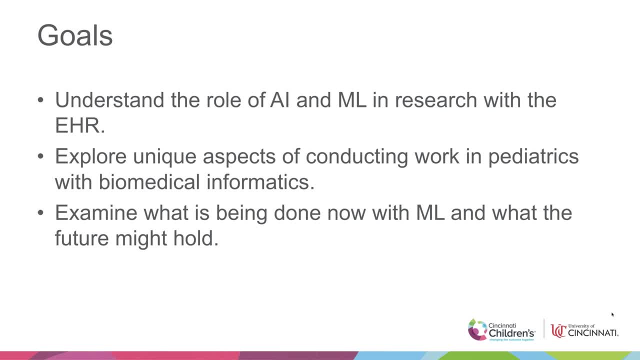 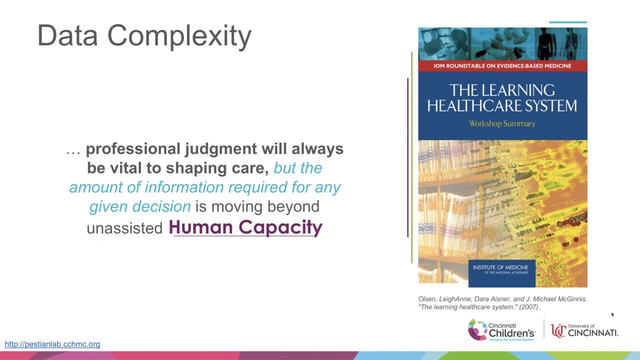 then to examine what's being done now with machine learning and what might the future hold for everything. So why do we do this? And the important thing about this is the data complexity. We've talked about how much data there are, and they're all there. they're. 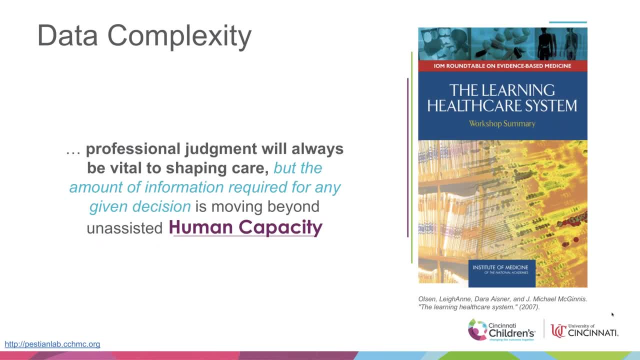 all available, but we need to make use of all of them. So, with those 80% of unstructured data, they contain rich and valuable information for everything, But the amount of information required for a given decision is just too much for one human to take care of, And that's where the computers come in. We can help people. 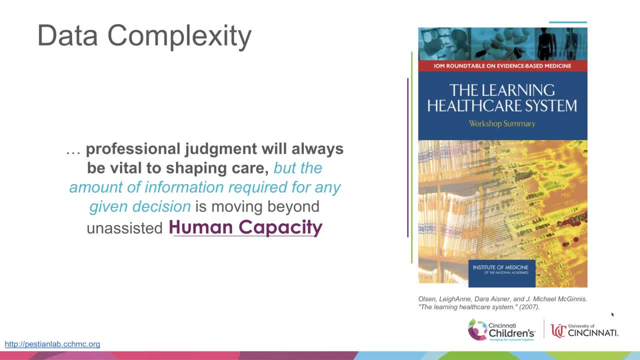 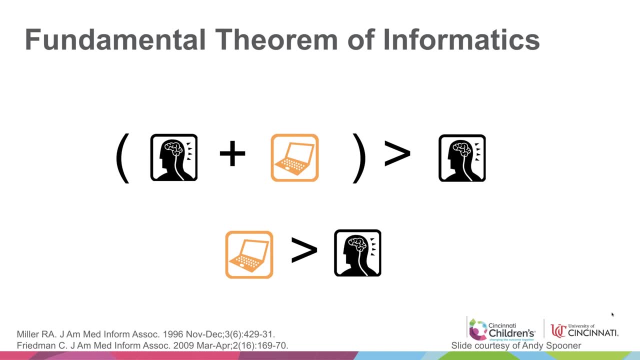 make better decisions with more information, with the idea of improving care. So I want to go ahead and present to you what's the fundamental theorem of informatics. The goal of informatics is that the human And the computer is going to perform better than the human alone. The fundamental theorem. 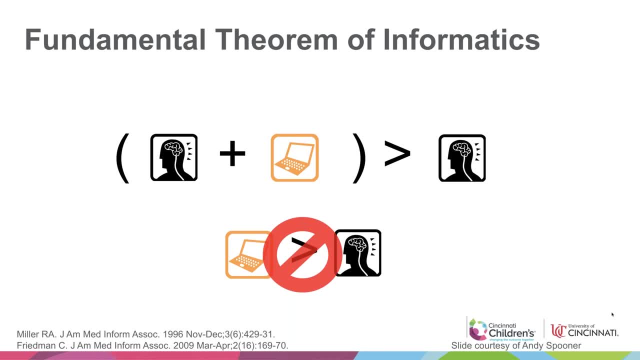 of informatics is not that the computer is going to perform better than the human, but that we can aid someone and we can help them make a better decision. So what we want to do is help the users make a more informed decision and basically, ultimately improve. 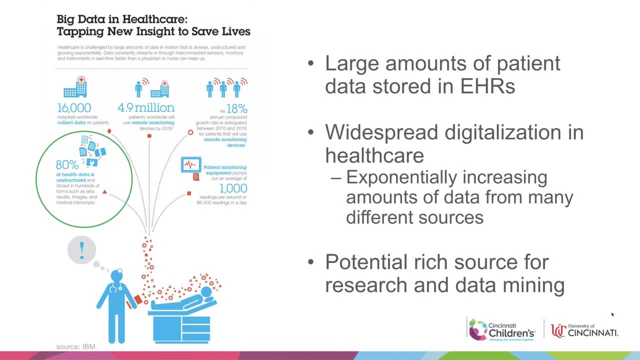 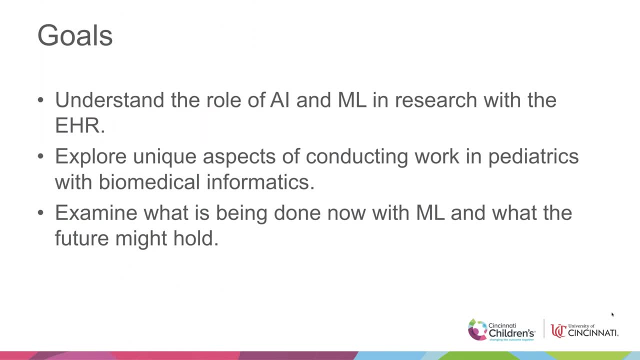 better place? well, the short answer is that we are. we're just doing it piecemeal as we go through things. so the goals- kind of is the overarching for the rest of the talk- is to understand the role of artificial intelligence and machine learning in research, with the EHR to explore some of the unique aspects. 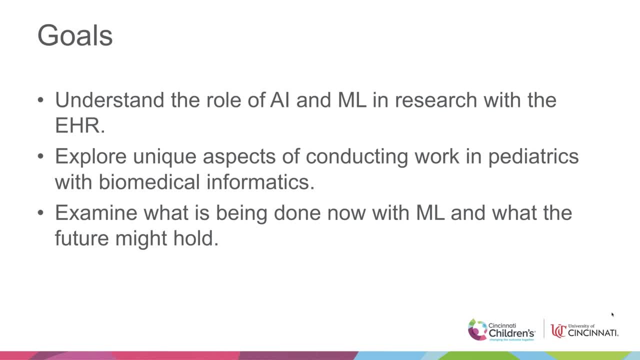 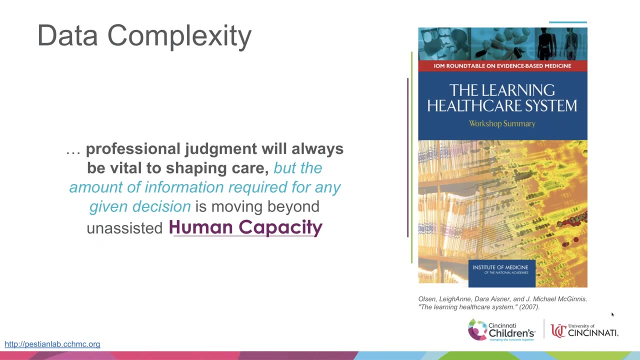 of conducting research and work in pediatrics with biomedical informatics, and then to examine what's being done now with machine learning and what might the future hold for everything. so why do we do this? and the important thing about this is the data complexity. we've talked about how much data there are and 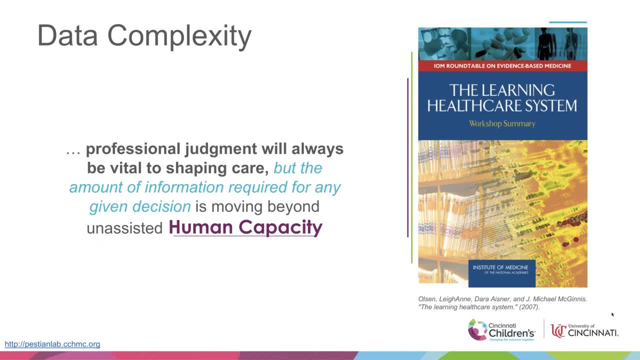 they're all there, they're all available, but we need to make use of all of them. so, with those 80% of unstructured data, they contain rich and valuable information for everything, but the amount of information required for a given decision is just too much for one human to take care of, and that's where the computers come in. we can help. 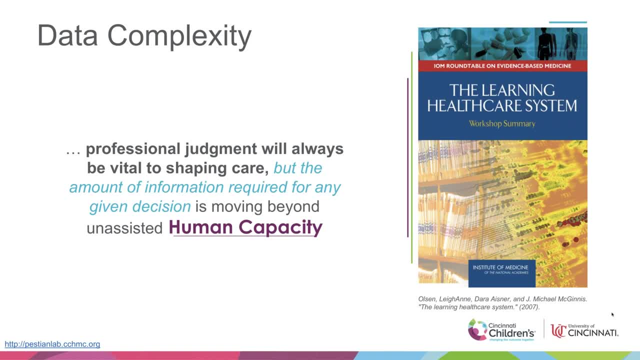 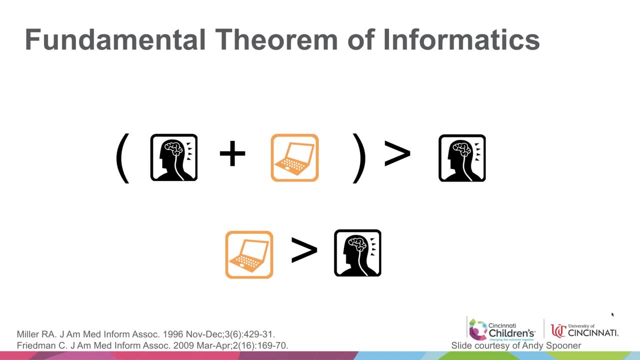 people make better decisions with more information, with the idea of improving care. so I want to go ahead and present to you what's the fundamental theorem of informatics. the goal of informatics is that the human and the computer is going to perform better than the human alone. the fundamental theorem of 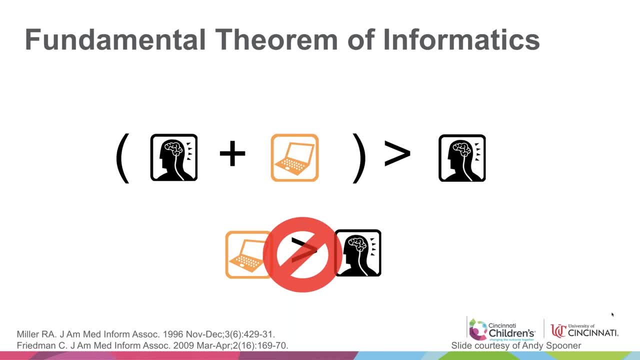 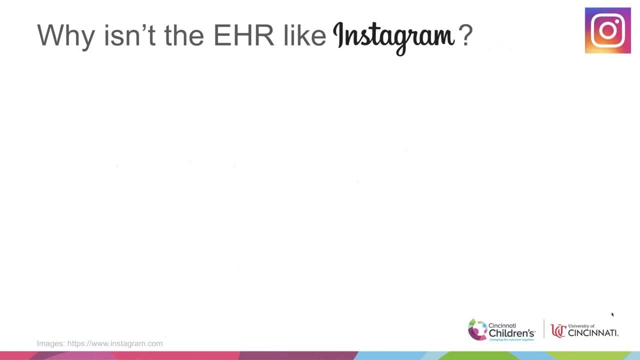 informatics is not that the computer is going to perform better than the human, but that we can aid someone and we can help them make a better decision. so what we want to do is help the users make a more informed decision and basically ultimately improve patient outcomes. so but you say I have an EHR or I use a. 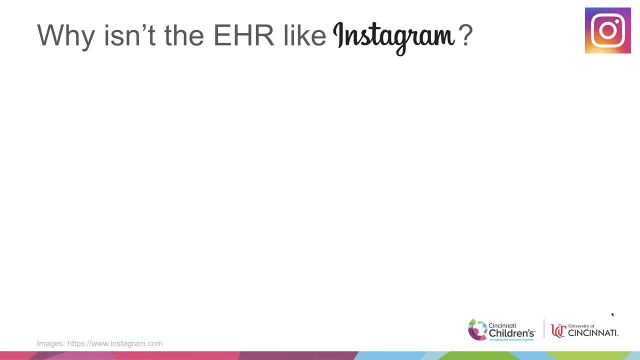 word processing program or I use email and it's actually not that easy to use. it's not user-friendly. you suffer from alert fatigue in both your EHR and your phone. you get text messages, you get reminders. you get everything under the Sun, like you. just you really want research to be great. you want everything to be happy, but you. 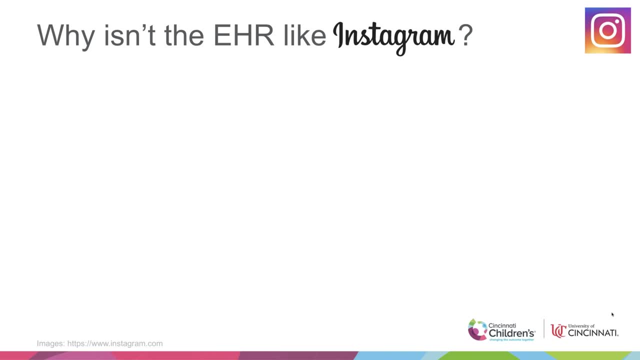 also want it to be really easy, simple to use and do exactly what you want, exactly like what happens when you want to upload a new picture to Instagram. so why isn't the EHR example? it's not exactly like Instagram right now. luckily, I have a comparison for you. 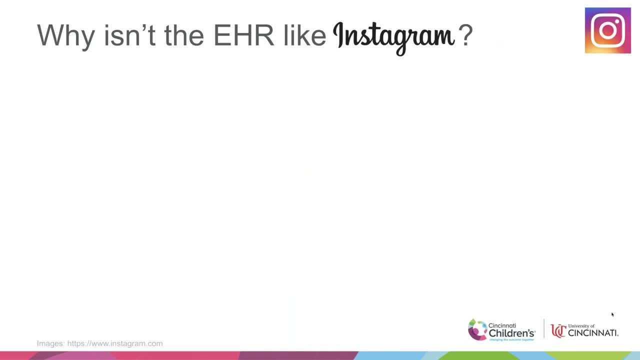 patient outcomes. So? but you say: I have an EHR or I use a wordpress, I use email And it's actually not that easy to use. It's not user friendly. You suffer from alert fatigue in both your EHR and your phone. You get text messages, You get reminders. 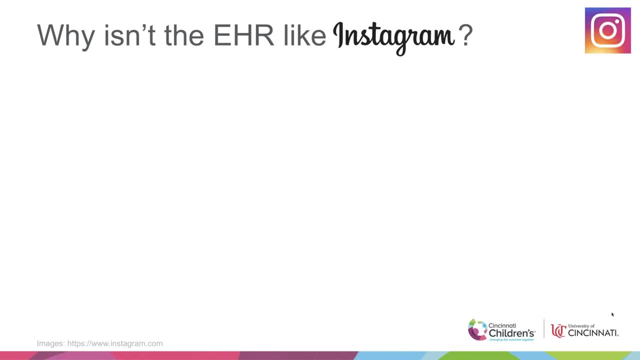 You get everything under the sun, Like you just. you really want research to be great. You want everything to be happy, But you also want it to be really easy, simple to use and do exactly what you want. Exactly, Exactly, Exactly. like what happens when you want to upload a new picture to Instagram. 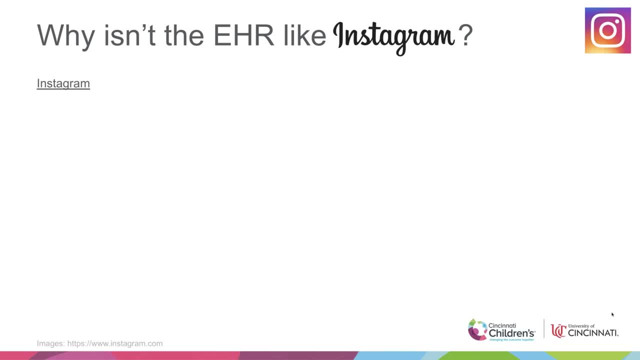 So why isn't the EHR exactly like Instagram right now? Luckily, I have a comparison for you. So here on Instagram, there's really only one type of user, And that's fine. So you, you have your own account, You can do everything you want to. 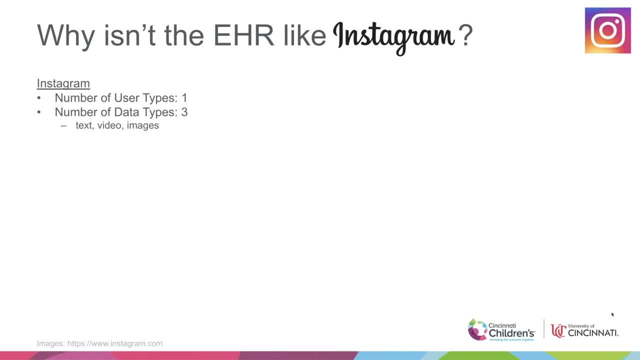 do with it. You have a couple of different types of data. You can have text data, You can have video, You can have images. You're control in control of all of your own data. here You have a lot of features. You can upload a photo, You can 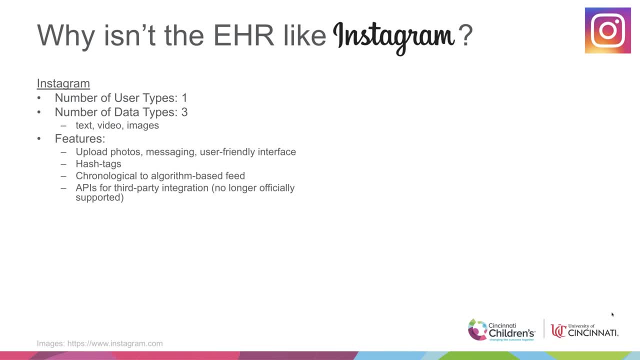 message someone. You have a nice, clean, user friendly interface. You can add hashtags so that it's easier to search things in the future, And you have both a chronological or an algorithmic based feed, depending on what Instagram is doing today, so that you can kind of see what's. 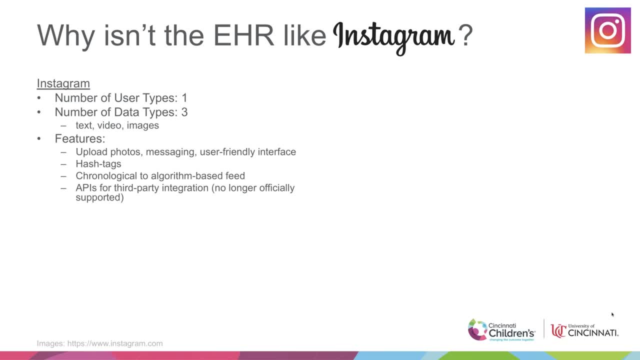 happened with you and your friends, etc. And then APIs, which are application programming interfaces, exist for 30 days, And then you have third party integration. So they they do technically exist, But the idea is, if you said I don't like the way, 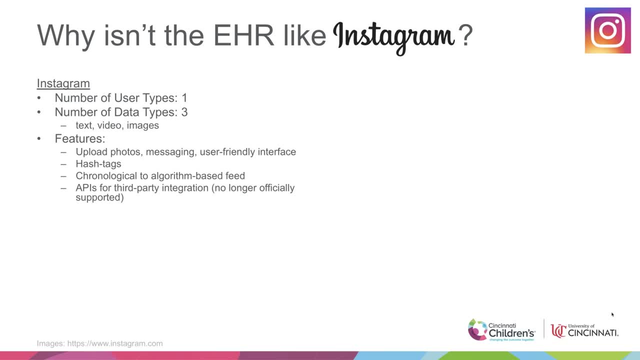 Instagram shows me these things. I want to use this other program to get out the same data. You can do that, And so you control your own data. You have privacy. You can choose what's posted to your account. You can ask for an image to be removed. You can do something if someone else tags. 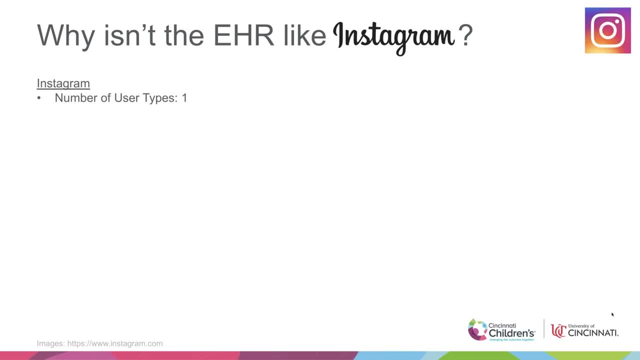 so here on Instagram, there's really only one type of user and that's fine. so you, you have your own account. you can do everything you want to do with it. you have a couple of different types of data. you can have text data, you can have video, you can have images. you're control, in control of all of your own data here. 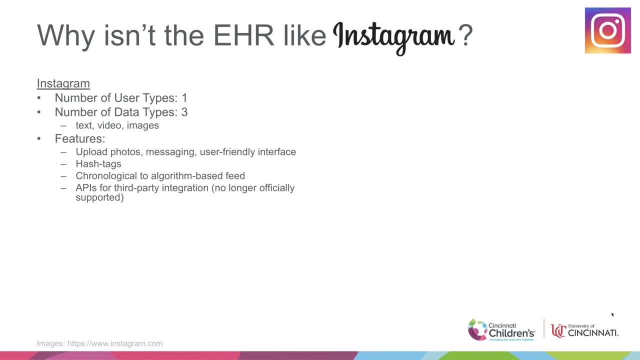 you have a lot of features: you can upload a photo, you can message someone, you can send a text message. you can send a text message. you can send a text message. you have a nice, clean, user-friendly interface. you can add hashtags so that it's easier to search things in the future, and you have both a 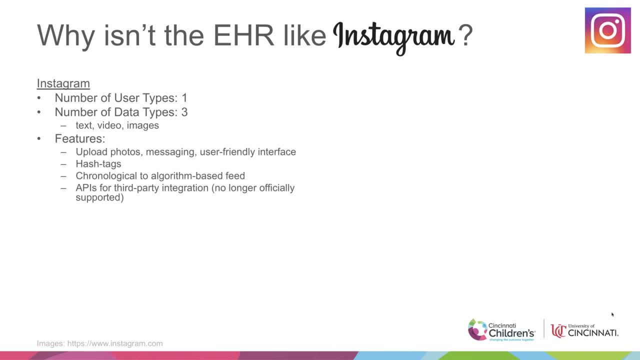 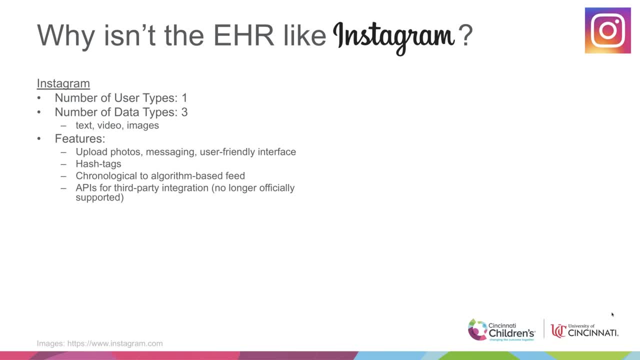 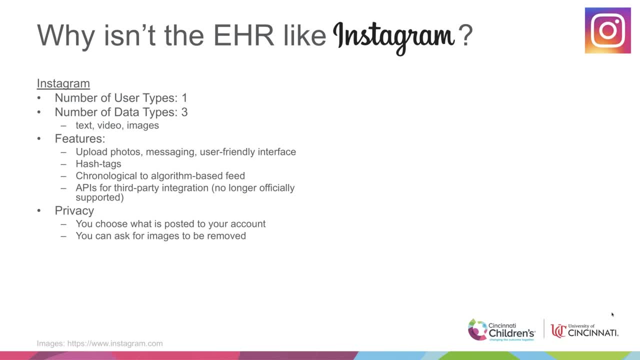 privacy. you can choose what's posted to your account. you can ask for an image to be removed. you can do something if someone else tags you in an image you don't want to be in anymore. this is great. Instagram is wonderful. it's easy to use. so how is the EHR are different, so first let's do the number of. 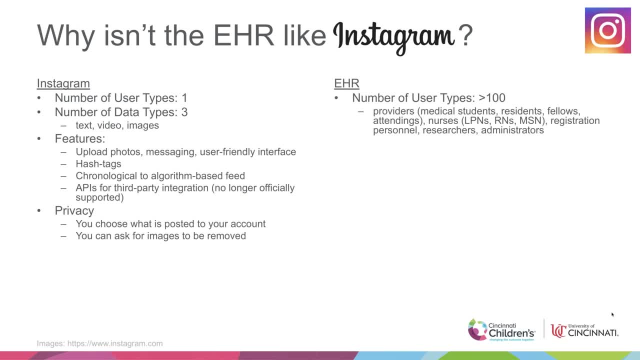 different user types. So there's, conservatively, more than 100 different types of user in the EHR As far as providers alone. you have medical students, you have residents, you have fellows, you have attendings, and then you have different types of provider for different areas, And they 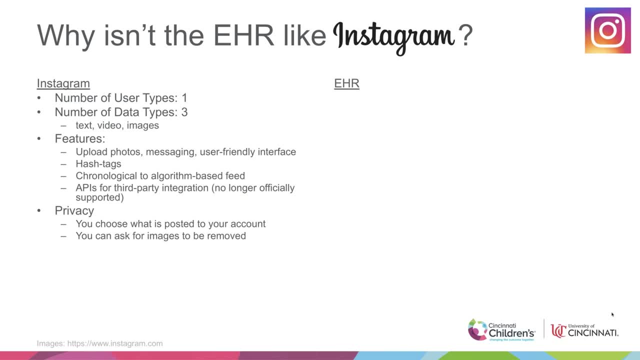 you in an image you don't want to be in anymore. This is great. Instagram is wonderful. it's easy to use. So how is the EHR different? So first let's do the number of different user types. So there's conservatively. 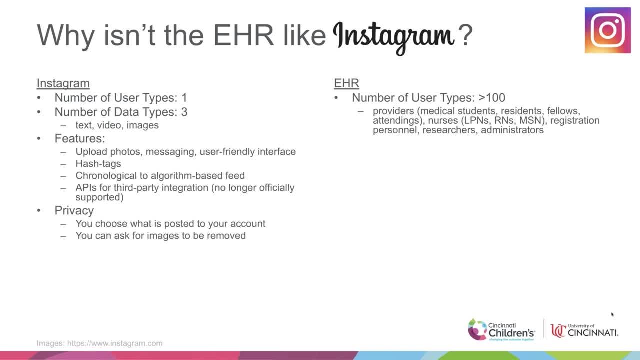 more than a hundred different types of user in the EHR as far as providers alone. You have medical students, you have residents, you have fellows, you have attendings, and then you have different types of providers for different areas, and they each have their. 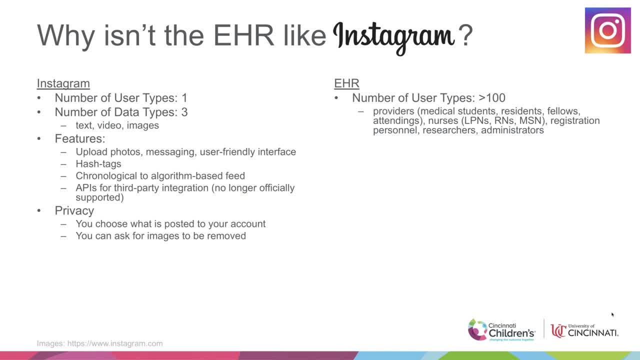 own, different view to aid in their workflow. Then you have nurses, and nurses each have their own type of providers as well. with the same idea, You only want some people to be able to write orders. For example, I want my provider to be able to write a medication. 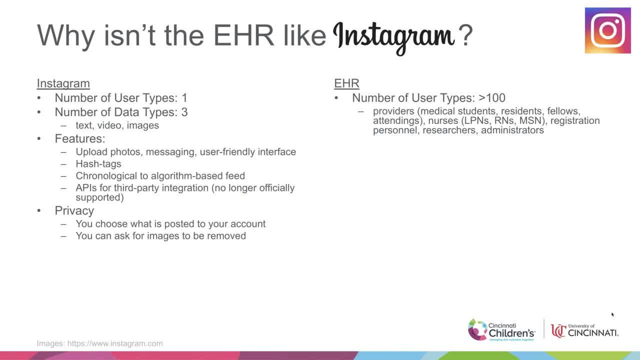 order for me, but I don't really want researchers or administrators to be able to write a medication order for me, So those have to be taken care of. And so what about the data that are stored in the EHR? I also went a little over conservative here and said there were at least 20 types. 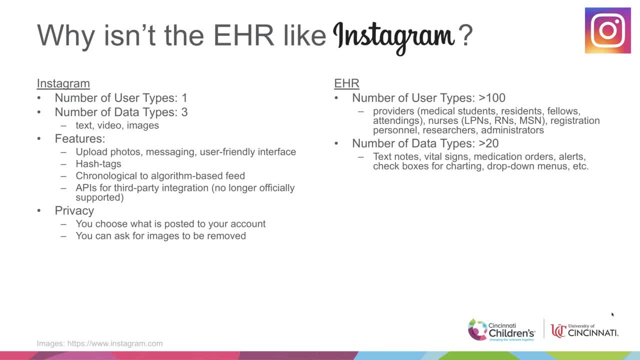 of data in the EHR. There are in fact more, But just on the baseline. you could have a text-based note, You could have those structured data that are vital signs. You could have your medication orders. You could have the check boxes that are just there for charting. 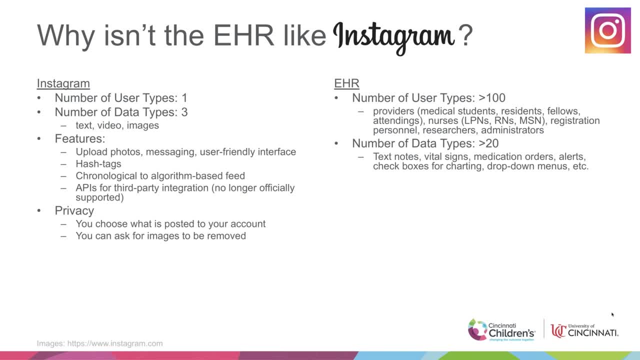 to make sure things got done. You could have drop-down menu selections, You could have images, You could have PDFs, You could have all sorts of things being stored. So these are a lot of things and nothing is insurmountable. 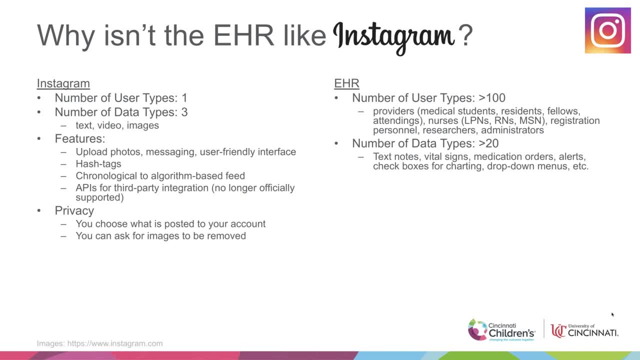 So now we've still got a lot going on right here to not make it quite as easy to use. But what about the number of features that are included in your EHR, As I kind of alluded to earlier? you can have notes, You can have orders, You can have your. 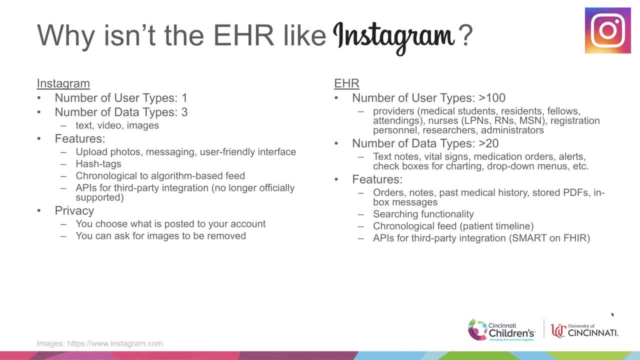 past medical history. You can have an in-basket message where your providers message each other about your care, Or reminders could be sent to your provider about you and about your care, about what needs to be done in the future, just to help them out. 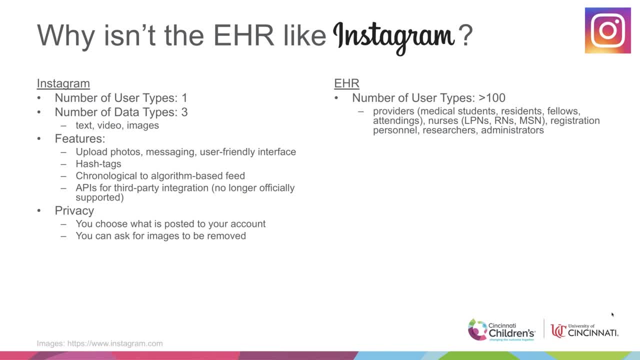 each have their own different view to help aid in their workflow. Then you have nurses, and nurses each have their own type of providers as well. with the same idea, You only want some people to be able to write orders. For example, I want my provider to be able to write a medication order. 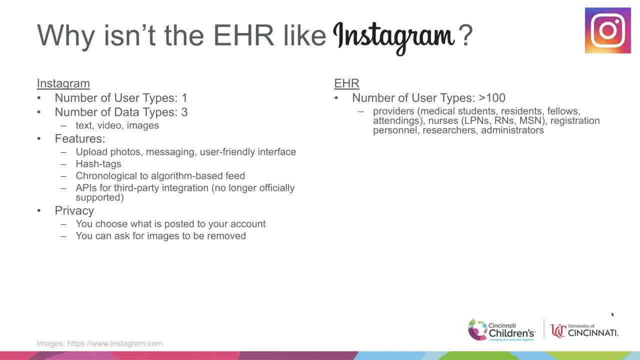 for me, but I don't really want researchers or administrators to be able to write a medication order for me, So those have to be taken care of. And so what about the data that are stored in the EHR? I also went a little over conservative here and said there were at least 20 types of data in 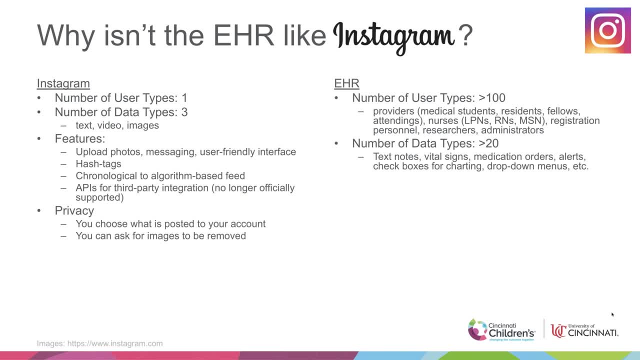 the EHR. There are in fact more, But just on the baseline. you could have a text-based note. You could have those structured data that are vital signs. You could have your medication orders. You could have the check boxes that are just there for charting to make sure. 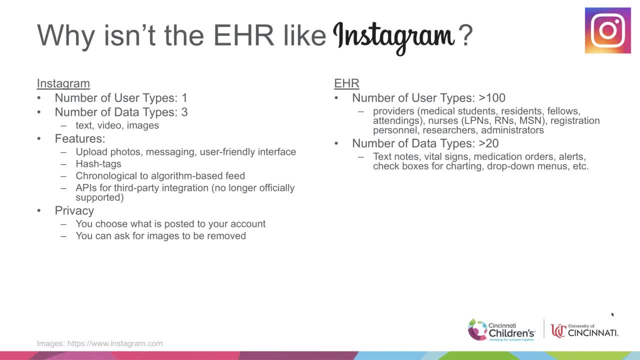 things got done. You could have drop-down menu selections, You could have images, You could have PDFs, You could have all sorts of things being stored. So these are a lot of things and nothing is insurmountable. So now we've still got a lot going on right here. to not make it quite as easy, 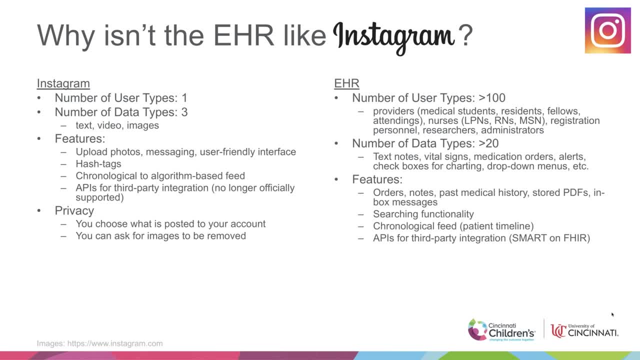 to use, But what about the number of features that are included? So the number of features that are included in your EHR, As I kind of alluded to earlier. you can have notes, You can have orders, You can have your past medical history, You can have an in-basket message. 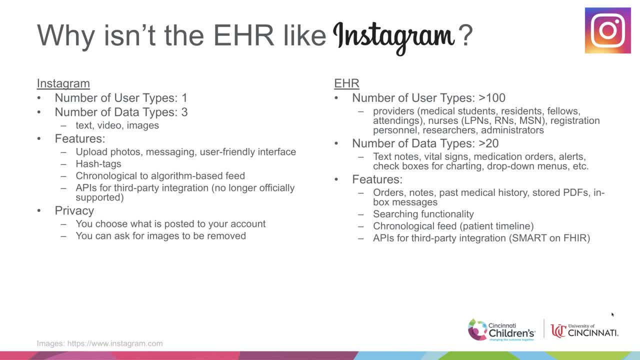 where your providers message each other about your care, Or reminders could be sent to your provider about you and about your care, about what needs to be done in the future, just to help them out. You have a searching functionality, not entirely unlike Instagram, except no hashtags. You have a. 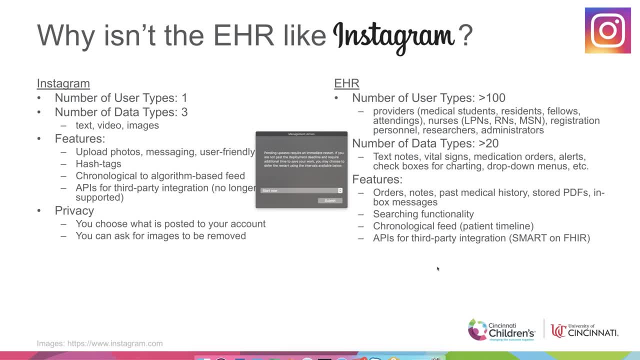 chronological feed. You can have a search for your provider. You can have a search for your provider. You can have a chronological feed which is a patient timeline. You have an interruptive alert that comes up in the middle of your presentation. What a great example. Thank you, Microsoft. So you have searching functionality. You have 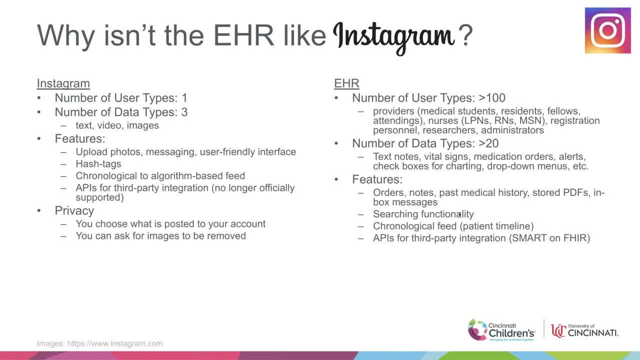 a chronological feed So you can go back through and say, from the time this patient entered the emergency department to the time they left, what happened, what different courses of action were taken and who came in contact with them. And then, finally, you also have APIs for third-party integration to get data into and out of the EHR. 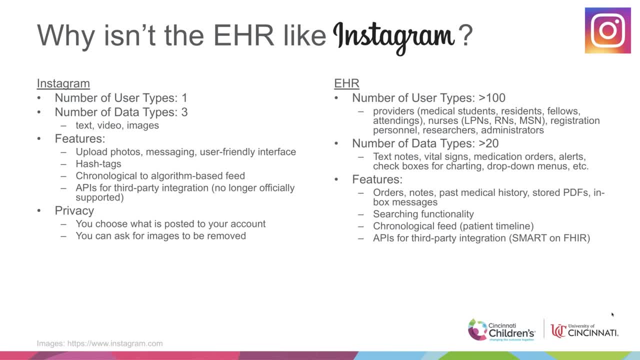 You have a searching functionality not entirely unlike Instagram, except no hashtags. You have a chronological feed, which is a patient timeline. There we go. You have an interruptive alert that comes up in the middle of your presentation. What a great example, Thank. 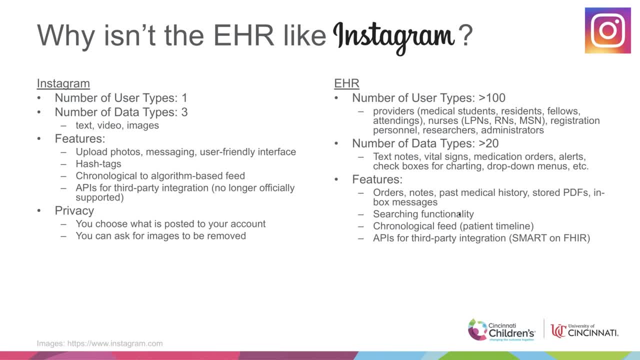 you Microsoft, So you have searching functionality. You have a chronological feed So you can go back through and say, from the time this patient entered the emergency department to the time they left, what happened, what different courses of action were taken and who. 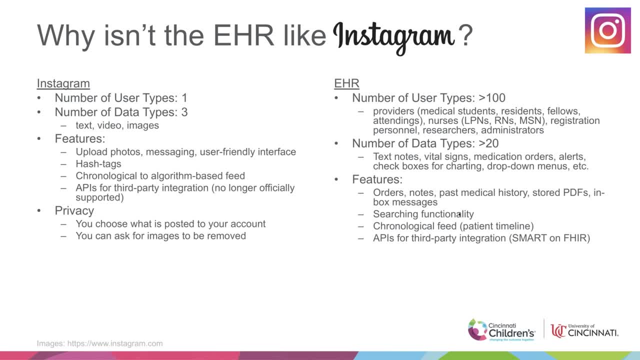 came in contact with them. And then, finally, you also have APIs for third-party integration to get data into and out of the EHR. And so what's another option, which is privacy. So there are audit logs just the same. with you can track who accessed your record, every single click. 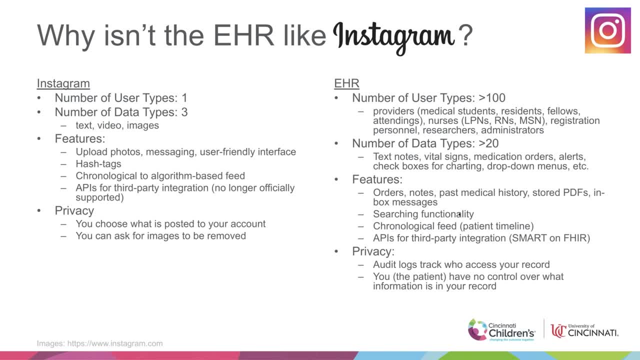 everything you do in the EHR is stored, And you, the patient, unfortunately have no real control over what information is in your record. You can send a message and say I don't believe this is correct, and this gets logged in your record as well, but this doesn't actually provide any. 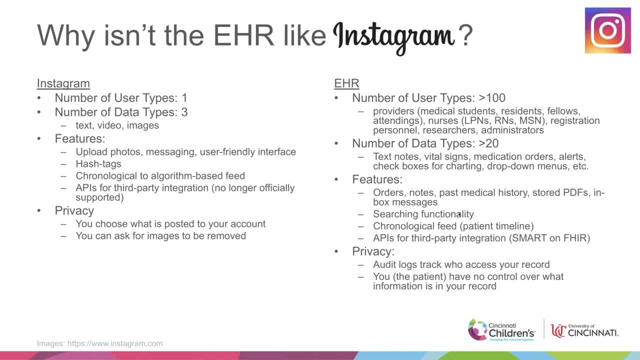 updates to your record, and it doesn't say remove a diagnosis that you, the patient, may not agree with. These are all wonderful, but there's actually more things that the EHR has to deal with, including regulatory compliance and safety issues. All of these things together combine to say why the EHR 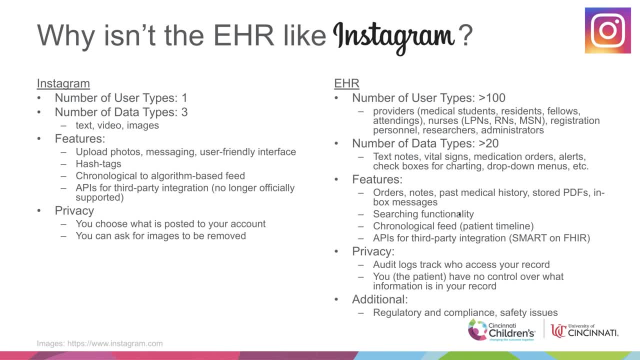 front end isn't necessarily clean, beautiful and easy to use. It's trying to do a whole lot of things, And so now- now, hopefully I've convinced you that, wow, there's a lot of stuff in there- What can we do to make it easier for users? What can we do to access some of those data? 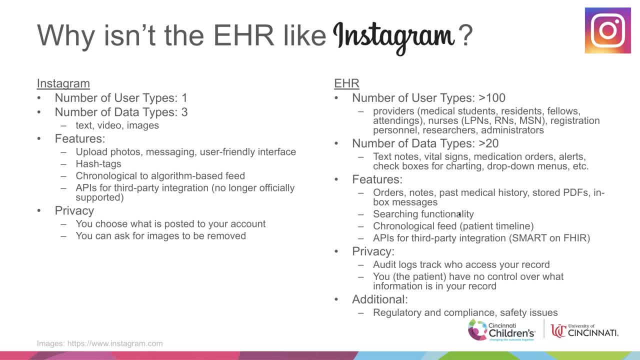 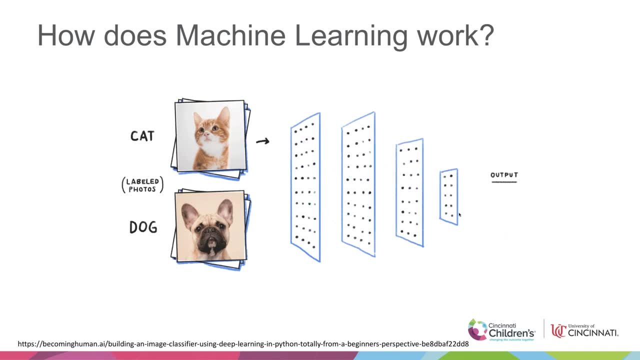 pull important things together and then provide it to users so that they can see it when they need it. So this is where I'm going to give the easiest simple overview of machine learning. So what we could do with all these EHR data is we could use: 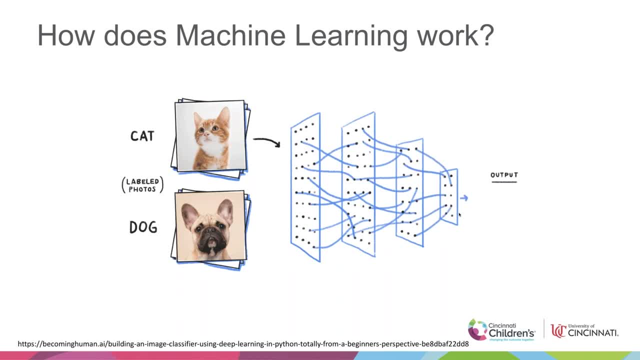 machine learning. We could take a bunch of the complex information, we could filter it down to what's the most important in the most number of patients, and then we could give it to the providers and say: you know what? I think you should consider this. So here's my sample explanation. 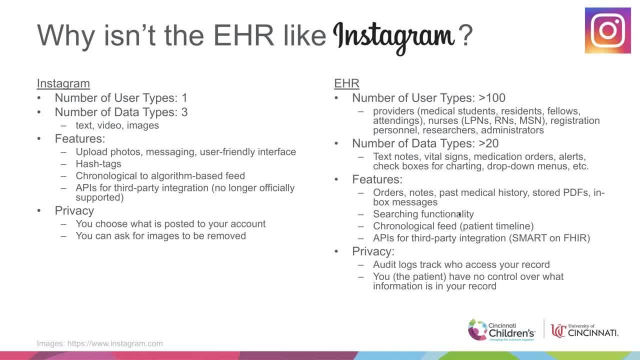 And so what's? another option, which is privacy. So there are audit logs, Just the same. with you can track who accessed your record, every single click, Everything you do in the EHR is stored, And you, the patient, unfortunately have no real control over what information is in your record. You can send a message and say: 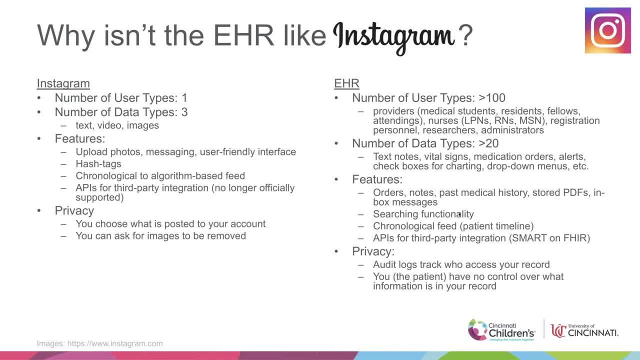 I don't believe this is correct, And this gets logged in your record as well, But this doesn't actually provide any updates to your record And it doesn't say remove a diagnosis that you, the patient, may not agree with. These are all wonderful, but there's actually more things that the EHR has to deal with, including: 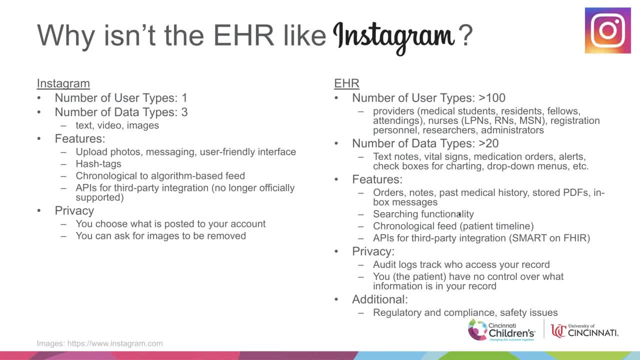 regulatory compliance and safety issues. All of these things together combine to say why the EHR front end isn't necessarily clean, beautiful and easy to use. It's trying to do a whole lot of things, And so now- now, hopefully, I've convinced you that, wow, there's a lot of stuff in there. 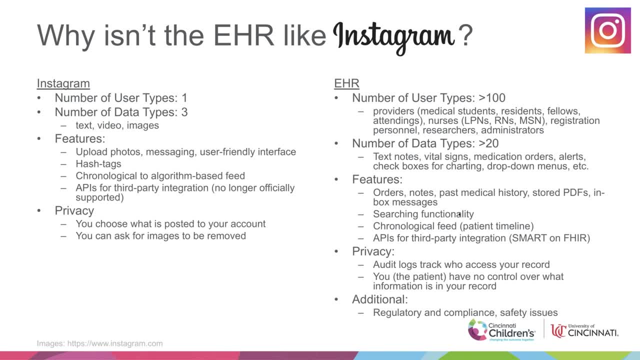 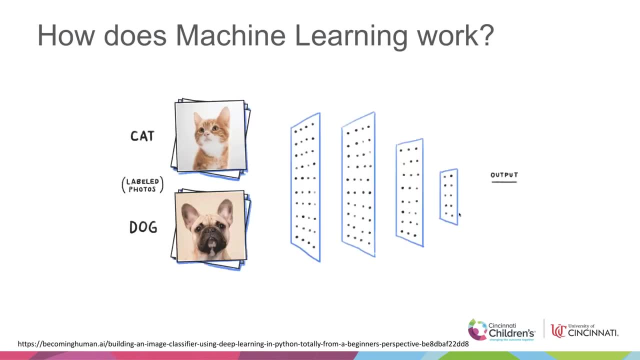 What can we do to make it easier for users? What can we do to access some of those data, pull important things together and then provide it to users so that they can see it when they need it? So this is where I'm going to give the easiest simple overview of machine learning. 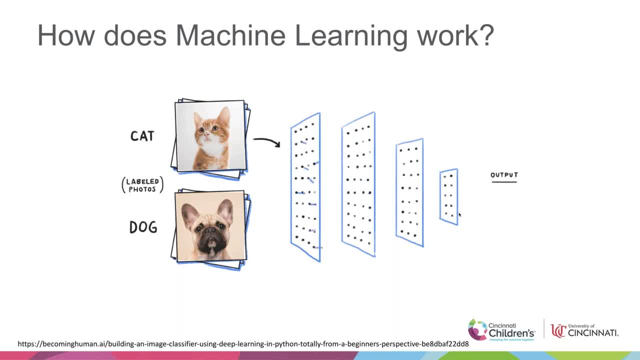 So what we could do with all these EHR data is we could use machine learning. We could take a bunch of the complex information, We could filter it down to what's the most important in the most number of patients, And then we could give it to the providers and say: you know what? I think you should consider this. 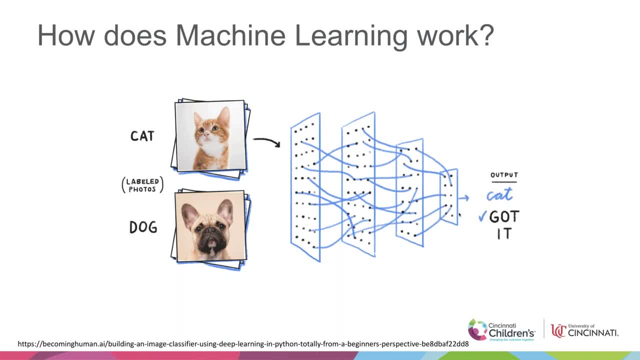 So here's my sample explanation. Here you have two sets of labeled pictures. One stack of pictures is labeled cat, One stack of pictures is labeled dog. This is supervised machine learning. Someone said: these are cats, These are dogs. And then what we did with these things that I have helpfully called cheese graters? 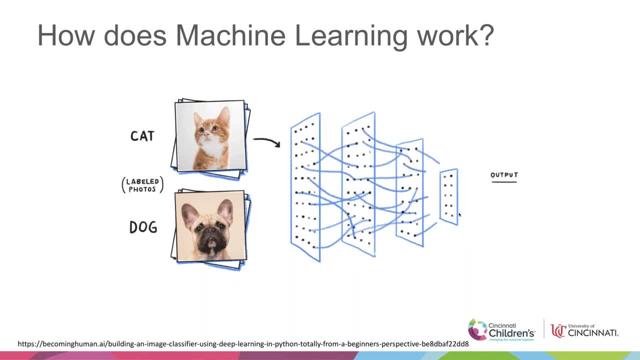 here in the middle. these are really the machine learning input layers. This is really the model that we created and trained to tell the difference between the picture of a cat and a picture of a dog. So then, when we show it a brand new picture of a cat, that it's. 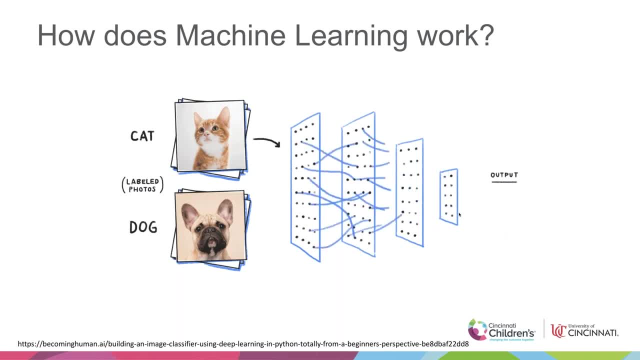 Here you have two sets of labeled pictures. One stack of pictures is labeled cat, one stack of pictures is labeled dog. This is supervised machine learning. Someone said: these are cats, These are dogs. And then what we did with these things that I have helpfully called cheese? 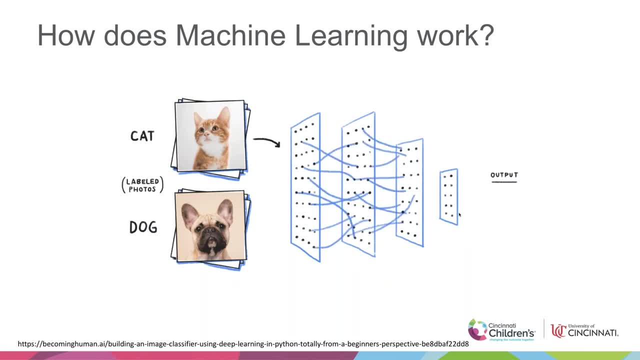 craters here in the middle. these are really the machine learning input layers. This is really the model that we created and trained to tell the difference between the picture of a cat and a picture of dog. so then, when we show it a brand new picture of a cat that it's never seen, 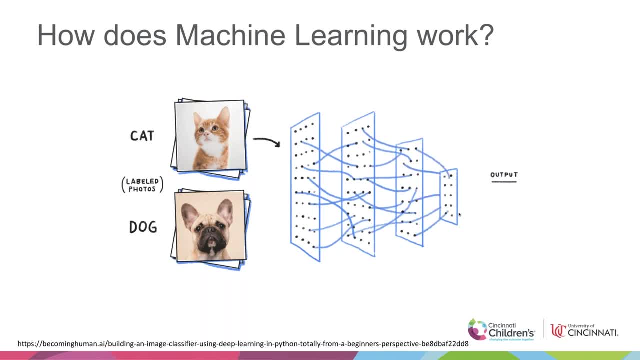 before it goes through all of these layers and the output is: what is it? and in this case it's a cat. the machine is correct. great job. we've classified it correctly and we have used machine learning on a brand new set of data based on something we've trained it on. we're going to talk about primarily. 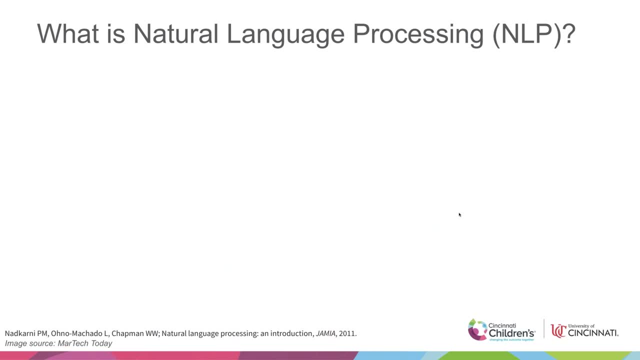 natural language processing, which is part of why I've stressed how important it is that most of the data in the EHR is in unstructured notes. so natural language processing in the briefest sense is using a computer to get meaning out of text-based data. so I'm going to show you similar to the picture before. 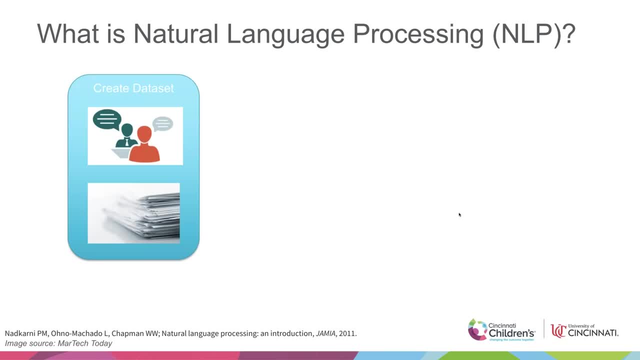 what it is we do to create natural language processing, to create a new algorithm and then to apply it to new situations. and so this first picture is: the first thing we do is create a data set. we're going to create a data set and then we're going to create a data set. 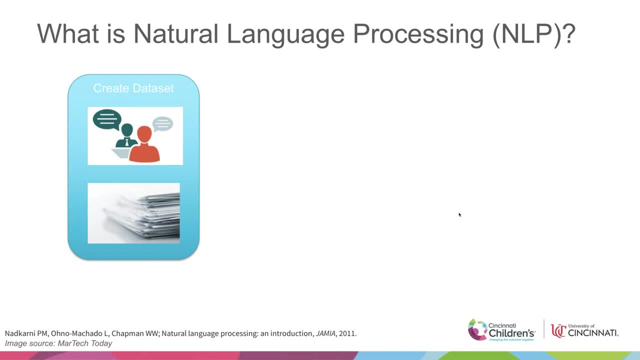 we talk to people, we create it different ways. we pull records, we pull it data from the EHR. we create a great robust data set that includes everything we need. then what do we do then? we create and train a model. what you see down here on the bottom half of the middle screen is an example of 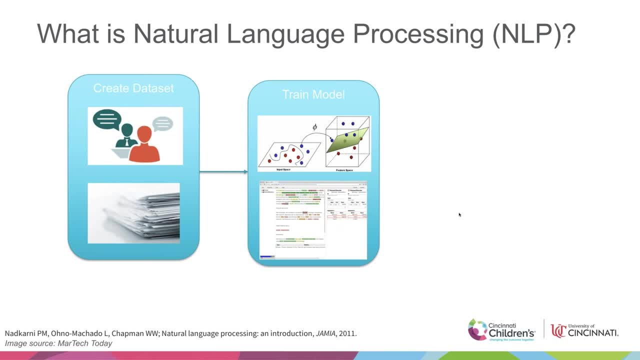 annotation. this is a clinical note that a human has gone through and annotated and said: these items are important for this thing, these items are not important for something else. and so we do this with a subset of notes. and again, this is a supervised machine learning. and then we 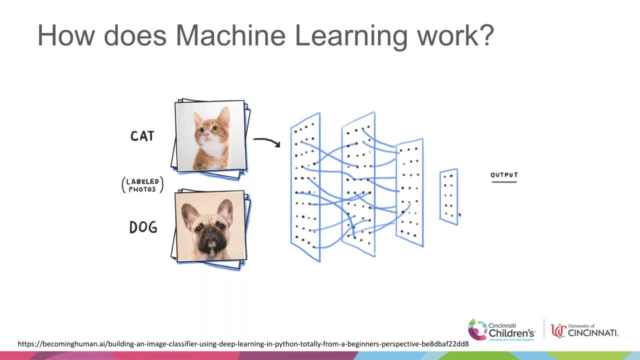 never seen before. it goes through all of these layers and the output is: what is it? And in the case it's a cat. The machine is correct. Great job. We've classified it correctly and we have used machine learning on a brand new set of data, based on something we've trained it on. 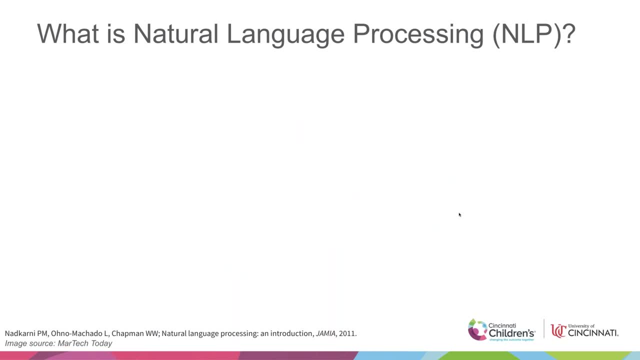 We're going to talk about primarily natural language processing, which is part of why I've stressed how important it is that most of the data in the EHR is in unstructured notes. So natural language processing in the briefest sense is using a computer to get meaning out of. 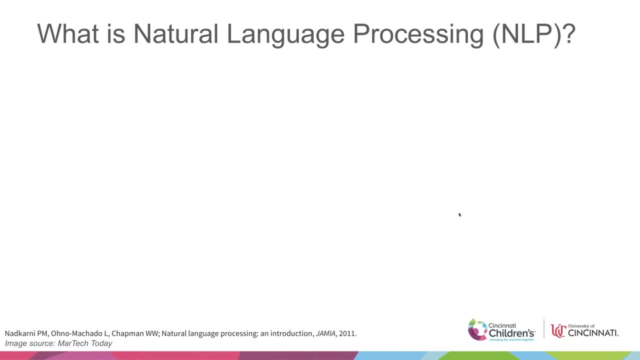 text-based data. So I'm going to show you, similar to the picture before, what it is we do to create natural language processing, to create a new algorithm and then to apply it to new situations, And so this first picture is the first thing we do is create a data set. We talk to people. 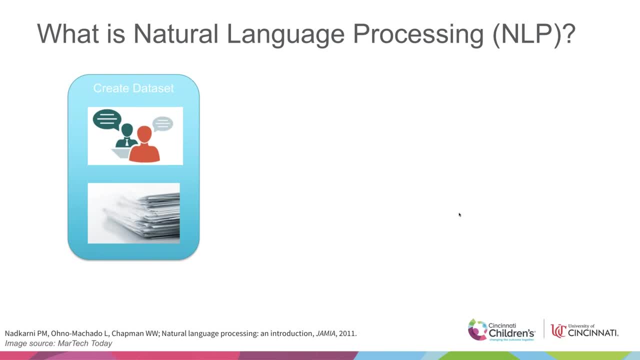 we create it different ways. we pull records, we pull data from the EHR. we create a great robust data set that includes everything we need. Then what do we do Then? we create and train a model, What you see down here on the bottom half of the middle screen. 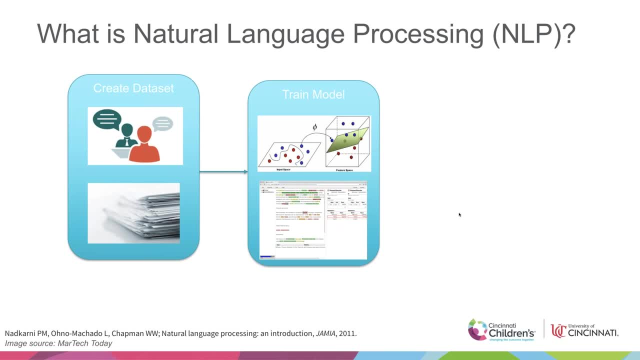 is an example of annotation. This is a clinical note that a human has gone through and annotated and said: these items are important for this thing, These items are not important for something else, And so we do this with a subset of notes. And again, this is the supervised machine learning. 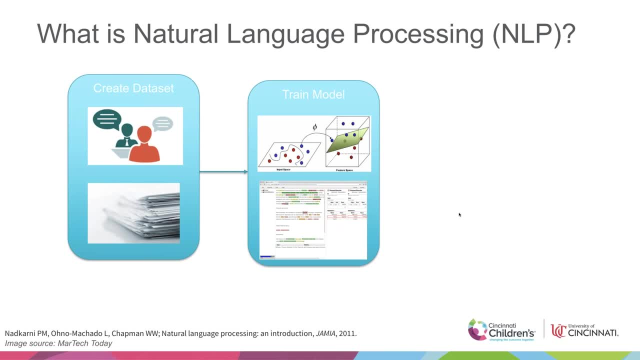 And then we have two sets of outcomes: cases and controls. The top half of this image has the cases and controls. We have blue and we have red dots. What we do is we put this into our machine learning algorithm and then we try to draw a line. That's what's happening in the box that says feature space. 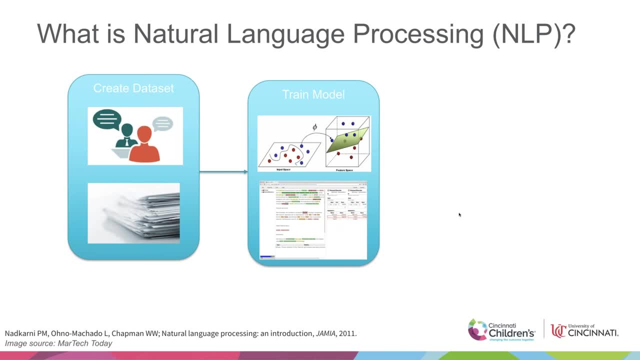 And we try to differentiate so that when we see someone brand new we can tell whether you're a blue dot or you're a red dot And from this point of course, then we can make predictions on future data. So we can say: we have this whole new set of data. 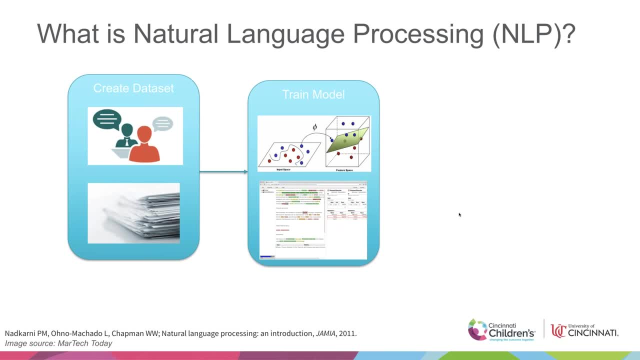 have two sets of outcomes: cases and controls. the top half of this image has the cases and controls. we have glue and we have red dots. but we do is we put this into our machine learning algorithm and then we try to draw a line. that's what's happening in the box. this is the sort of low dyke love that you won't see. i'm sorry, I know. like I said, it's not much better than the first kilometer. okay, without the addition of American trees. you predict how the results will be will be pretty obvious, but the only erle fact of all things are the errors. larger lined boxes are easier to slow down. would you be surprised that research? 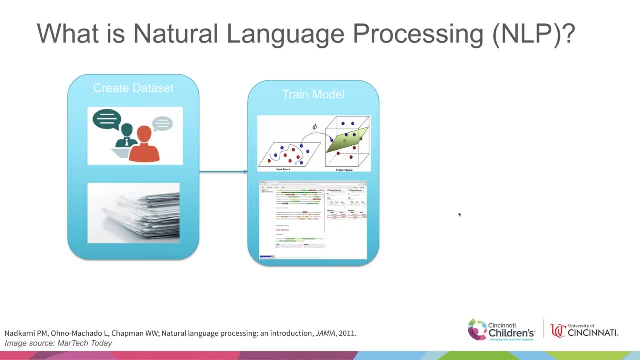 feature space and we try to differentiate so that when we see someone brand new, we can tell whether you're a blue dot or you're a red dot and from this point of course, then we can make predictions on future data. so we can say: we have this whole new set of data, what is it that you are? and then 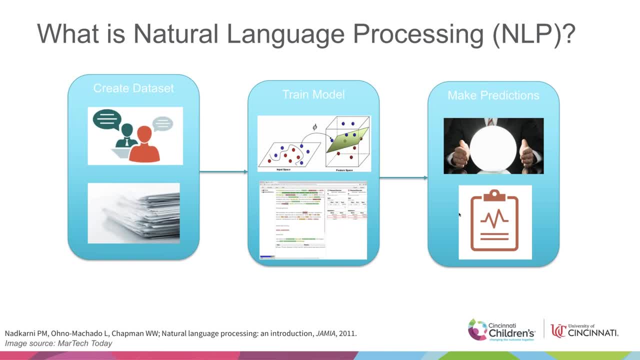 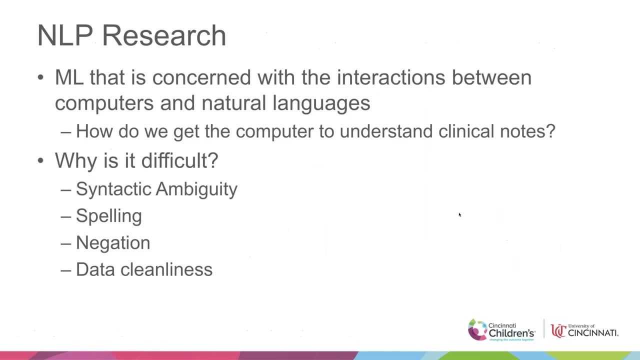 we can say, based on our past information, it turns out you're going to be a red dot, and then we can evaluate whether or not we're correct and we can give this information to providers. so with nlp research, so natural language processing, it's machine learning, that's. 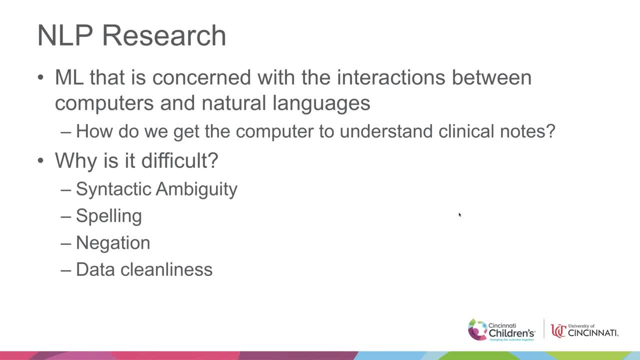 concerned with the interactions between computers and natural languages and the how do we get the computer to understand clinical notes? and so let's do a couple of light caveats about why it's difficult. the first one: syntactic ambiguity. this one is my favorite example, and it's: time flies like an arrow, fruit flies like a banana. 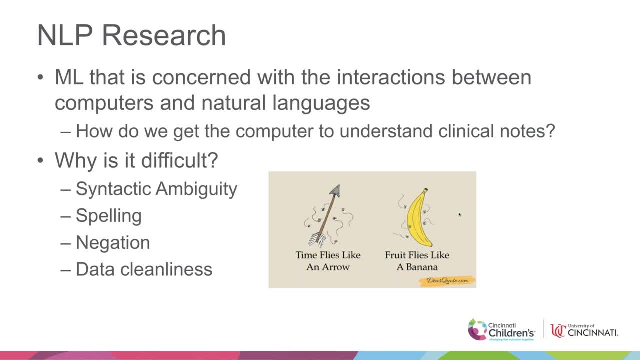 you, as a human, know the difference between these two sentences. the computer does not, and we need a way to teach the computer what the differences are when we look at these two types of things. a second one of these is basic spelling. we're looking at free text notes. 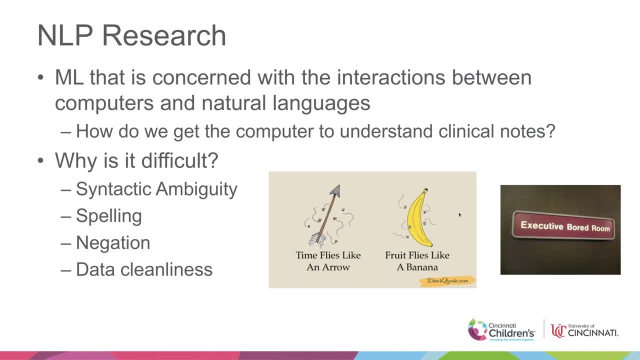 and people make mistakes sometimes in spelling when they're typing. you know this from autocorrect. everyone has used it and loved it and hated it on things like their phones in this case. this is another one of my favorite examples because it has so many meetings. the executive boardroom does get the meaning across, but it's not necessarily. 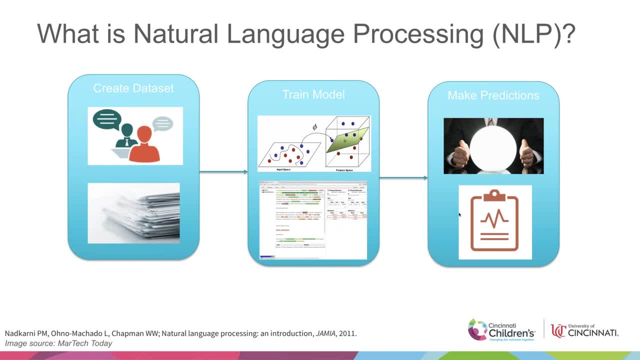 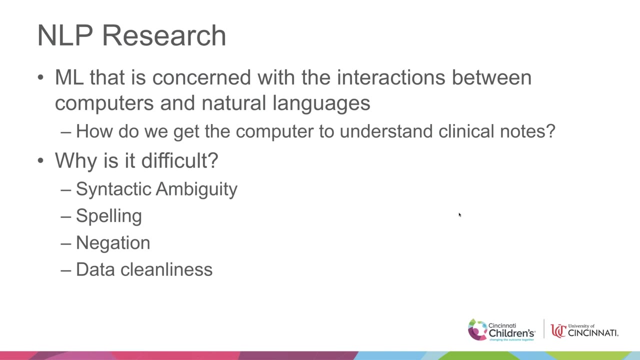 What is it that you are? And then we can say, based on our past information, it turns out you're going to be a red dot, And then we can evaluate whether or not we're correct And we can give this information to providers. So, with NLP research, so natural language processing, it's machine. 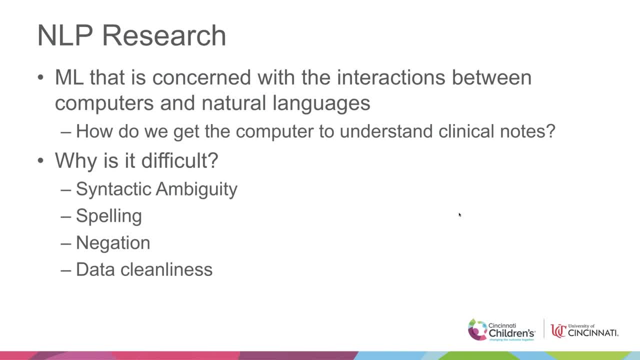 learning. that's concerned with the interactions between computers and natural languages. So in a way it's like getting our word out of the water. The emotion is a little bit different. So the chemical is like: how about we get this thing together? see how we get the computer. 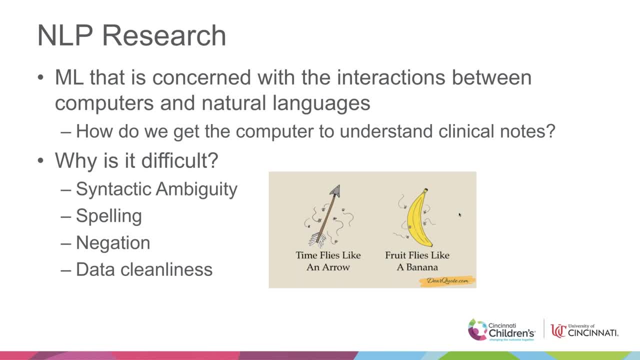 to understand clinical notes, And so let's do a couple of like caveats about why it's difficult. The first one: syntactic ambiguity. This one is my favorite example, And it's: time flies like an arrow, fruit flies like a banana. 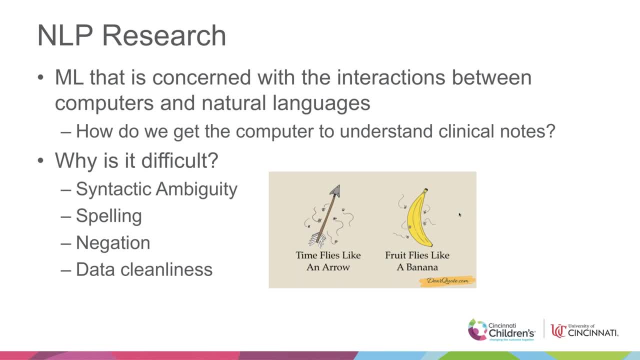 You, as a human, know the difference between these two sentences, what the differences are when we look at these two types of things. a second one of these is basic spelling. we're looking at free text notes and people make mistakes sometimes in spelling when they're typing. you know this from. 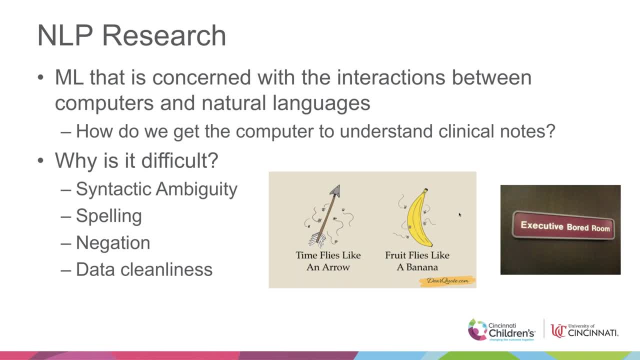 autocorrect. everyone has used it and loved it and hated it- on things like their phones in this case. this is another one of my favorite examples because it has so many meetings. the executive boardroom does get the meaning across, but it's not necessarily what we want to have happening here. the 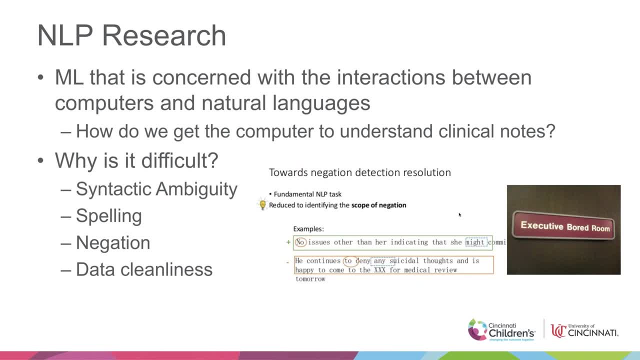 next is negation, and this is an example from Google, from an idea of clinical negation. so here's an example. so the first one on top is: there are no issues other than her indicating that she might commit suicide. there is clearly a negation here and there's something else that's important. and then the second one. 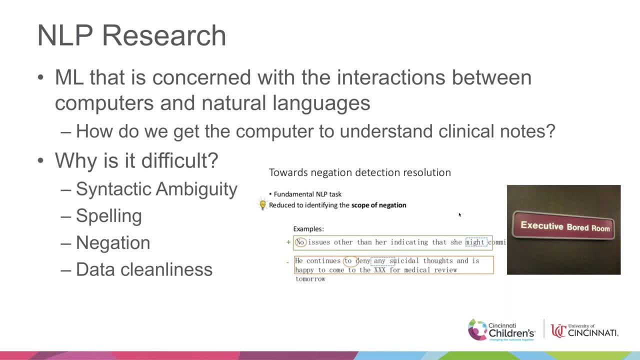 is that he continues to deny any suicidal thoughts and is happy to come, etc. etc. these two things mean very different things. however, there's a lot of different processing that you, the human, go through before you say, oh no, the first one is someone I might be concerned about and the second one I'm 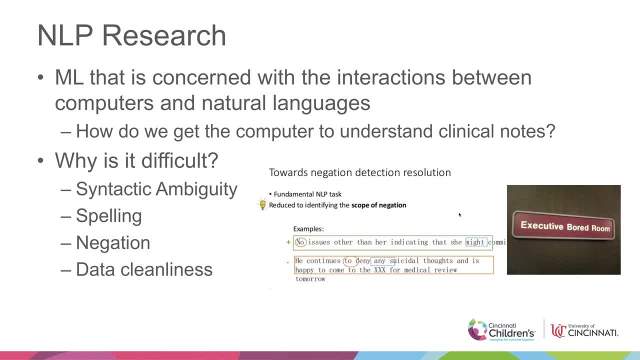 what we want to have happening here. the next is negation, and this is an example from google, from um, an idea of clinical negation. so here's an example. so the first one on top is: there are no issues other than her indicating that she might commit suicide. there is clearly a negation here. 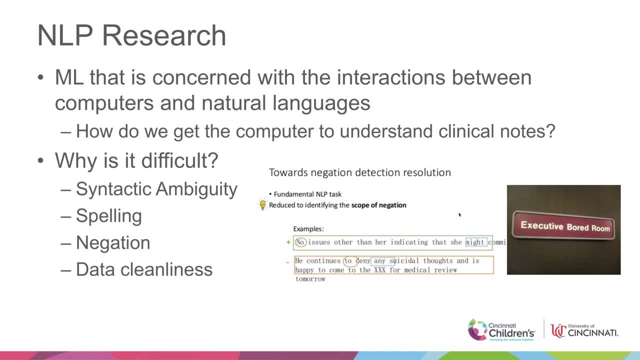 and there's something else that's important. and then the second one is that he continues to deny any suicidal thoughts and is happy to come, etc. etc. these two things mean very different things. however, there's a lot of different processing that you, the human, go through before you say: 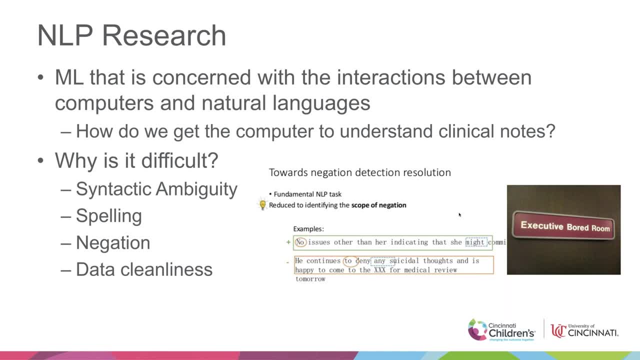 oh no, the first one is someone i might be concerned about and the second one i'm not. and then the third thing, of course, is just data cleanliness. so you have a lot of data and it was not collected for research purposes, and so it's wonderful for clinical care, but it's not necessarily wonderful the way it is, for 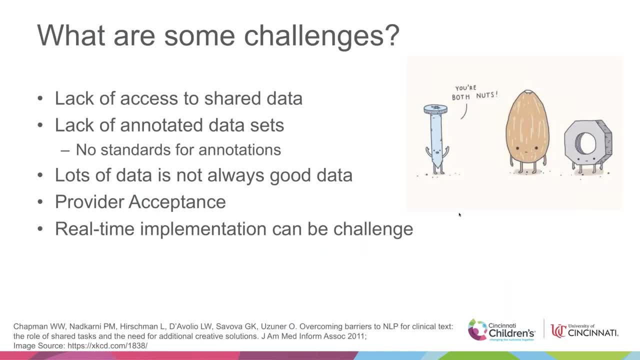 research. so what are some of the overall challenges with basically all database product projects? one of them is a lack of access to shared data. there are a lot of data out there, but there aren't a lot of shared data that we can openly access and do everything with. there's a lack of 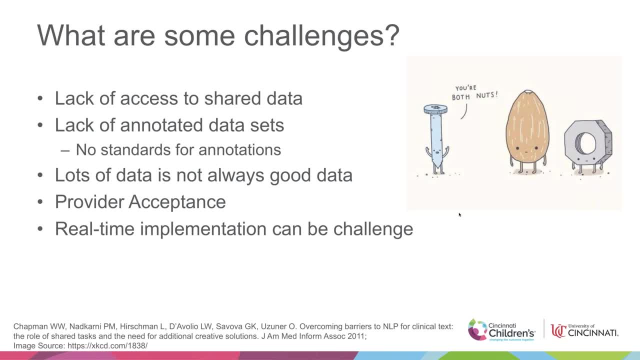 annotated data sets. in that previous slide, i showed you that we needed to annotate a lot of our data sets to be able to make predictions based on and there's no standards for annotations. so even if we annotate all of our data sets, we won't necessarily be able to share them with another. 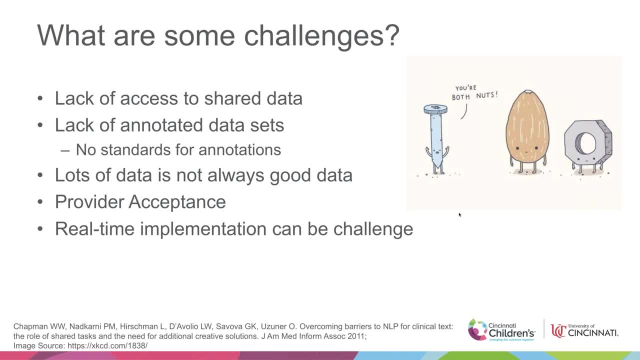 institution. lots of data, of course, is not always good data, so more is not always better. and then one of the issues is provider acceptance from the machine learning recommendations. you need to have your provider, your end user, someone, included at all times, from the very start, so that they feel 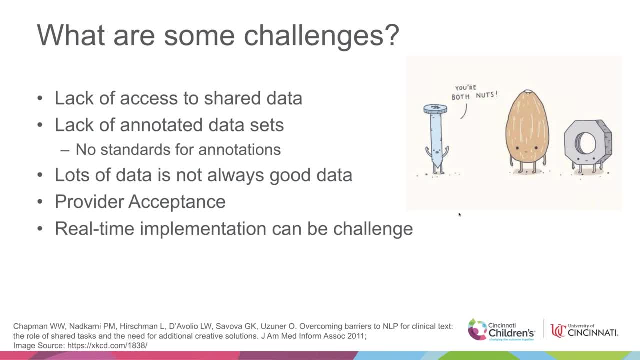 comfortable with the recommendations, that are, computers providing them. and then the last is: real-time implementation can be a challenge. one of the goals in informatics is to hit the real-time implementation with the right person, the right time, the right information, and so these all just need to be planned in advance. 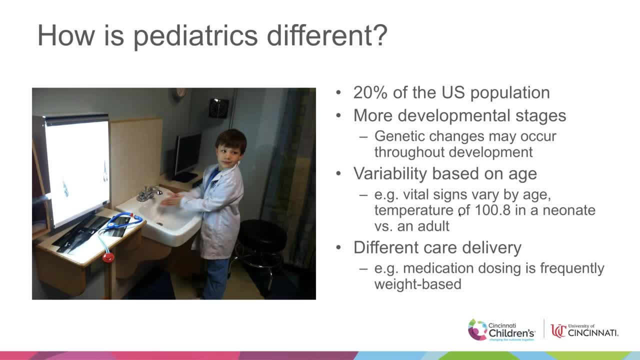 so i'm going to step into some nlp implementations that we've done and i'll talk about that in a little bit, but i want to give you a brief description of like things to incite discussion about what the future might hold. but i want to take a step back because 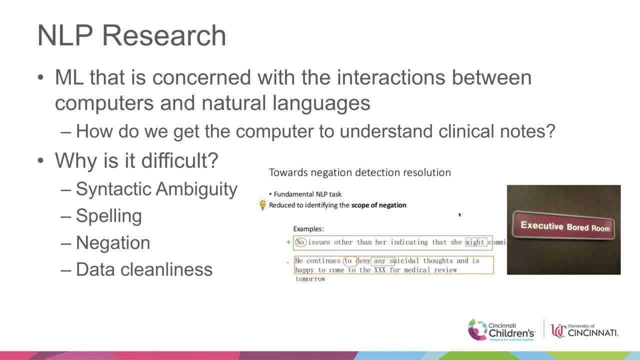 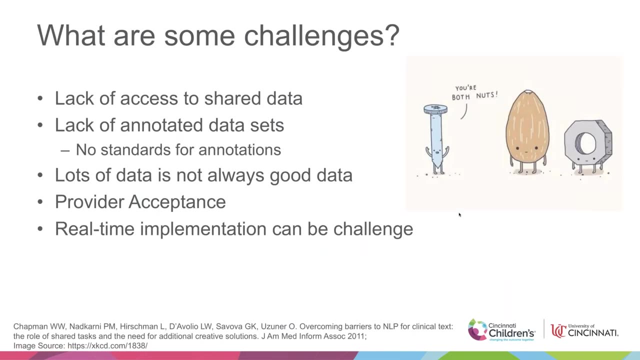 not. and then the third thing, of course, is just data cleanliness. so you have a lot of data and it was not collected for research purposes, and so it's wonderful for clinical care, but it's not necessarily wonderful the way it is for research. so what are some of the overall challenges with basically all database? 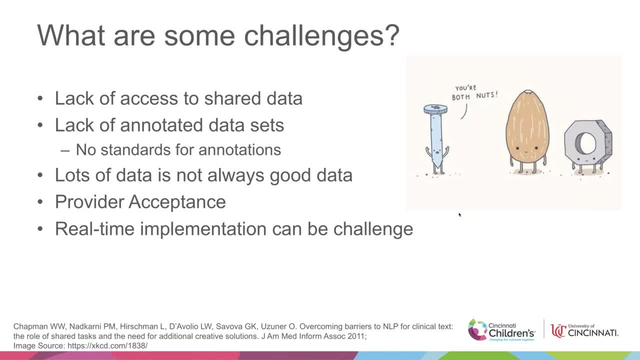 product projects. one of them is a lack of access to share data. there are a lot of data out there, but there aren't a lot of shared data that we can openly access and do everything with. there's a lack of annotated data sets. in that previous slide, I showed you that we needed to annotate a lot of our datasets to be 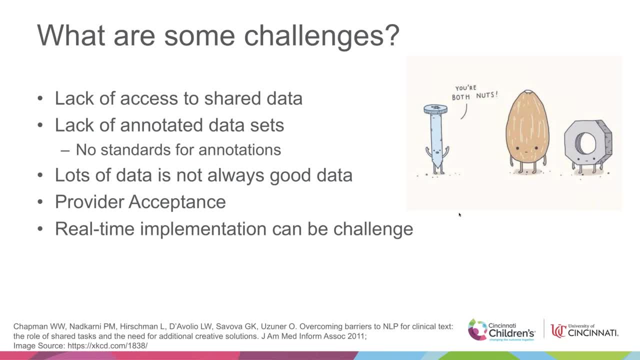 able to make predictions based on our and there's no standards for annotations. so even if we annotate all of our datasets, we won't necessarily be able to share them with another institution. lots of data, of course, is not always good data, so more is not always better. and then one of the issues is provider acceptance from the machine learning. 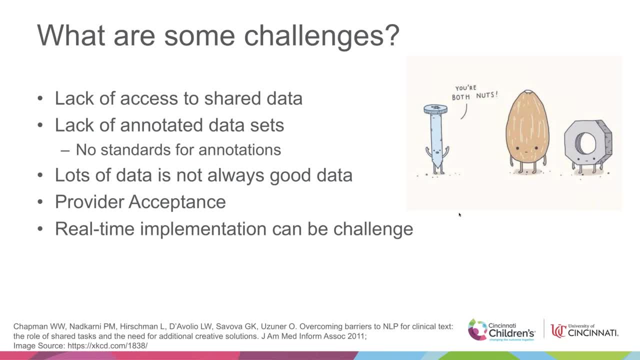 recommendations. you need to have your provider, your end user, someone included at all times, from the very start, so that they feel comfortable with the recommendations that are computers providing them. and then the last is real-time implementation can be a challenge. one of the goals in informatics. 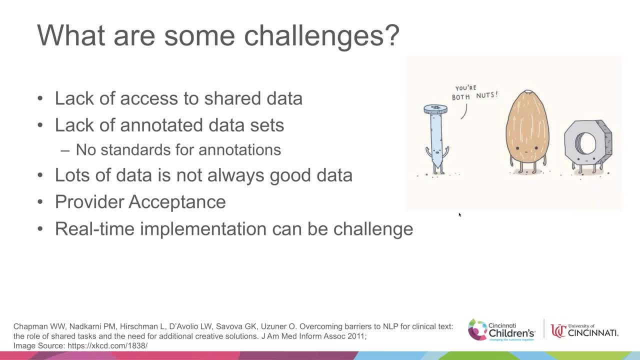 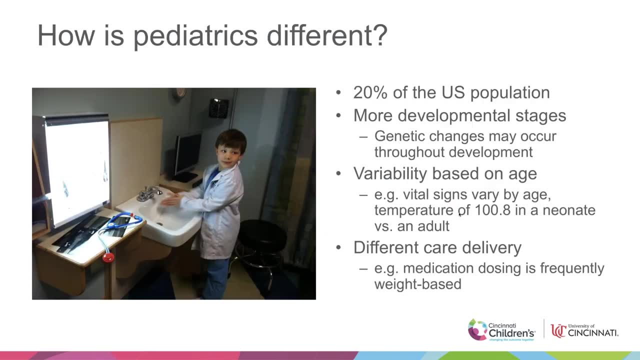 is to hit the real-time implementation with the right person, the right time, the right information, and so these all just need to be planned in advance. so i'm going to step into some nlp implementations that we've done, along with a brief description of like things to incite discussion. 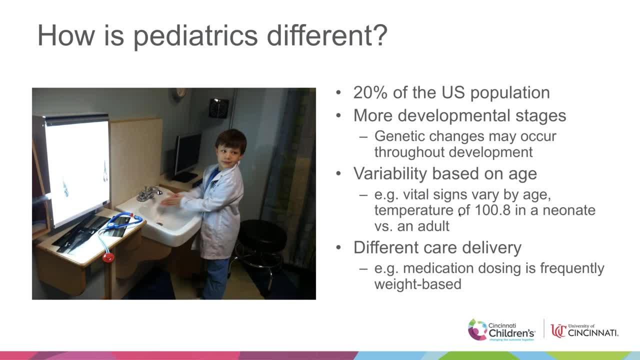 about what the future might hold. but i want to take a step back, because i'm based at a pediatric institution, so let's examine how pediatrics might be different. about 20 percent of the united states population is pediatric. are they really just tiny adults? no, unfortunately they aren't. 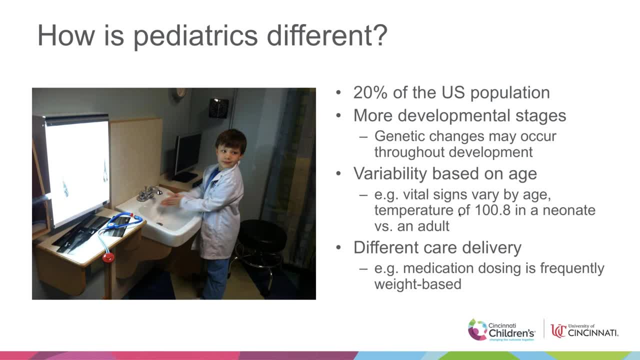 eventually they'll be adults, but now, while we're looking at them, and so they have more developmental stages, and so, from the genomic side, what this means is that genetic changes may occur throughout the child's development, and so things may need to be rerun and reevaluated. they have a lot of 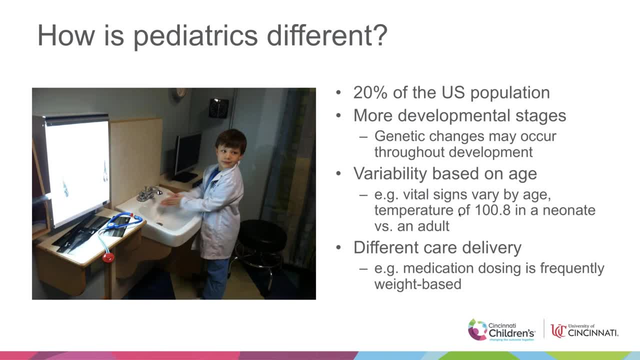 i'm based at a pediatric institution, so let's examine how pediatrics might be different. about 20 of the united states population is pediatric. are they really just tiny adults? no, unfortunately they aren't. eventually they'll be adults. but now, while we're looking at them, 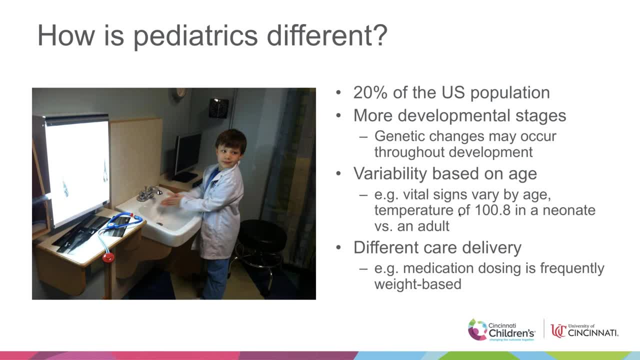 and so they have more developmental stages, and so this means is that genetic changes may occur throughout the child's development, and so things may need to be rerun and reevaluated. they have a lot of variability based on age that's not necessarily apparent in an adult side. so, for example, a vital sign varies by age: a temperature. 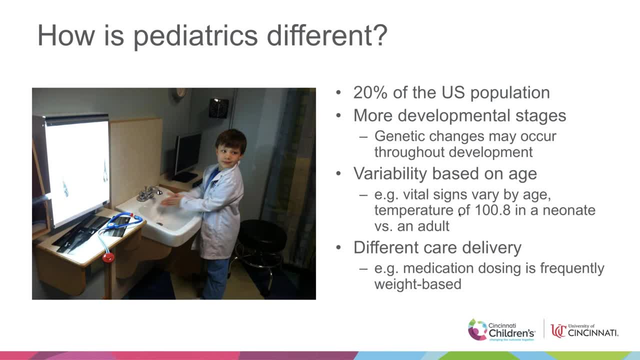 of 100.8 degrees and a neonate maybe calls for concern, whereas if i come in as an adult with a temperature of 100.8 degrees, nobody is all that concerned. and really why did i go in necessarily that day? and then the other thing is there are different modalities of care delivery, so medication. 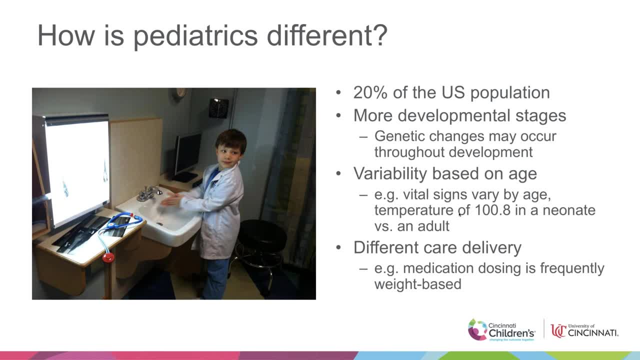 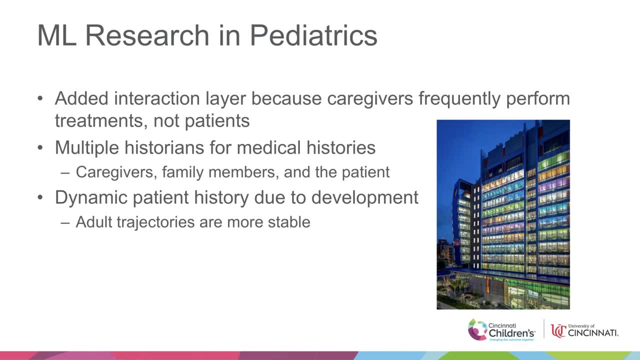 dosing is frequently weight based in pediatrics, whereas it's not on the adult side, and so this adds a whole new layer of things to think about while we build our decision support in the end. so more of the stuff on machine learning research in pediatrics. one of the issues, of course, is an 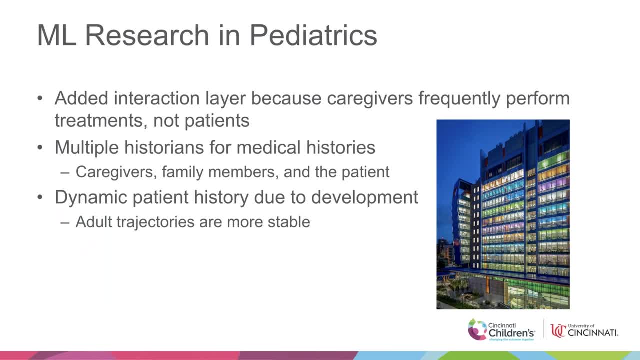 added interaction layer, because it's the caregiver, not the patient, that might be performing a required or suggested treatment. the patients are fairly not autonomous yet, and so they are not the only ones participating in their own care. another is that there's multiple historians for medical histories, so it's not just me saying here were my symptoms over the past three weeks. 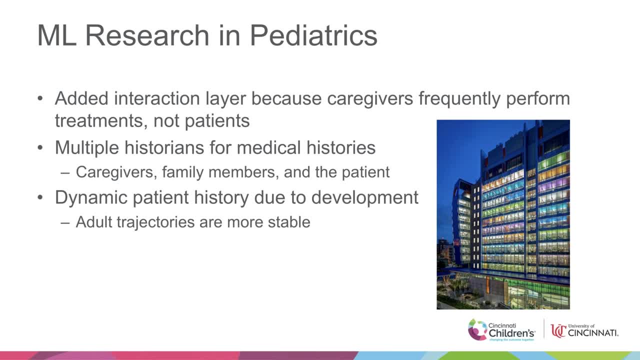 but it could be any caregivers, including mom and dad, family members or someone else, and the patient as they get older, and all of these different lines need to come together to make a cohesive narrative, and which is a challenge for the pediatricians but also a challenge on the machine learning side. 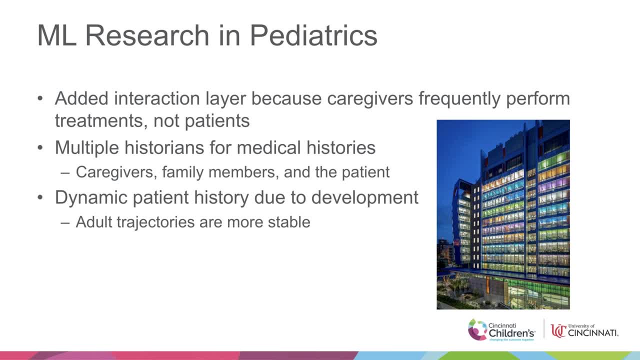 and then the last thing is that there can be a dynamic patient history due to development. adult trajectories are typically more stable, so it was important to note and to report, when my child was between 6 and 12 months of age, what solid food he ate, that he ate solid food and how he tolerated. 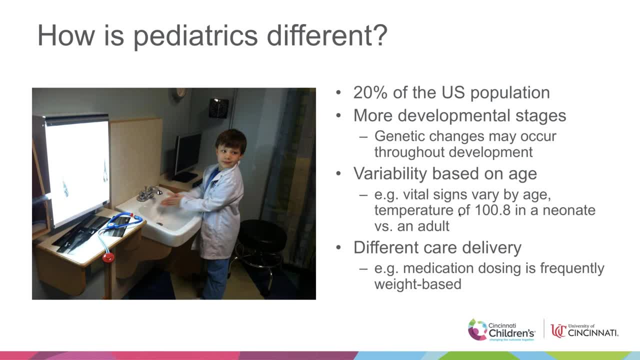 variability based on age. that's not necessarily apparent in an adult side. so, for example, a vital sign varies by age. a temperature of 100.8 degrees and a neonate maybe calls for concern, whereas if i come in as an adult with a temperature of 100.8 degrees, nobody is all that concerned. and 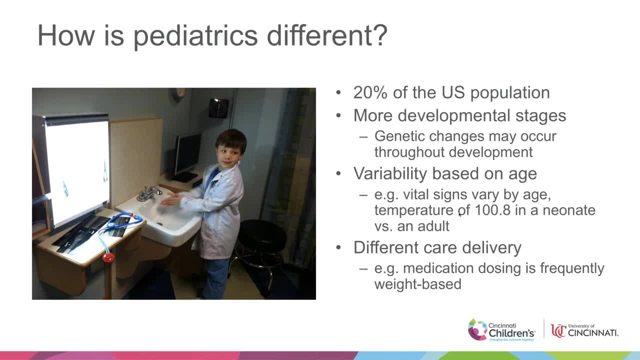 really, why did i go in necessarily that day? and then the other thing is there are different modalities of care delivery, so medication dosing is frequently weight-based in pediatrics, whereas it's not on the adult side, and so this adds a whole new layer of things to think about while we 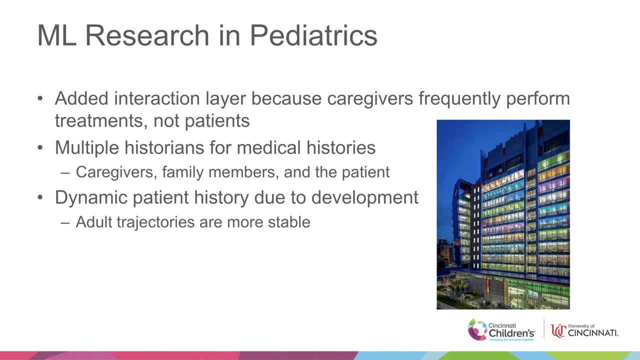 build our decision support in the end. so more of the stuff on machine learning, research and pediatrics. one of the issues, of course, is an added interaction layer, because it's the caregiver, not the patient, that might be performing a required or suggested treatment. the patients are fairly not autonomous yet, and so they are not the only ones participating in their own care. 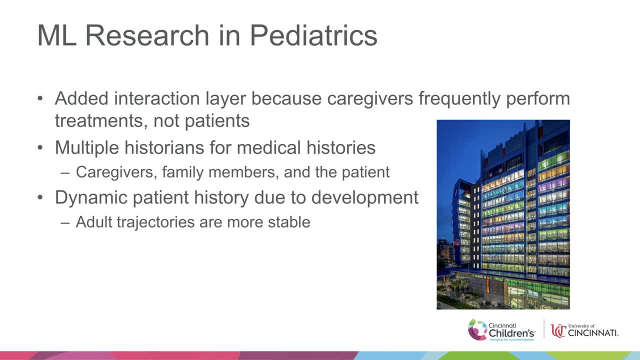 another is that there's multiple historians for medical histories, so it's not just me saying here were my symptoms over the past three weeks, but it could be any caregivers, including mom and dad, family members or someone else, and the patient as they get older, and all of these different. 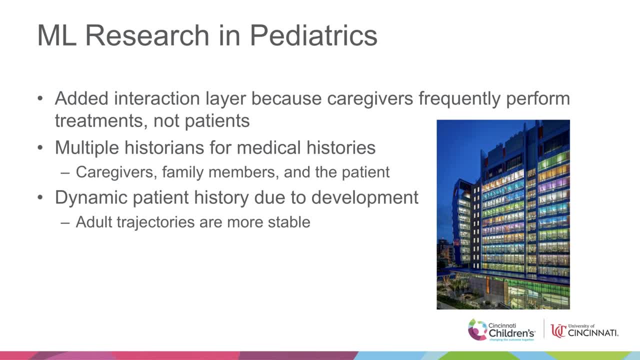 lines need to come together to make a cohesive narrative, and which is a challenge for the pediatricians, but also a challenge on the machine learning side. and then the last thing is that the patient is a very flexible person, and so we know that there can be a dynamic patient history due to 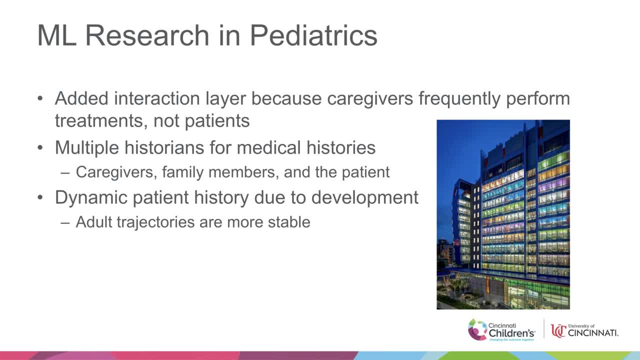 development. adult trajectories are typically more stable, so it was important to note and to report, when my child was between 6 and 12 months of age, what solid food he ate, that he ate solid food and how he tolerated it. however, now, at about 11 years old, it's currently pretty much entirely. 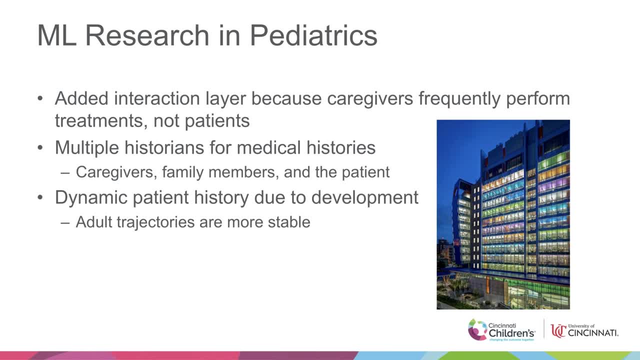 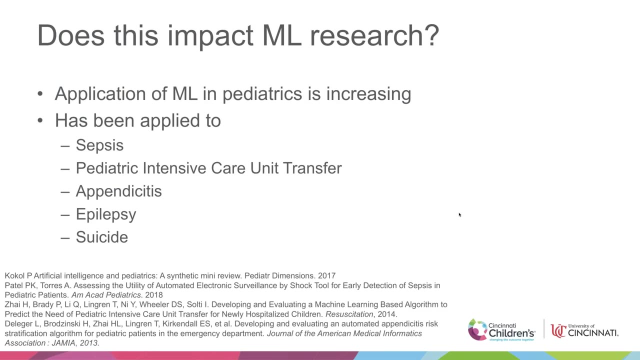 unremarkable that he's eating solid food and will remain so for most of the rest of his life, unless, as a mother, it's a vegetable, in which case that's great and important for me, but not necessarily as important for his provider. so do all these things impact machine learning research? they do, um, but machine the applications. 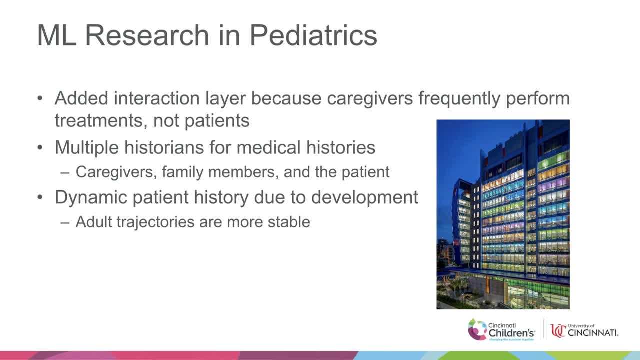 it. however, now, at about 11 years old, it's currently a little bit more difficult for him to understand the difference between solid food and solid food, and that's because he's eating solid food and will remain so for most of the rest of his life, unless, as a mother, it's a vegetable. 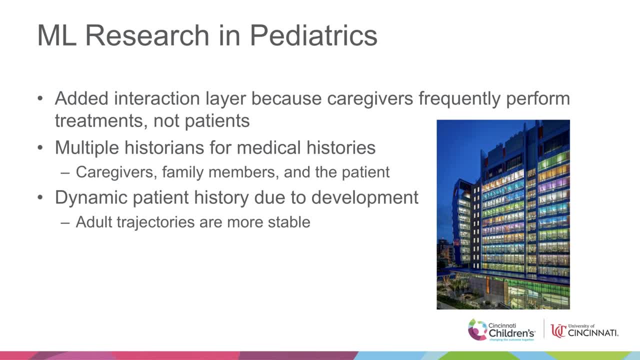 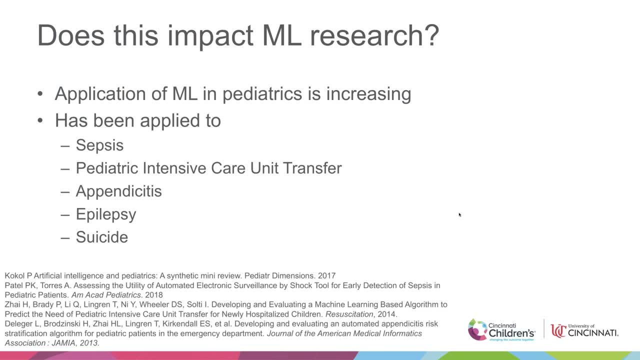 in which case that's great and important for me, but not necessarily as important for his provider. so do all these things impact machine learning research? they do, um, but machine- the applications of machine learning- in pediatrics is continuing to increase, and so machine learning has been applied in pediatrics and sepsis identification. 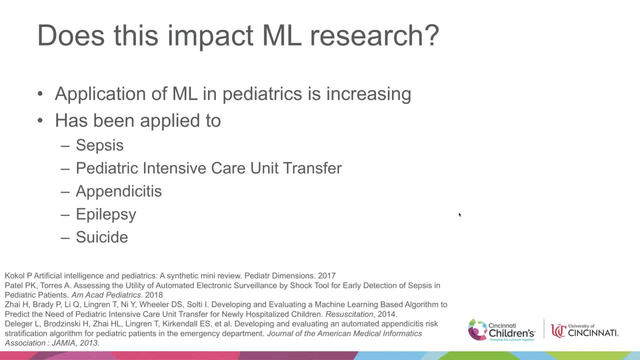 both in the emergency department and in pediatric intensive care. machine learning has been applied with pediatric intensive care unit transfer to identify people who may have appendicitis, to identify patients who may be eligible for epilepsy surgical consults, which i will talk about briefly, and to identify identify patients who may be. 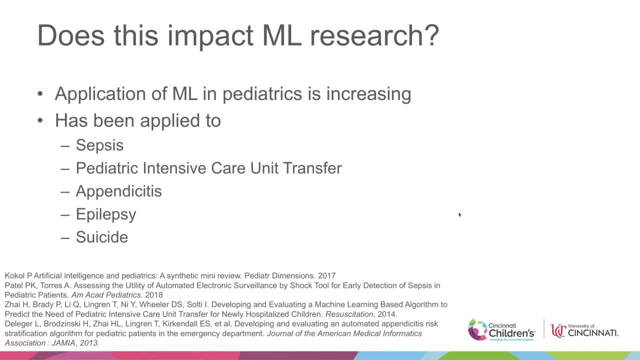 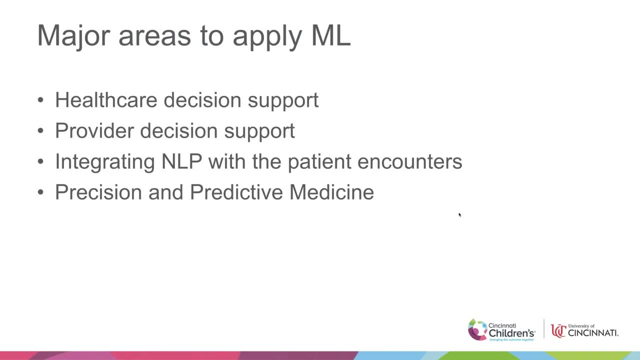 suicidal. so let's go to a couple of projects that we've done and kind of steps through things that have happened in machine learning, in pediatrics, and so i have four main categories here and each of these represents kind of a project to go through, and the first one is: 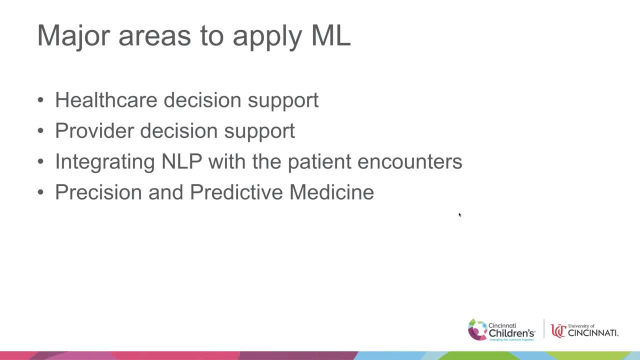 healthcare decision support. the second is provider decision support. the third would be integrating nlp with patient encounters. so it's still provider decision support, but it's directly involving the patient in their care. and then the last one is more of a future: look at precision and predictive medicine and what's. 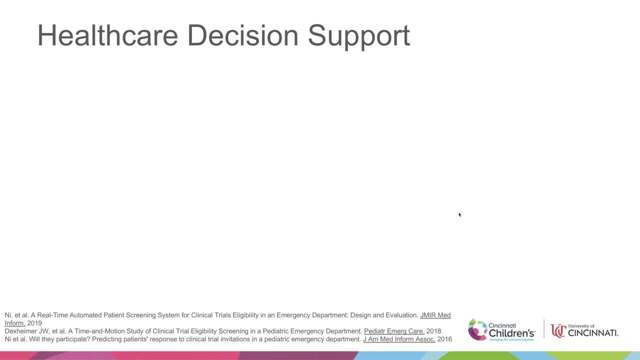 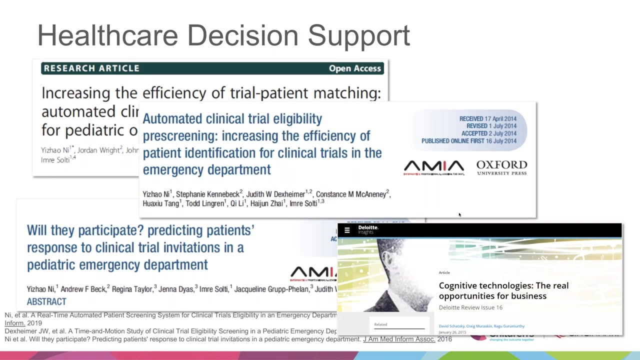 going to be coming up. so for healthcare decision support, what's important here is that we made a real-time identification system to screen patients who may be eligible for enrollment in clinical trials during their emergency department visit. and what's really important to know here is that there is a lot of retrospective background and work that goes on. 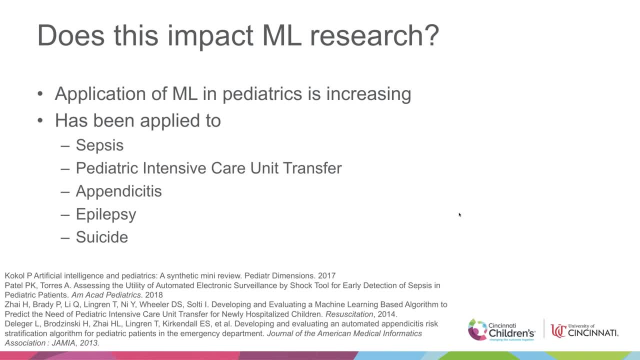 of machine learning in pediatrics is continuing to increase, and so machine learning has been applied in pediatrics and sepsis identification, both in the emergency department and in the pediatric intensive care. machine learning has been applied with pediatric intensive care unit transfer to identify people who may have appendicitis, to identify patients who may be. 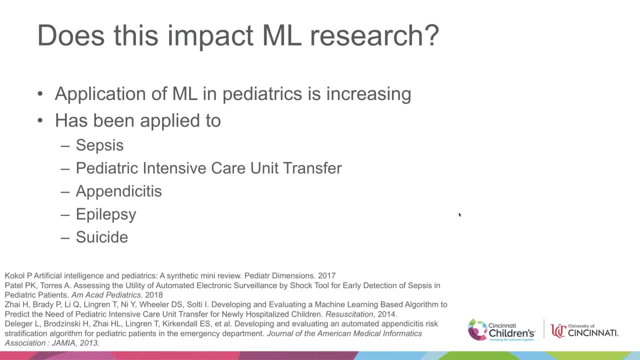 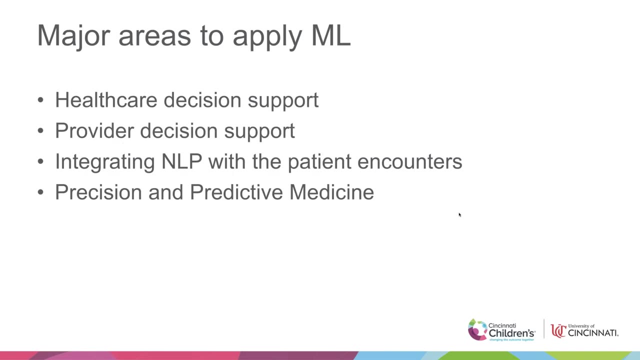 eligible for epilepsy surgical consults, which i will talk about briefly- and to identify, identify patients who may be suicidal. so let's go to a couple of projects that we've done and kind of stepped through things that have happened in our practice in machine learning, in pediatrics, and so I have four main categories here in each. 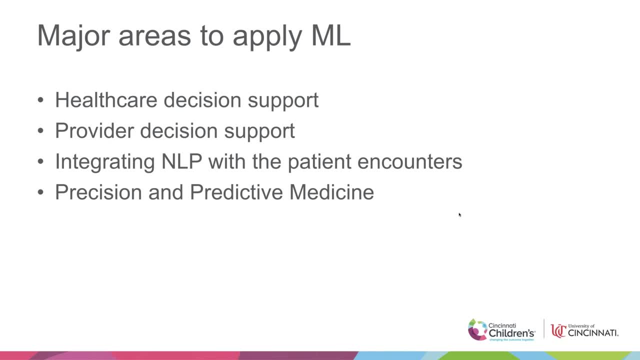 of these represents kind of a project to go through, and the first one is health care decision support, the seconds provider decision support, the third would be integrating NLP with patient encounters. so it's still provider decision support, but it's directly involving the patient in their care and 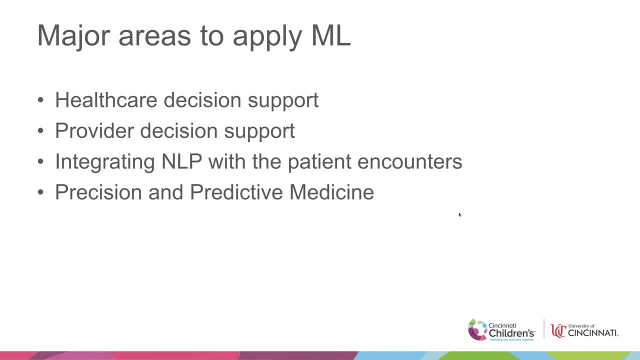 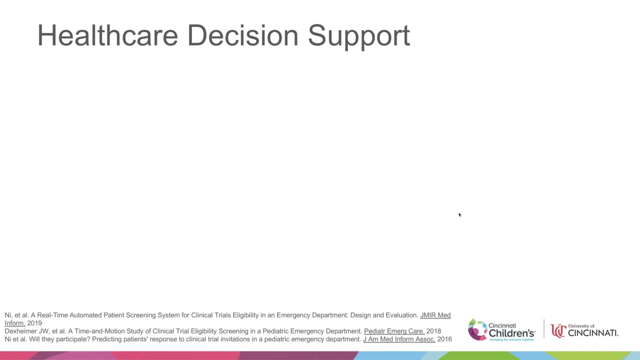 then the last one is more of a future look at precision and predictive medicine and what's going to be coming up so for health care decision support, what's important here is that we made a real-time identification system to screen patients who may be eligible for enrollment in clinical trials during 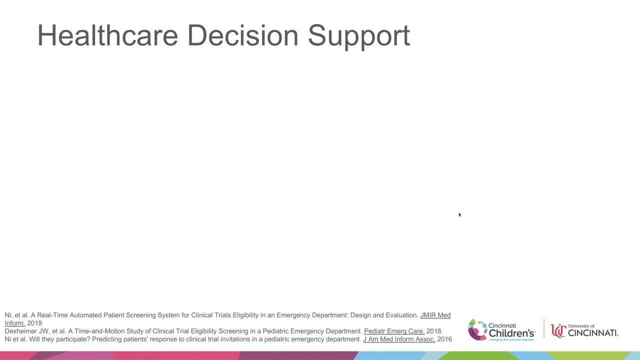 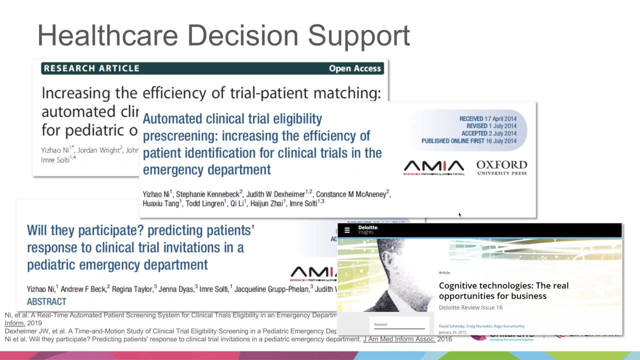 their emergency department visit, and what's really important to know here is that there is a lot of retrospective background and work that goes on prior to something being implemented prospectively. so in our case, starting in about 2014, we started working with end-users and looking at data to design this implementation. that would be helpful for. 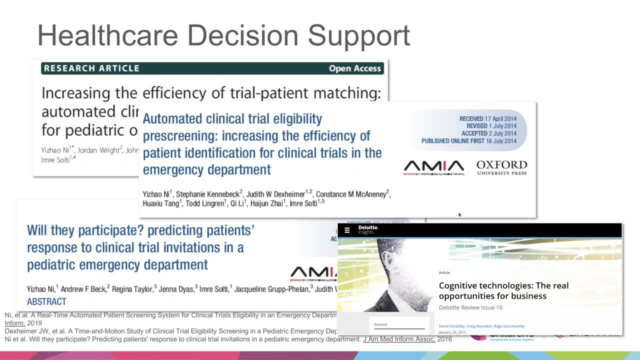 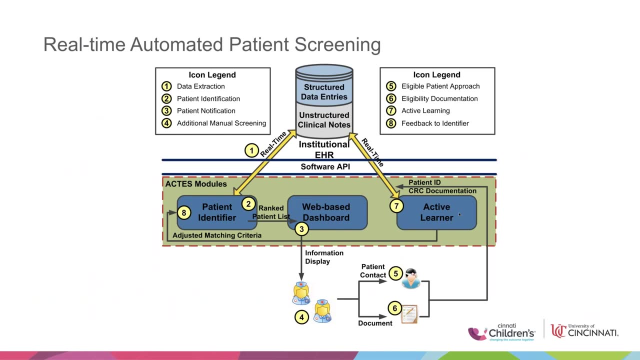 them in the emergency department and our end-users here were primarily clinical research coordinators, who I'm going to call the CRCs. so first let me tell you about the CRCs old work workflow method, then I'll describe our system and then I'll tell you about their new workflow. 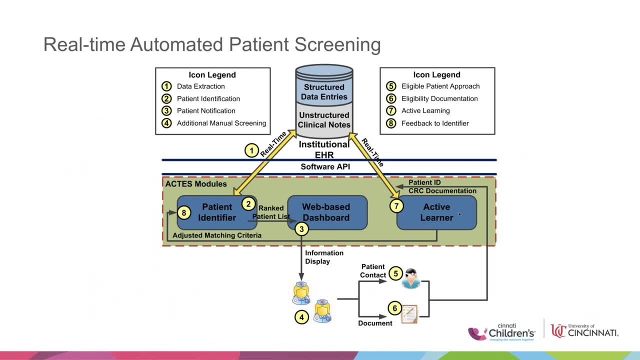 method and let you know whether or not this was effective. So what they did was the clinical research coordinators could sit and look for patients who were coming in check for their structured data, such as their age, their chief complaint, things like that, and then look back. 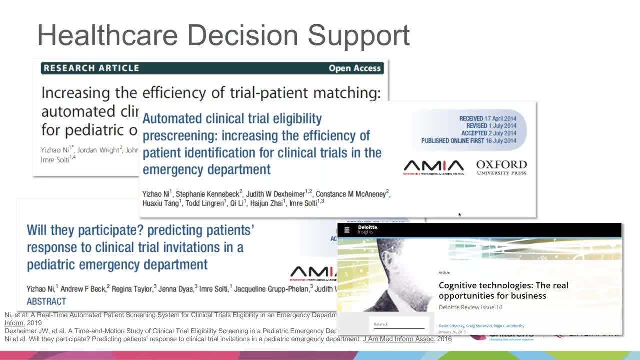 prior to something being implemented prospectively. so in our case, starting in about 2014, we started working with end users and looking at data to design this implementation that would be helpful for them in the emergency department, and our end users here were primarily clinical research coordinators, who i'm going to call the crcs. 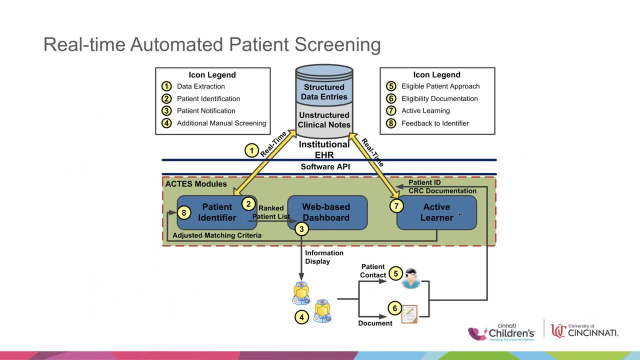 so first let me tell you about the crc's old workflow method, then i'll describe our system, and then i'll tell you about their new workflow method and let you know whether or not this was effective. so what they did was the clinical research coordinators could sit and 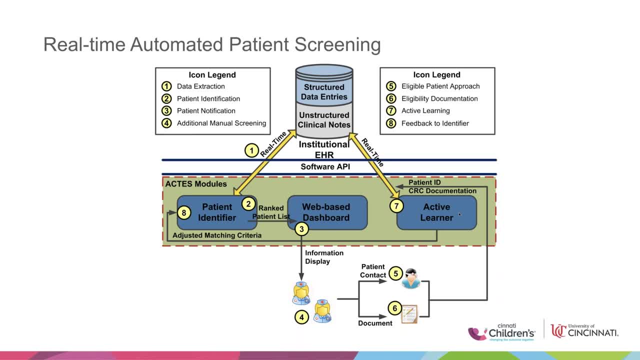 look for patients who were coming in check for their structured data, such as their age, their chief complaints, things like that, and then look back at their list of clinical trials they're currently enrolling, see which ones the patients might want to get it applied to and for what they need to do. 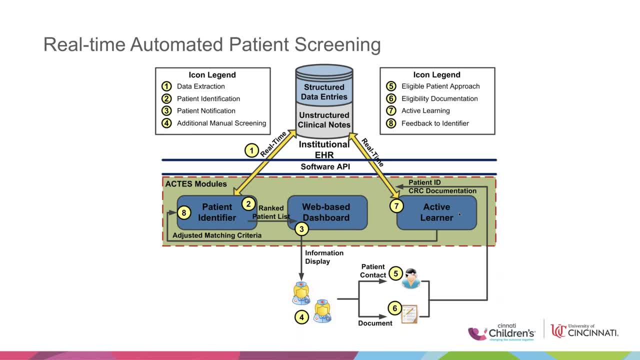 match up with and then do kind of a further dive into their electronic health record before they approach them for enrollment. So what we have here is we developed a real-time natural language processing system with the idea being we can do the structured data for you automatically and we can do some of the 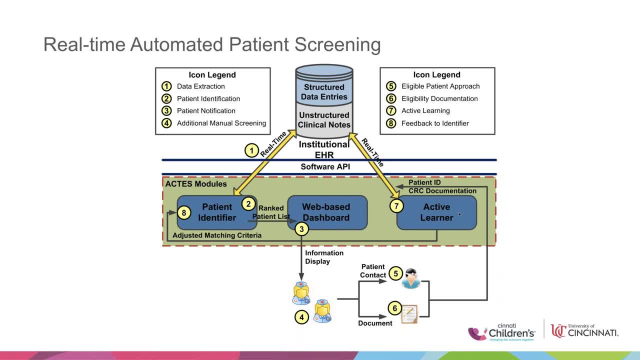 note data as they're filed automatically as well and save you time and hopefully increase clinical trial enrollment and certainly clinical trial screening. So this top part here is our EHR database, the database-looking structure, And so we have structured data entries and we have unstructured clinical notes. 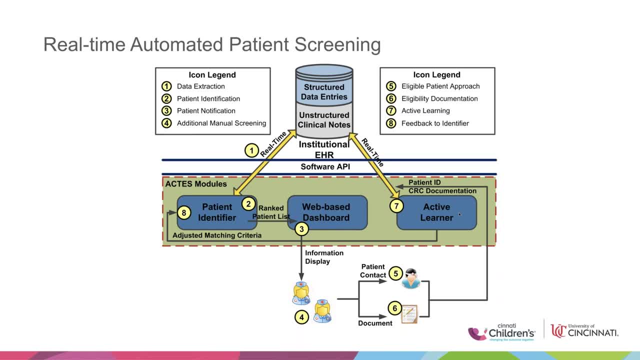 This green part in the middle is the ACTSES module, and it includes all of the NLP, the patient identifier and a web-based dashboard which I'll show you on the next slide for the clinical research coordinator to use. So what happens is we do the same thing. 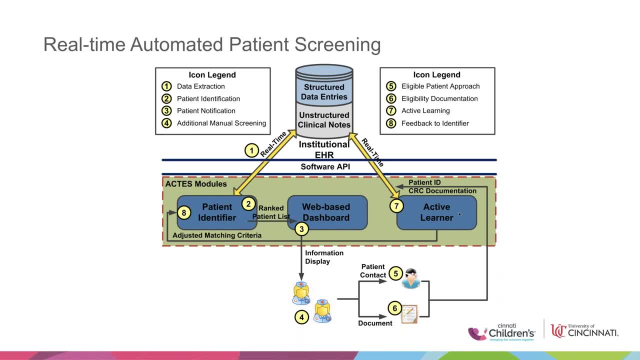 As a patient comes into the emergency department. we identify the patients using the structured data and using unstructured clinical notes as they're filed, Then we display them on this web page for the clinical research coordinators to make a decision about whether or not they should approach them or not. 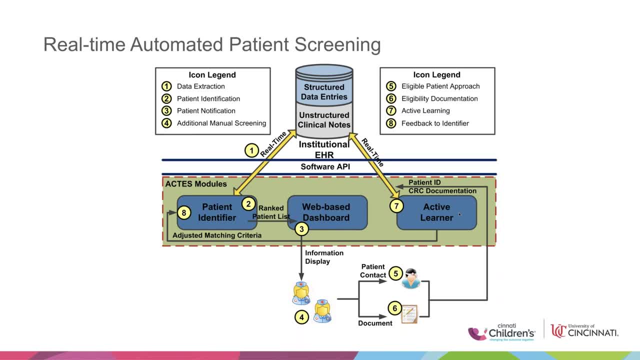 at their list of clinical trials they're currently enrolling, see which ones the patients might match up with and then do kind of a further dive into their electronic health record before they approach them for enrollment. So what we have here is we developed a real-time natural language. 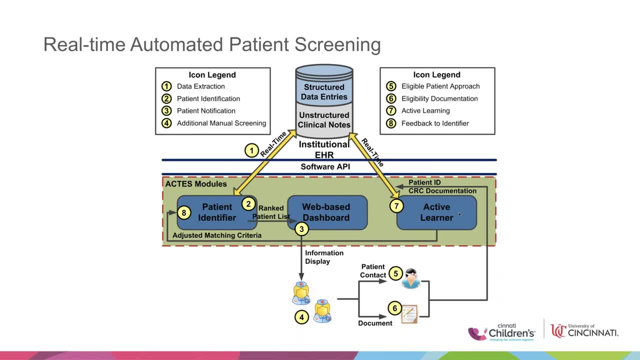 processing system, with the idea being we can do the structured data for you automatically and we can do some of the note data as they're filed automatically as well and save you time and hopefully increase clinical trial enrollment and certainly clinical trial screening. So this top part here is our EHR database, the database-looking structure, And so we have 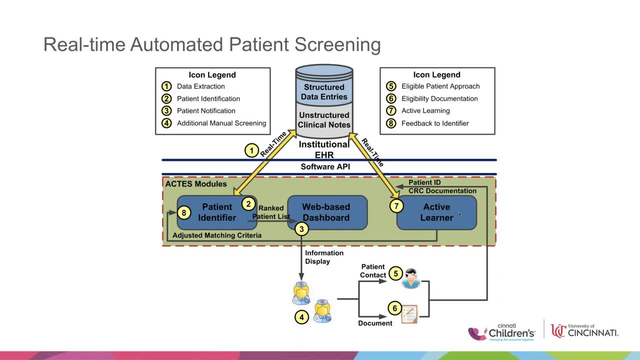 structured data entries and we have unstructured clinical notes. This green part in the middle is the ACTIES module and it includes all of the NLP, the patient identifier and a web-based dashboard, which I'll show you on the next slide, for the clinical research coordinator to use. 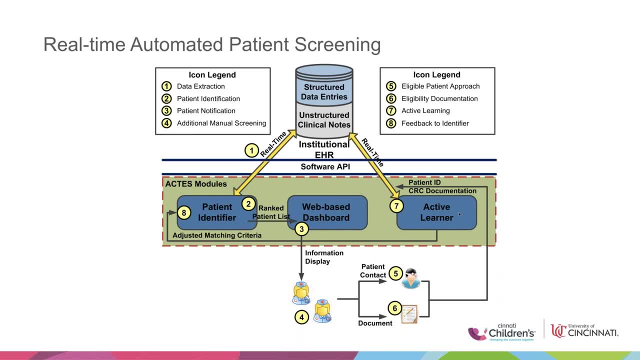 So what happens is we do the same thing. As a patient comes into the NLP, we do the same thing: We send them to the emergency department. We identify the patients using the structured data and using unstructured clinical notes as they're filed, Then we display them on this web page for 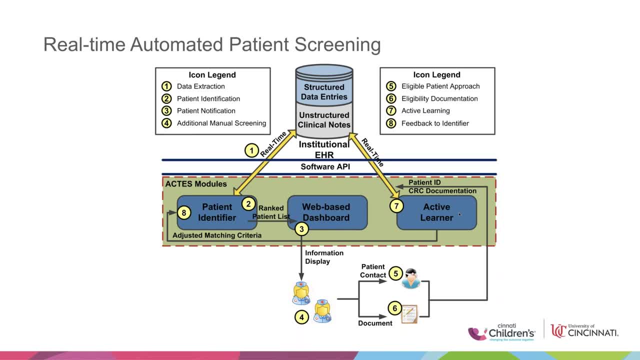 the clinical research coordinators to make a decision about whether or not they should approach them or not. They can annotate the patient's eligibility. They can annotate the screening. Basically, they can aid in communication across all of the different clinical research coordinators. 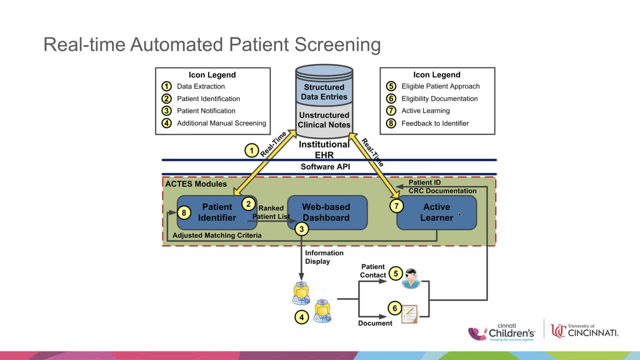 And then ultimately, whether or not they decide to approach the patient. they can annotate the patient's eligibility. They can then document whether or not the patient was enrolled or if the patient was not eligible at all for this study, in which case all of these data come back into the NLP. 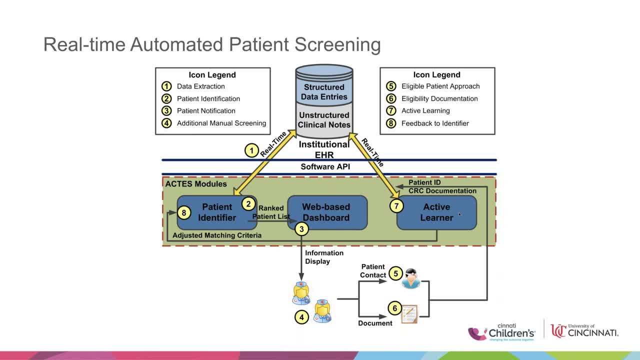 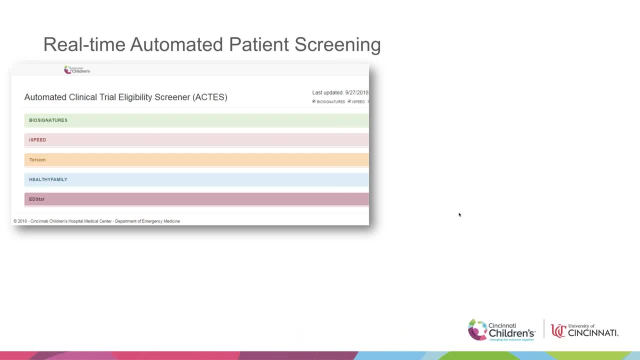 and it performs active learning and we improve our recommendations for next time. So here's what their website looks like. What you see here is it's color-coded for the five clinical trials currently being enrolled in our emergency department. What you also see is at the top right of that box is the time it was last updated. 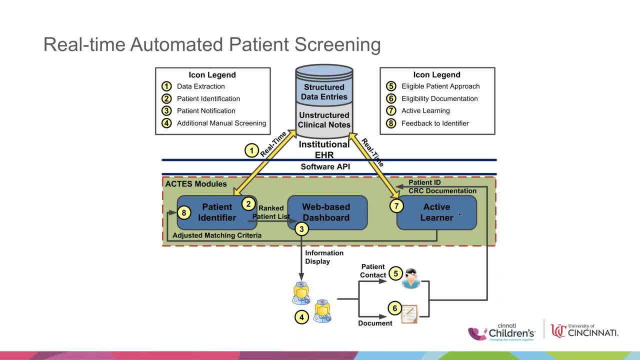 They can annotate the patient's eligibility. They can annotate the screening. Basically, they can aid in communication across all of the different clinical research coordinators And then ultimately, whether or not they're eligible for the EHR. they can annotate the screening. 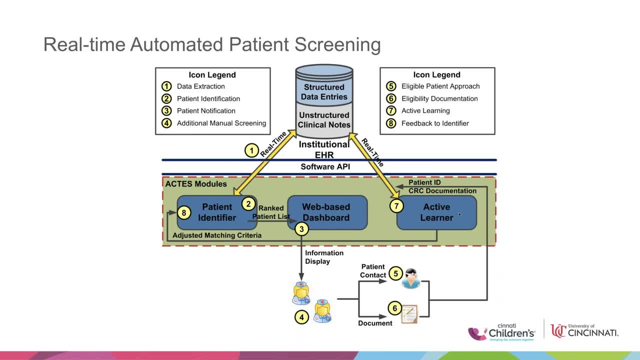 Basically, they can aid in communication across all of the different clinical research coordinators And then, ultimately, whether or not they decide to approach the patient. they can then document whether or not the patient was enrolled or if the patient was not eligible at all for this study, in which case all of these data come back into the NLP and it performs. 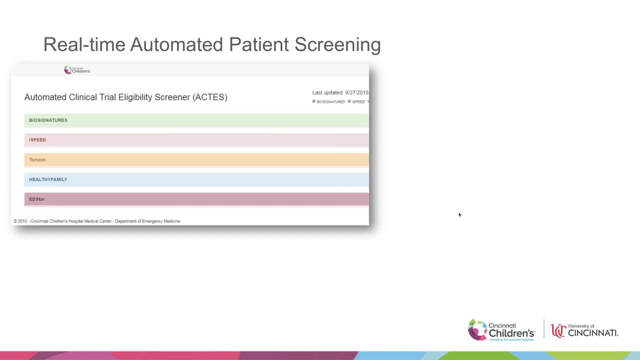 active learning and we improve our recommendations for next time. So here's what their website looks like. What you see here is it's color coded for the five clinical trials currently being enrolled in our emergency department. What you also see is at the top right of that box is the time it was last updated. 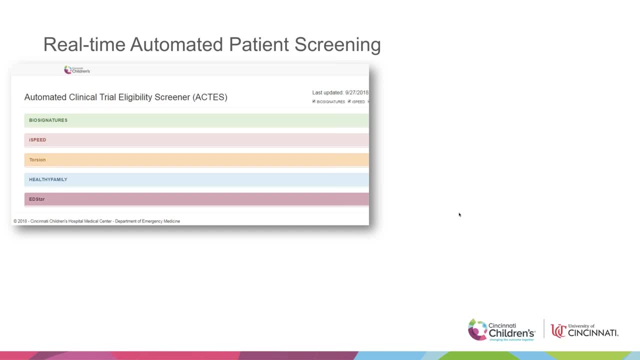 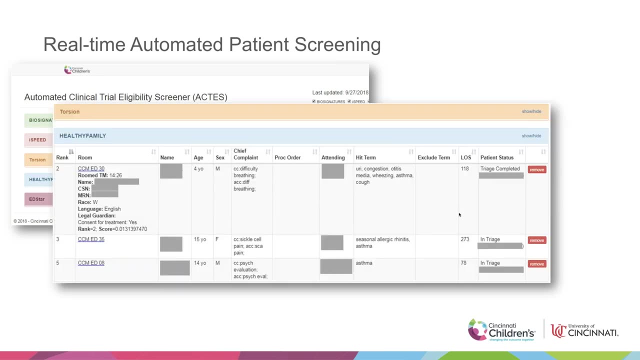 So it's updated approximately every 15 minutes and all new notes that have been filed since then are included in the processing and the new recommendations are made. So when a clinical trial associate wants to look at, say in this case, the healthy family, 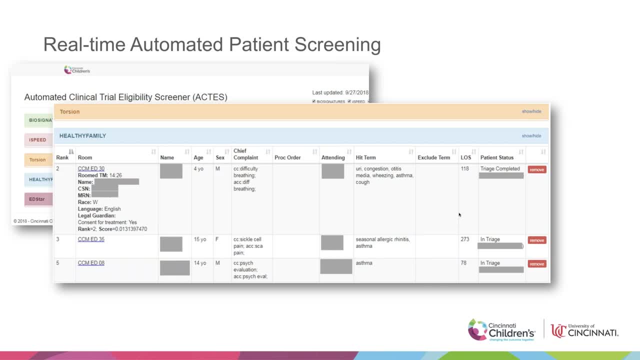 study. this is what they get. They say: here is the top ranked patient. Their rank is number two. Here's what room they're in. Here's their name, their age, their gender, their chief complaint. Here's their attending, in case you, the clinical research coordinator, need to approach them. 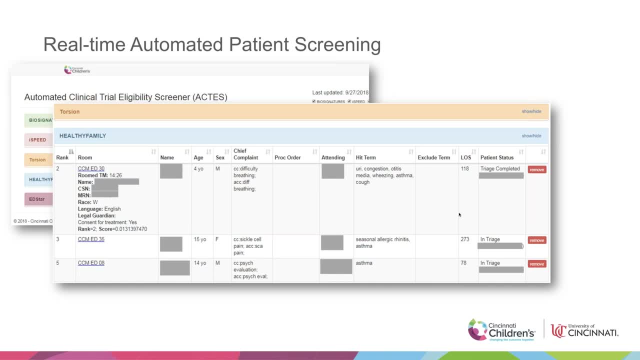 Here's why we think they're a great match for this study. That's what the HIT term is. Here's their length of stay in the emergency department. So you can kind of decide: perhaps they're going to be going home soon, Maybe they just got here and they need some time to make sure nothing else happens. 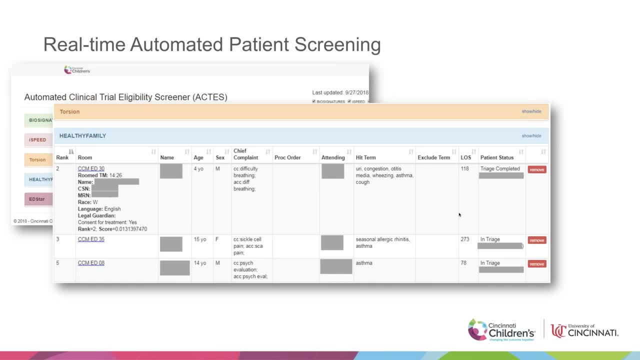 And then here's their official patient status from the EHR. So if the clinical research coordinator says yes, but this patient doesn't match and we don't want anybody else screening them again, they can click that little remove button. And what the remove button lets them do is say this patient's eligible, therefore I. 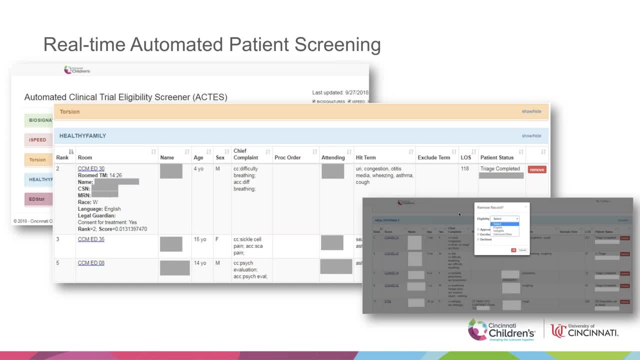 enrolled them And so they don't need to be on this list anymore because we don't need anyone else to talk to them. This patient's not eligible. I approached them but they declined, et cetera. So what this does for them is it lets them have aided communication. 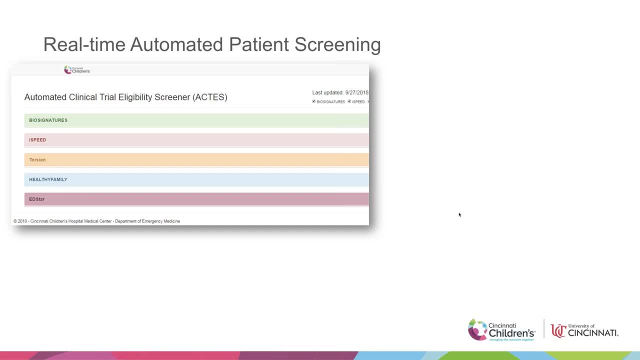 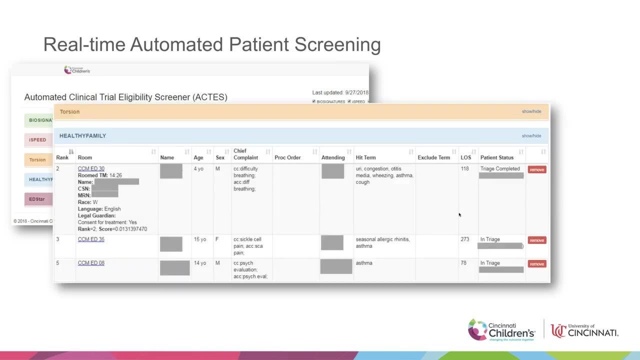 So it's updated approximately every 15 minutes and all new notes that have been filed since then are included in the processing and the new recommendations are made. So when a clinical trial associate wants to look at, say in this case, the healthy family study. 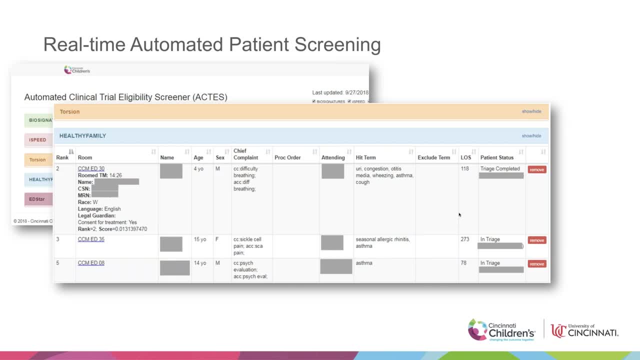 this is what they get. They say: here is the top ranked patient, Their rank is number two. Here's what room they're in. Here's their name, their age, Their gender, their chief complaint. Here's their attending, in case you. 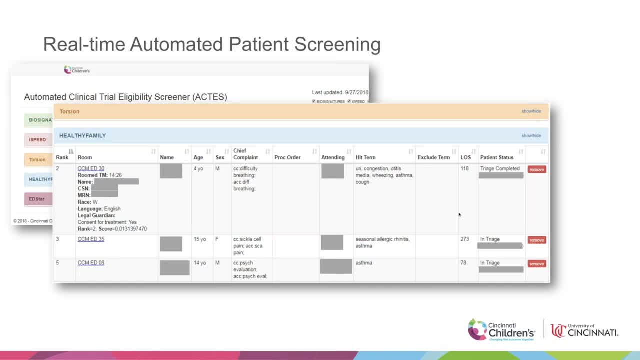 the clinical research coordinator need to approach them. Here's why we think they're a great match for this study. That's what the HIT term is. Here's their length of stay in the emergency department, So you can kind of decide Perhaps. 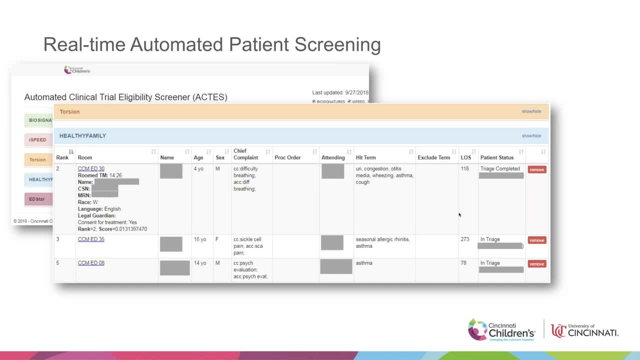 they're going to be going home soon. Maybe they just got here and they need some time to make sure nothing else happens. And then here's their official patient status from the EHR. So if the clinical research coordinator says, yes, but this patient doesn't match and we don't want anybody else screening them again, 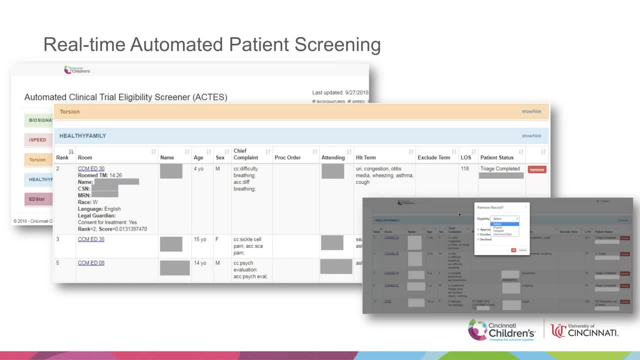 they can click that little remove button, And what the remove button lets them do is say: this patient's eligible, therefore I enrolled them And so they don't need to be on this list anymore, because we don't need anyone else to talk to them. This patient's not eligible. 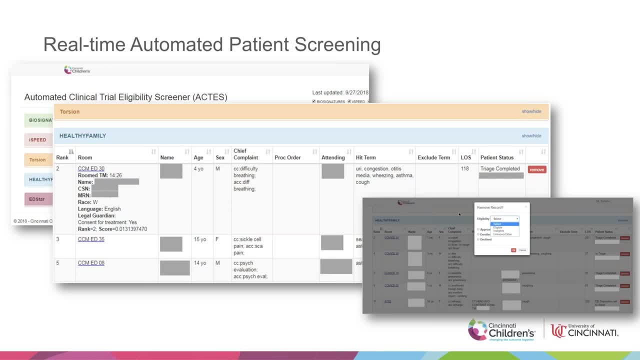 I approached them but they declined, et cetera. So what this does for them is it lets them have aided communication, It lets them spend less time going into the EHR and basically gives them a different place to view patients and see how they're doing. So the question is: did it work? 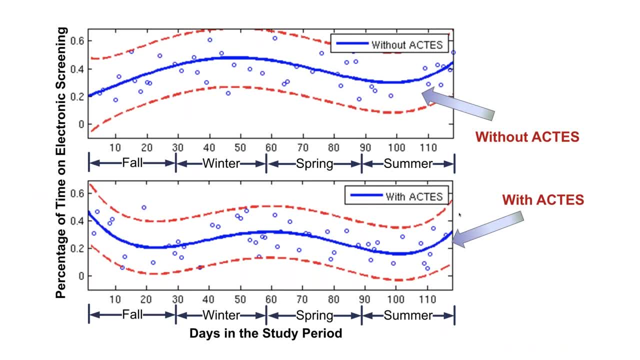 And the answer is yes, And so what we have here is that the top bar is without the system in place over a full year and the bottom bar is with it in place, And what happened was that we had a 30 percent reduction in screening time. 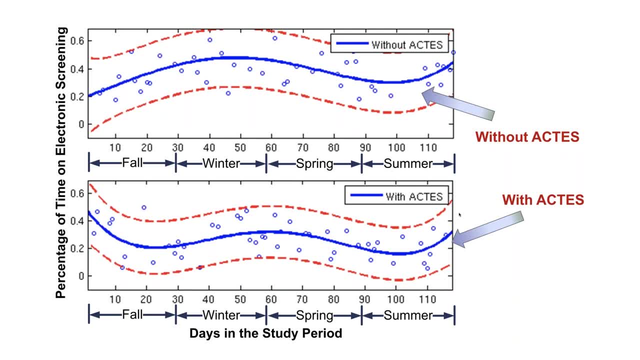 even when adjusting for the seasonal variation that comes with being in emergency medicine and patient visits. so this is great, and so what this means for us is that we continue can continue to expand it and add more studies, but it also means it'll help aid us in planning. 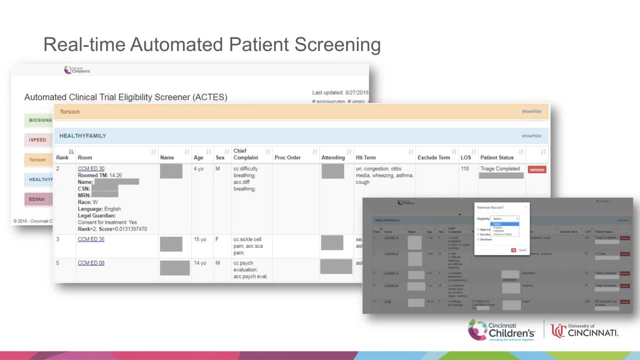 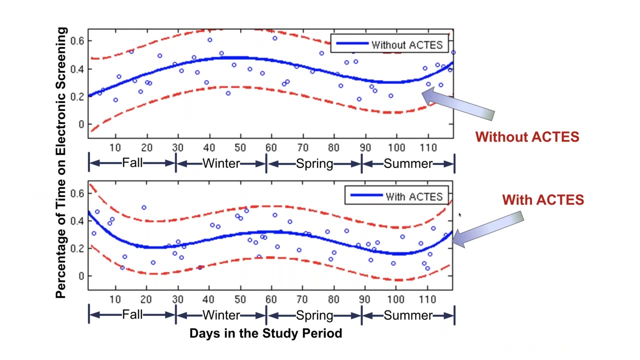 It lets them spend less time going into the EHR and basically gives them a different place to view patients and see how they're doing. So the question is: did it work? And the answer is yes, And so what we have here is that the top bar is, without the ACTI system in place, over a 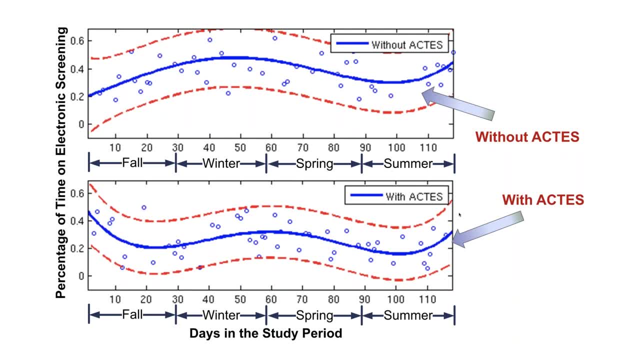 full year and the bottom bar is, with it, in place, And what happened was that we had a 30% reduction in screening time, even when adjusting for the seasonal variation. So this is something that comes with being in emergency medicine and patient visits. 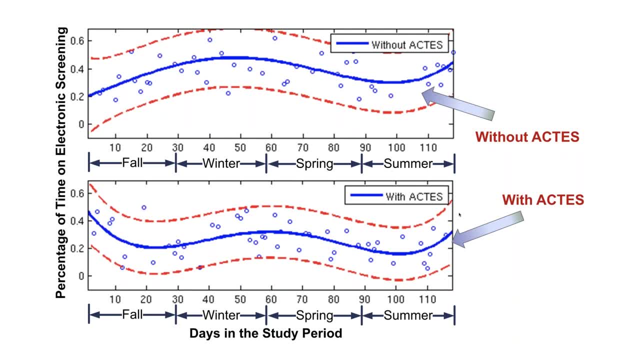 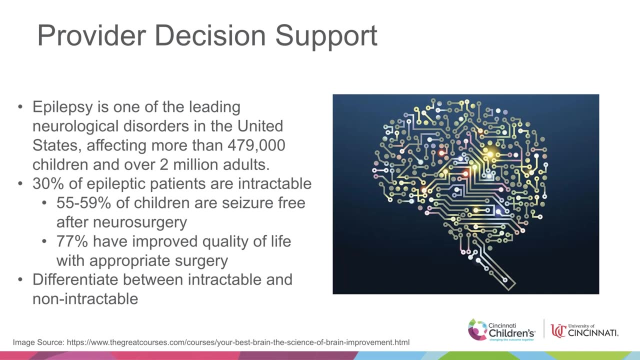 So this is great, And so what this means for us is that we can continue to expand it and add more studies, But it also means it'll help aid us in planning future research studies, finding patients who might be eligible and future staffing. So let's talk about something that's provider decision support. 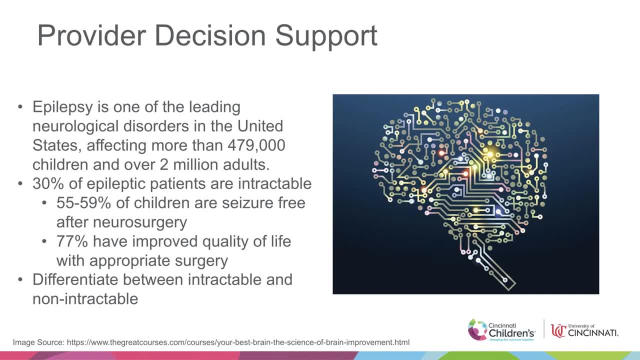 I'm going to do a brief background here for you on epilepsy. So epilepsy is one of the leading neurological disorders. in 크리스 유어� attack It's a disease that's seen in a number of patients with chronic stroke and long-term 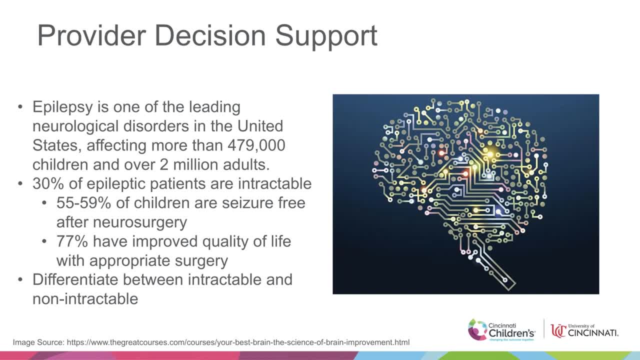 pain united states, and it affects more than 480 000 children and over 2 million adults. 30 of patients with epilepsy are intractable, and intractable epilepsy means that you have drug resistant epilepsy, so in other words, the medications don't control your seizures. and so of these who are 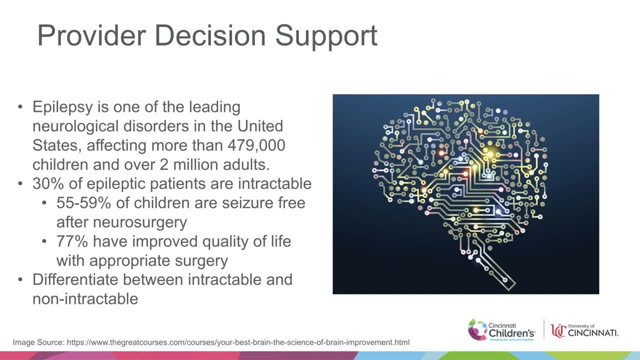 intractable. 55 to 60 percent of the children are eligible for neurosurgical evaluation and treatment and they're seizure-free after they've had appropriate neurosurgery. and of those, 77 have an improved quality of life with appropriate surgery. currently, the average here at cincinnati: 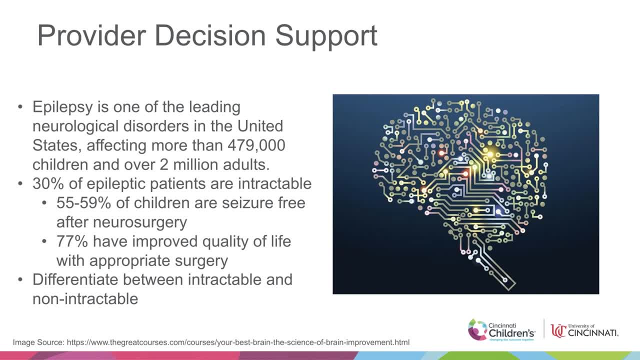 children's from diagnosis to surgery. identification is about six years. our goal with the pestian lab was to develop and create a system that would be able to treat children with epilepsy in a way that would be similar to the one we developed for petiveral epilepsy. the mission is that we would 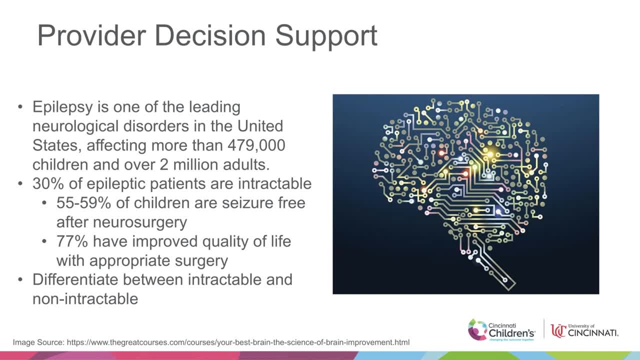 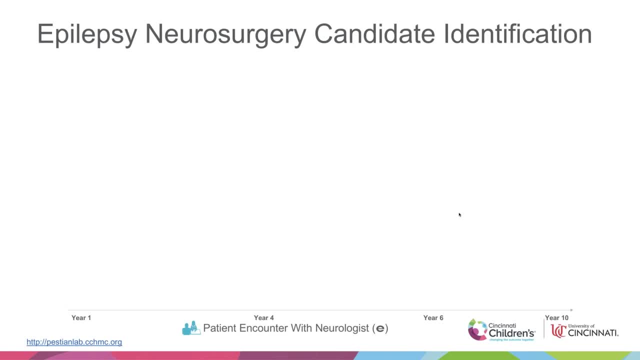 be able to treat children with epilepsy without the need or without the need of it, but that it would be between intractable and non-treatable seizures in children. so here's the way this one works. you can see on the bottom we have the patient identified. 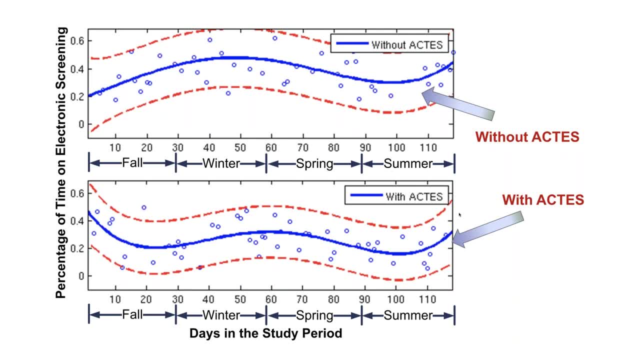 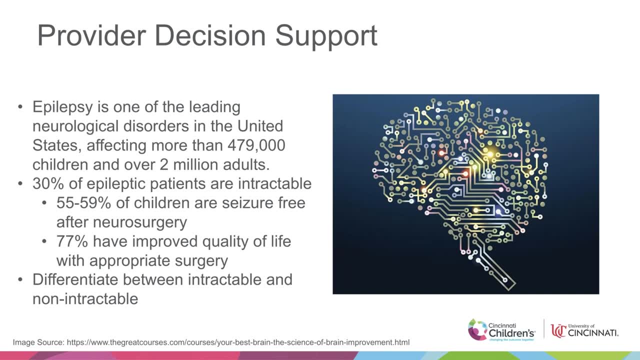 future research studies finding patients who might be eligible and future staffing. so let's talk about something that's provider decision support. i'm going to do a brief background here for you on epilepsy. so epilepsy is one of the leading neurological disorders in the united states and it affects more than 480 000 children and over 2. 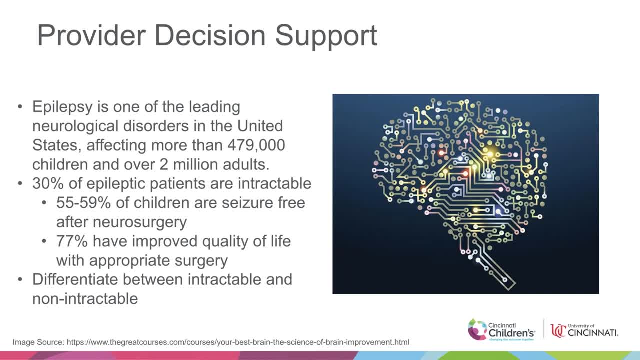 million adults, 30 of patients with epilepsy are intractable. and intractable epilepsy means that you have drug resistant epilepsy, so, in other words, the medications don't control your seizures. and so of these who are intractable, 55 to 60 percent of the children. 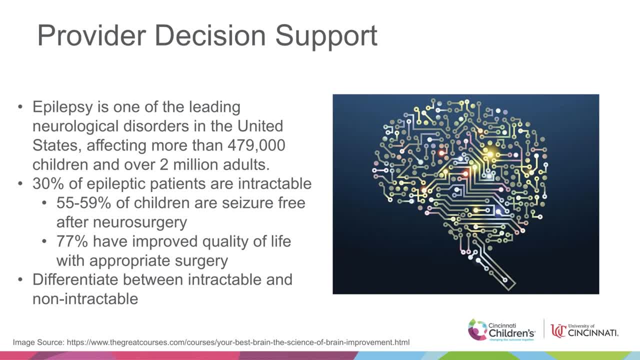 are eligible for neurosurgery and they're seizure-free after they've had appropriate neurosurgery and of those, 77 percent have an improved quality of life with appropriate surgery. currently the average here at cincinnati children's from diagnosis to surgery identification is about six years. our goal with the pestian lab was to develop and create a 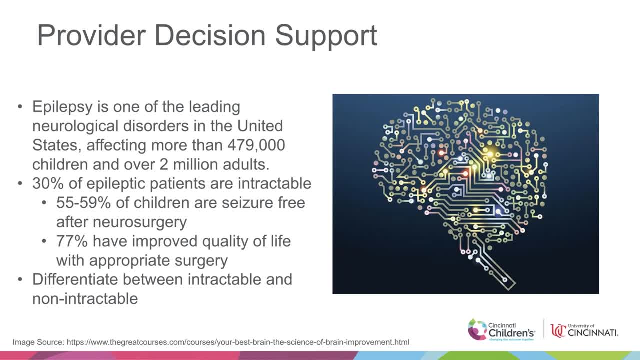 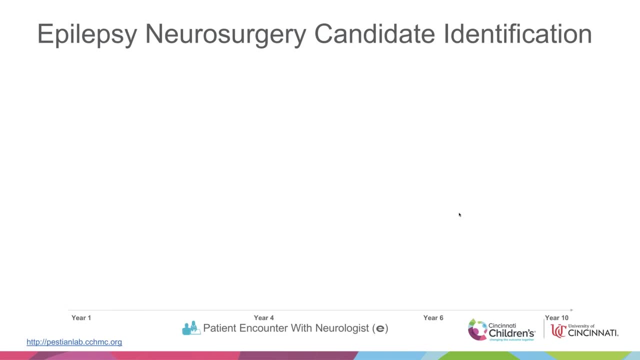 natural language processing algorithm that used the clinician notes to differentiate between intractable and intractable epilepsy, and we're going to talk a little bit more about that in the next few minutes, so let's get started. so here's the way this one works. you can see on the bottom. we have the patient identified at year. 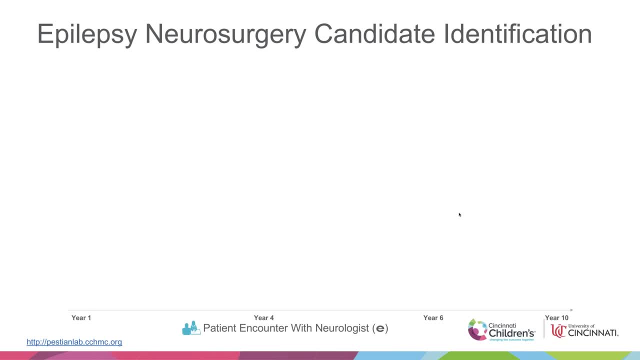 one. this was their date of diagnosis, and then year to 10, we can pretend this is how they are today. so what we have here in the top is the neurologist language of intractable seizures as they write their notes. what we have here at the bottom is the neurologist 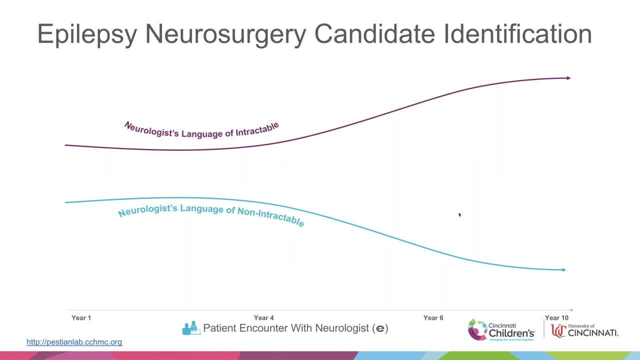 language of non-intractable seizures as they write their notes- and these are just general trends for the way they write their notes- Each of these little E's represents a patient visit with their neurologist, So you can see that as they go through their care, they're moving towards. 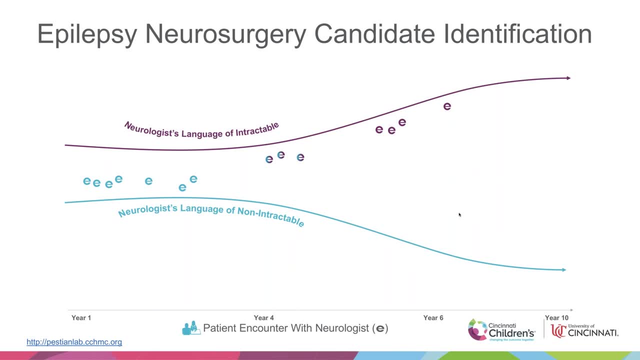 non-intractable. No, this patient is moving towards intractable. So what happens in the previous visits prior to implementation of our natural language processing algorithm? patients can be identified at year six And we say: look, you're intractable. You may need to be. 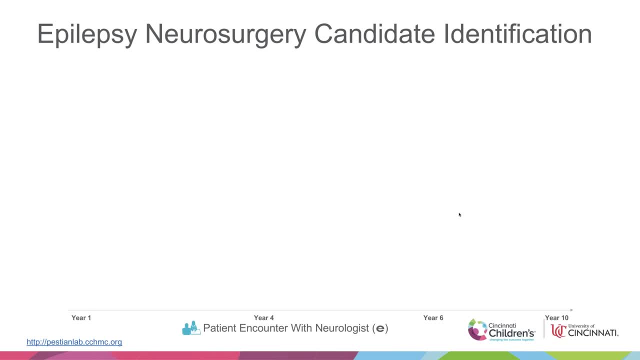 at year one. this was their date of diagnosis- and then year two ten. we can pretend this is how they are today. so what we have here in the top is the neurologist language of intractable seizures as they write their notes. what we have here at the bottom is the right-hand side of the 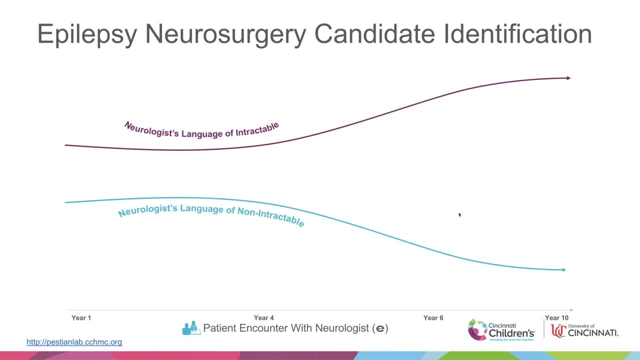 table. it's a four- BP tube at the right hand side which is the speech point and i'm going to show you is the neurologist language of non-intractable seizures. as they write their notes. And these are just general trends for the way they write their notes. 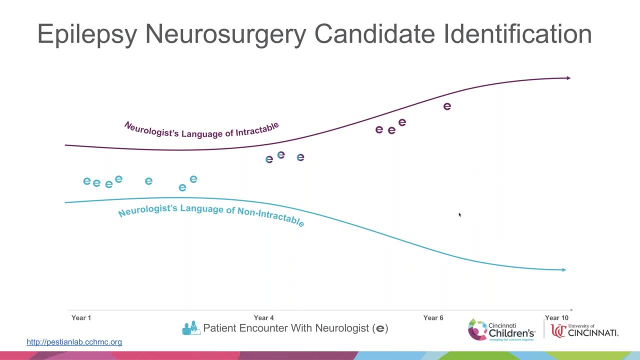 Each of these little Es represents a patient visit with their neurologist. So you can see that as they go through their care, they're moving towards non-intractable. No, this patient is moving towards intractable. So what happens in the previous visits? 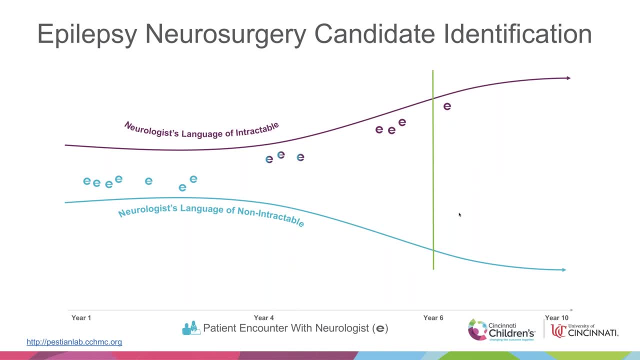 prior to implementation of our natural language processing algorithm. patients can be identified at year six And we say: look, you're intractable, You may need to be sent for surgery consult. Let's go ahead and send you Instead with the algorithm and alerting the providers. 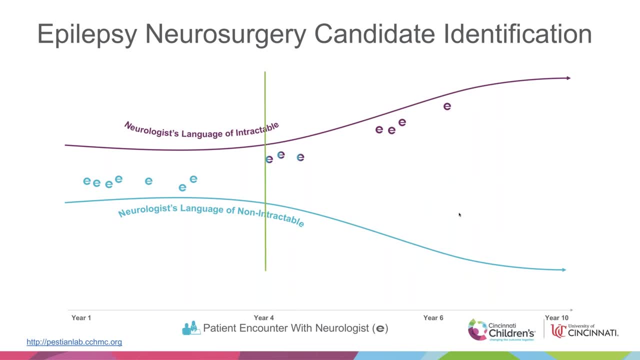 we can recommend and find patients at year four, So up to two years earlier than they're being found in typical clinical care, And so what we wanted to do with this was then implement it into clinical care. So here I'm gonna give you a brief description. 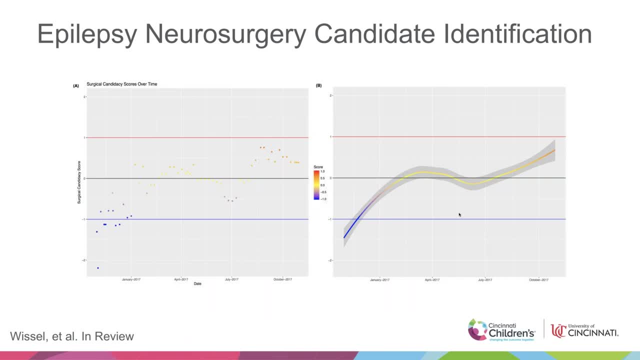 of like our real time implementation. So what we did is, every Sunday we ran through all patients that we knew who had epilepsy, who visited our clinics, And we looked for patients with an upcoming visit that Sunday, that week. We did it all on Sunday so that when we sent an alert, 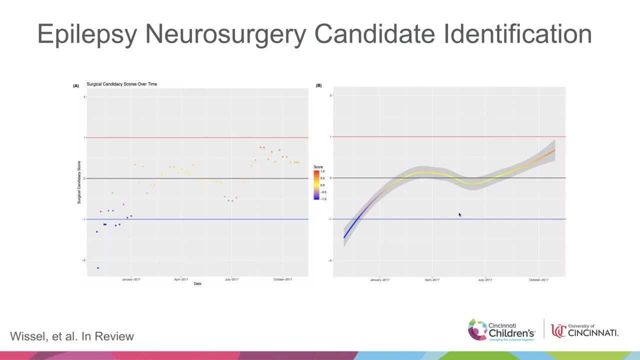 to providers. they had plenty of time before their patient visit to read through the chart, to look at things And to think about the recommendation we might be giving to them. So what we did is we evaluated all of the upcoming visits And then we assigned a score. 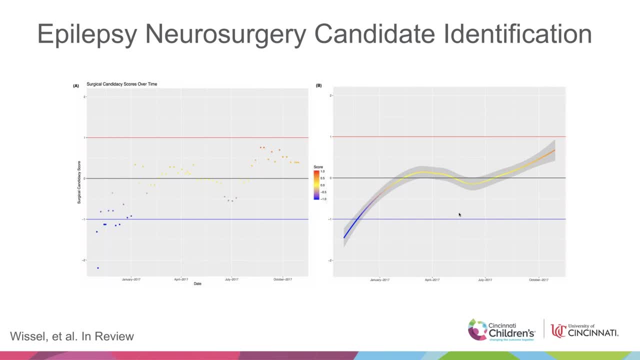 And in this case, on this page, the scores go from about negative two to two. This is one set of patient scores from January 2017 to October 2017.. And you can see that, as this patient gets a new score every week, they appear to be moving towards being intractable. 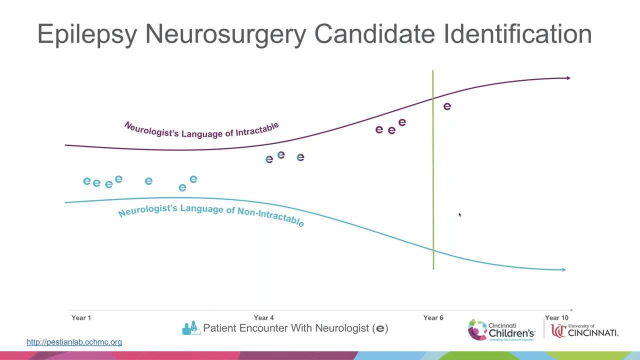 sent for surgery consult, Let's go ahead and send you Instead. with the algorithm and alerting the providers, we can recommend and find patients at year four, so up to two years earlier than they're being found in typical clinical care, And so what we wanted to do with this was then implement it. 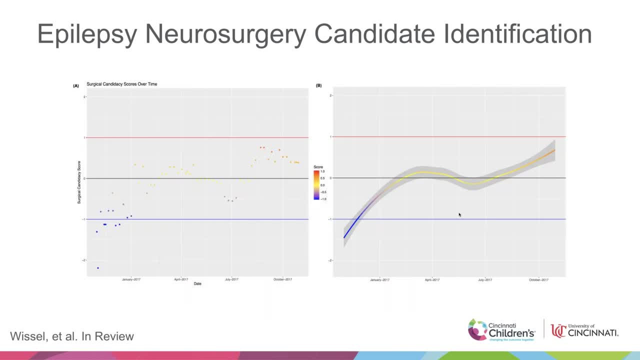 into clinical care. So here I'm going to give you a brief description of what we're doing. So what we did is, every Sunday we ran through all patients that we knew who had epilepsy, who visited our clinics, and we looked for patients with an upcoming visit that Sunday. 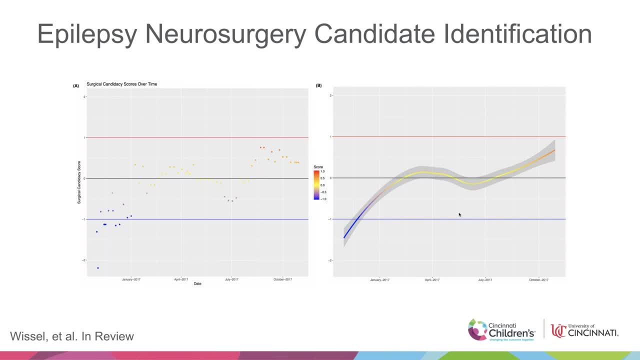 that week. We did it all on Sunday so that when we sent an alert to providers, they had plenty of time before their patient visit to read through the chart, to look at things and to think about the recommendation we might be giving to them. So what we did was we sent. 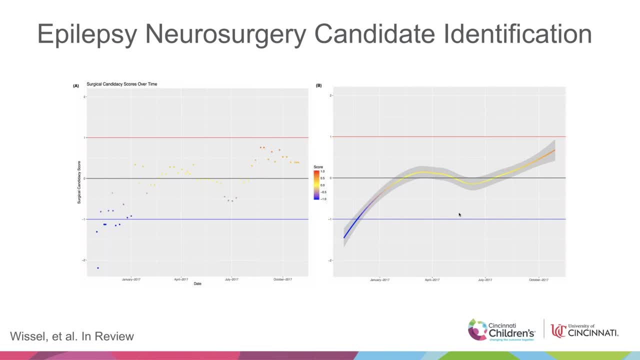 an alert to the providers. We sent an alert to the providers. We sent an alert to the providers. So what we did is we evaluated all of the upcoming visits and then we assigned a score, And in this case, on this page, the scores go from about negative two to two. 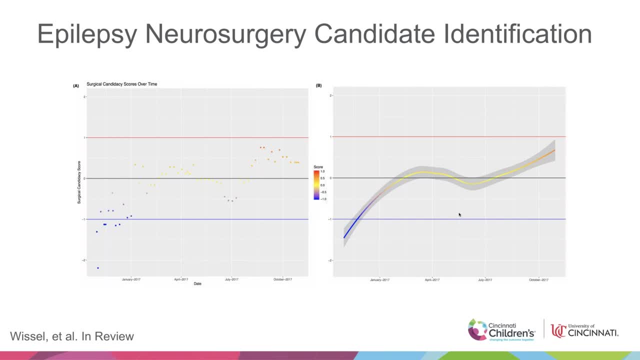 This is one set of patient scores from January 2017 to October 2017.. And you can see that, as this patient gets a new score every week, they appear to be moving towards being intractable, And so what we wanted to do was we set a cutoff on our algorithm to 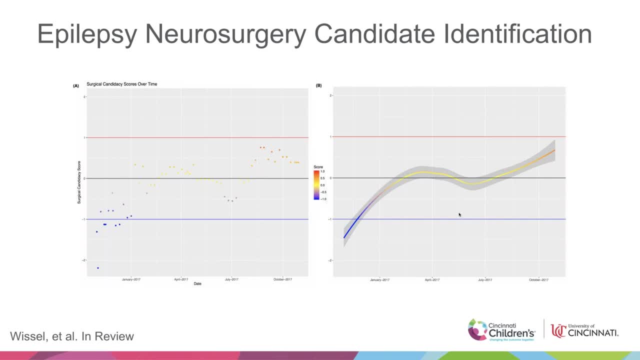 maximize the performance that we had. and then we sent a reminder to the provider with information And it said: you know what your patient may be eligible for neurosurgical evaluation. You know you should think about going ahead and sending them. 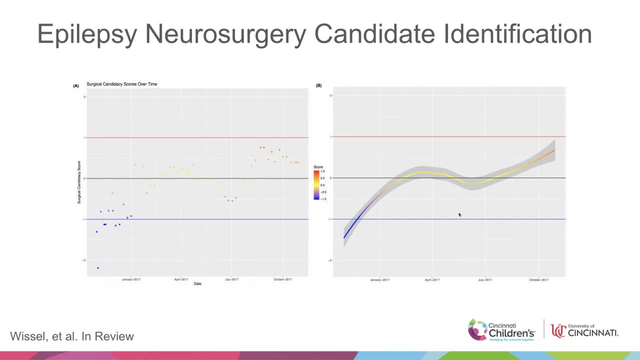 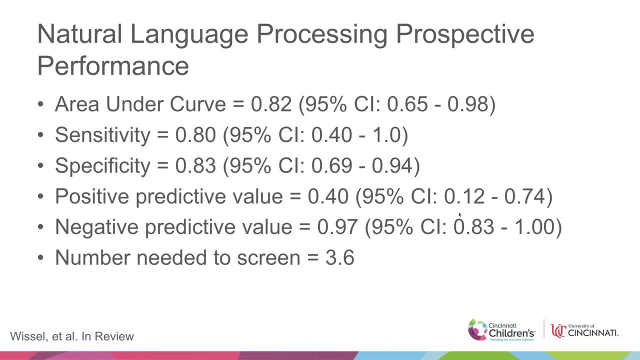 Providers received about one to two total alerts a week and that's about it. So we looked at our area under the curve because we developed everything retrospectively with the neurologist and then we wanted to evaluate it prospectively And we did a good job. We have 82% for area under the curve. Our positive predictive value is low. 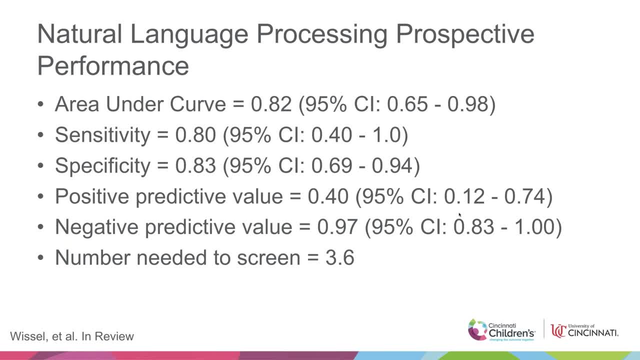 It's only 40%. Our negative predictive value is very high at 97%. What that means is that we're probably not missing anybody And our number needed to screen is 3.6 patients, And that means that we need to look at four patients to find 3.6 patients to find one who is going to be eligible to be sent to the program. 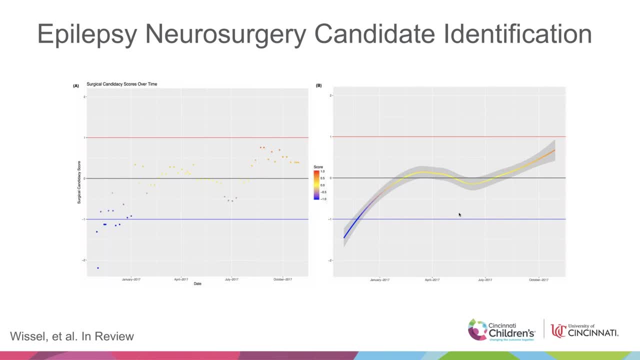 And so what we wanted to do was we set a cut off on our algorithm to maximize the performance that we had, And then we send a reminder to the provider with information And it said: you know what your patient may be eligible for neurosurgical evaluation. 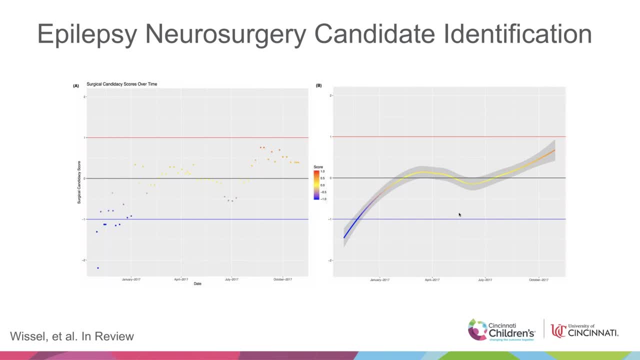 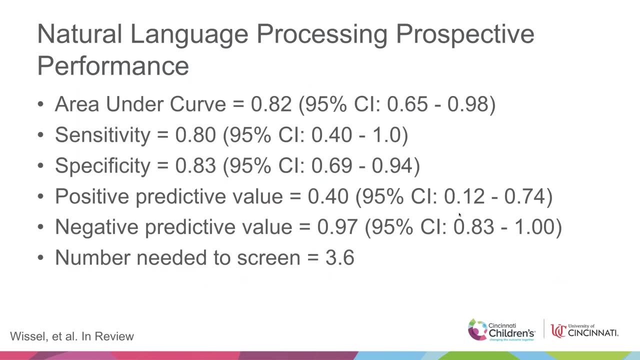 You know you should think about going ahead and sending them. Providers received about one to two total alerts a week And that's about it. So we looked at our area under the curve because we developed everything retrospectively with it. So we looked at our area under the curve because we developed everything retrospectively with it. 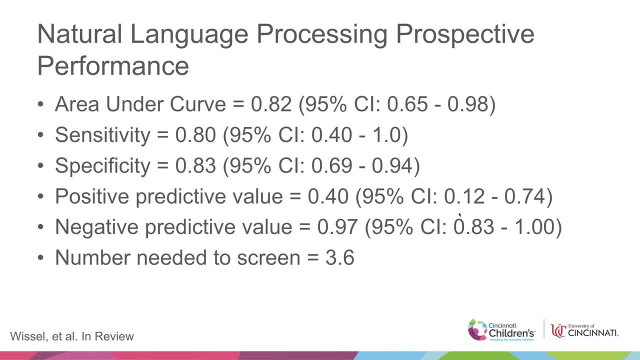 the neurologist, and then we wanted to evaluate it prospectively and we did a good job. we have 82 for area under the curve. our positive predictive value is low. it's only 40. our negative predictive value is very high at 97. what that means is that we're probably not missing anybody. 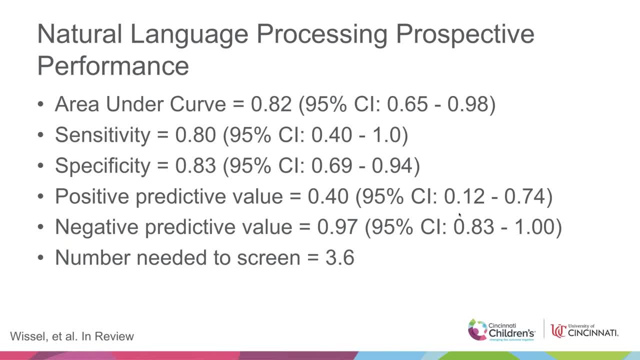 and our number needed to screen is 3.6 patients and that means that we need to look at four patients to find 3.6 patients, to find one who is going to be eligible to be sent to surgery consult and ensure that they can be sent. so we did that. we prospectively evaluated 200. 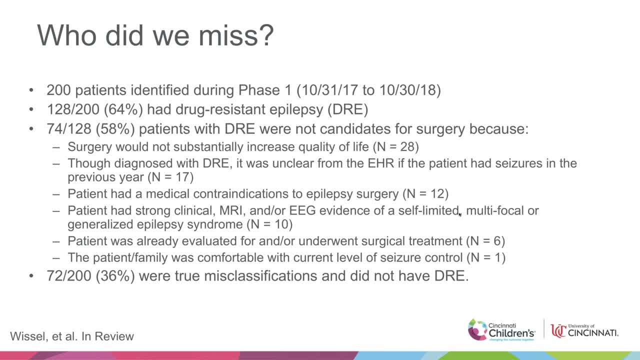 different patients that we identified from october 2017 to october 2018, and we had two epileptologists look at every single patient and say, yes, they should be sent based on just their clinical data, or no, they're not really going to be surgery candidates. 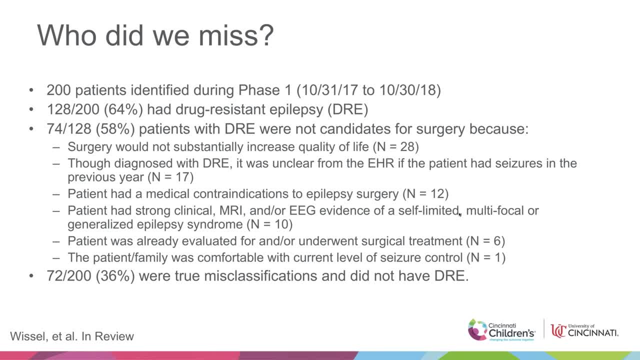 so of the 200 patients, 64 of them had drug resistant epilepsy and were eligible for surgical evaluation. of the 128 that were identified, about 58 percent were likely not going to be sent to surgery ever. for there's a right- a range of reasons listed below, but 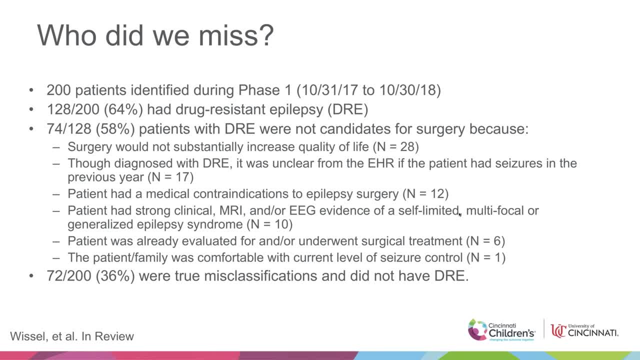 including the surgery probably would not substantially increase their quality of life. one six patients had already been evaluated for and had undergone surgical treatment, but they were still having seizures. and of course then things like social issues, where the patient and family were comfortable with the current level of seizure control and were interested in sending their child. 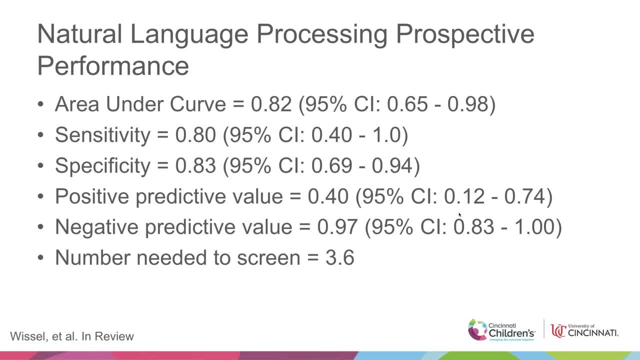 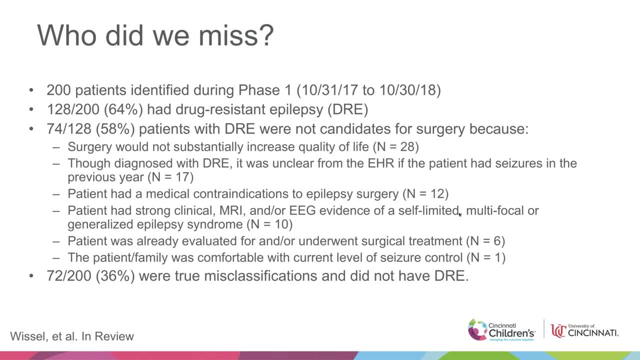 And we're really worried about that, because a lot of times we get uh, um, we get a mean number for patients and we're Didn't even know that we'd be able to actually get that number by 1,000, uh cases, Uh, so we decided to go ahead and make sure that we 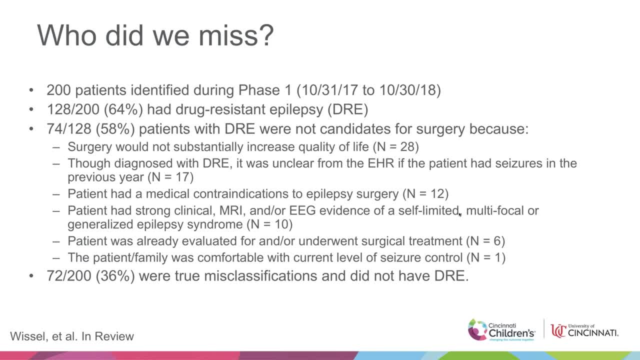 had that number in our catalog because we've been monitoring all these disease response indicators about how we can potentially provide people with those numbers and how we can provide those numbers to theygots. So we had a 2% number for patients who were already eligible to be sent. 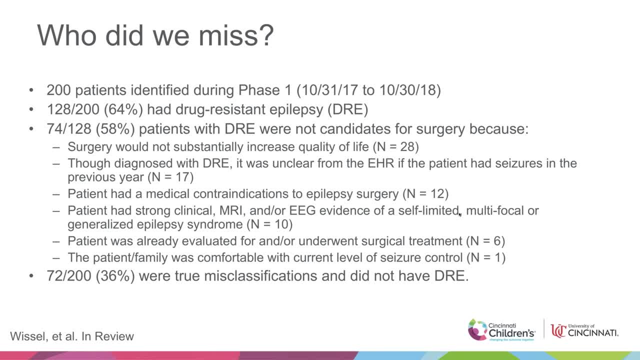 and we had a 1% number for those patients who were still eligible to be sent. So we had a 2% number. epilepsy and were eligible for surgical evaluation. Of the 128 that were identified, about 58% were likely not going to be sent to surgery ever, for there's a wider range of 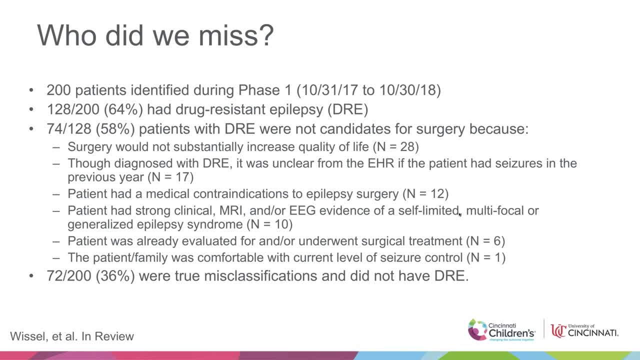 reasons listed below, but including the surgery probably would not substantially increase their quality of life. One: six patients had already been evaluated for and had undergone surgical treatment, but they were still having seizures. And of course then things like social issues, where the patient and family were comfortable with the current level of seizure control, and 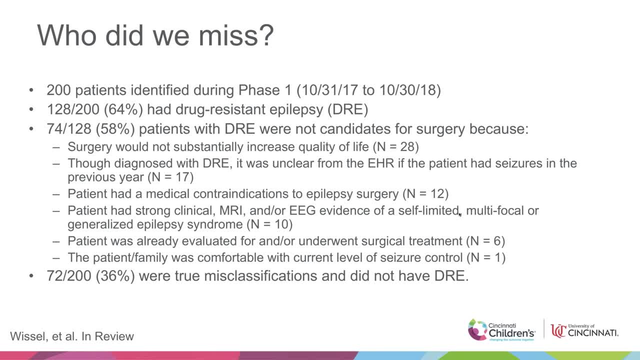 were interested in sending their child for surgical evaluation. 36%, and that's all, were true misclassifications and didn't have drug-resistant epilepsy. So this allowed the providers to make a better decision. When they saw their patient, they had this additional information and they could say: well, here's. 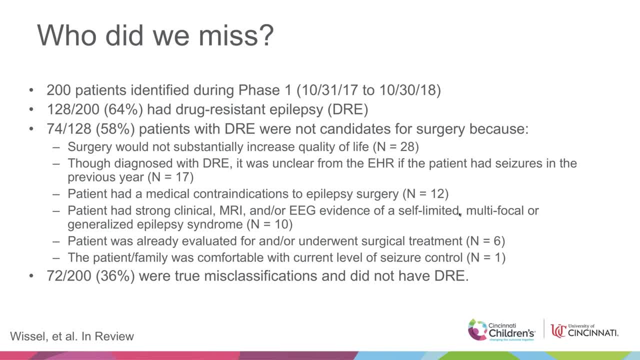 one of the decline reasons. This is why we don't think this patient's eligible. Or they could say: you know what, go ahead and send on. So we've improved surgery detection by about 43%, And so decision support is great and it's very important. But what about things that are more? 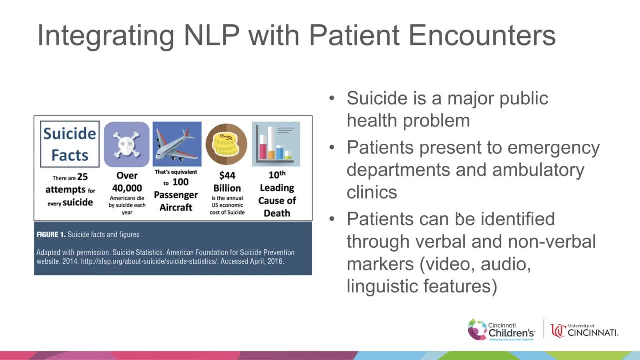 directly patient-facing, Like: how do we include the patients in their own care? And so here's a brief background on suicide, which is suicide is a major public health problem. Patients with a suicide attempt have you know, they've been diagnosed with a suicide attempt and they've 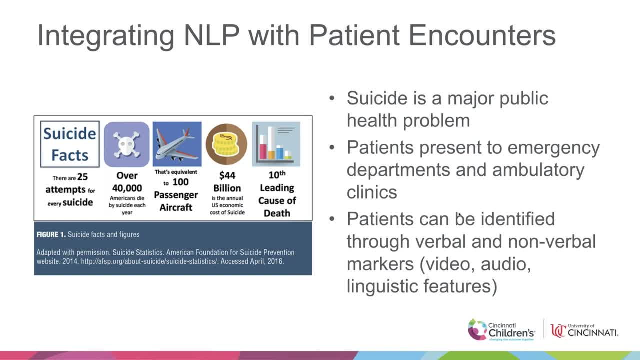 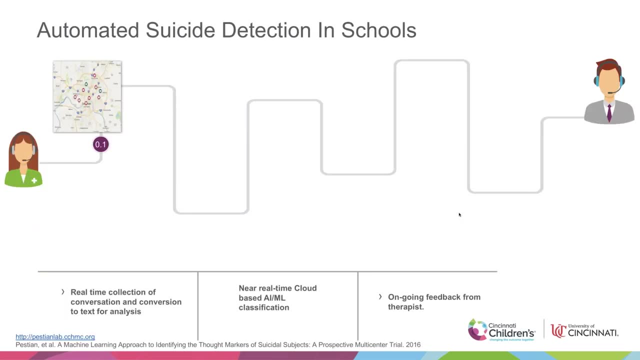 frequently presented to the emergency department or an ambulatory clinic up to two weeks prior to their attempt, And these patients can be identified through verbal and nonverbal markers, including video, audio and linguistic features. What I have here on this slide to show you is an application. 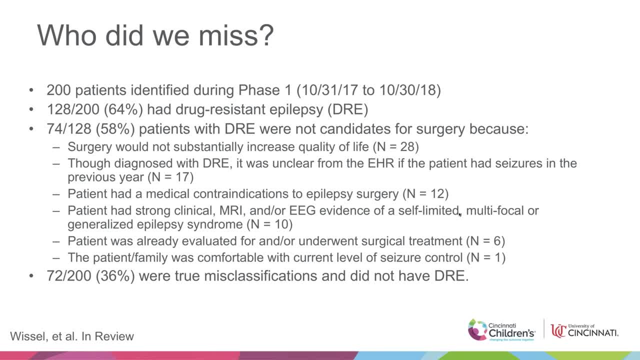 for surgical evaluation. 36 and that's all were true misclassifications and didn't have drug resistant epilepsy. so this allowed the providers to make a better decision. when they saw their patient, they had this additional information and they could say: well, here's one of the decline reasons. 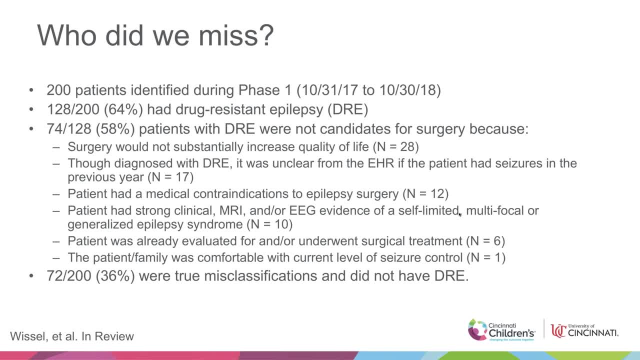 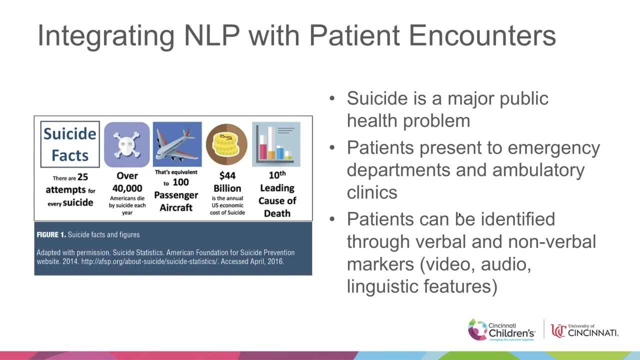 this is why we don't think this patient's eligible, or they could say: you know what, go ahead and send off. so we've improved surgery detection by about 43 percent, and so decision support is great and it's very important, but what about things that are more directly patient facing, like how do we improve? 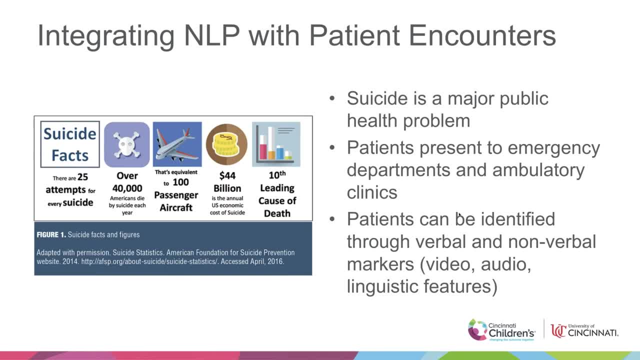 include the patients in their own care, and so here's a brief background on suicide, which is? suicide is a major public health problem. um patients with a suicide attempt have frequently presented to the emergency department or an ambulatory clinic up to two weeks prior to their attempt, and these patients can be identified. 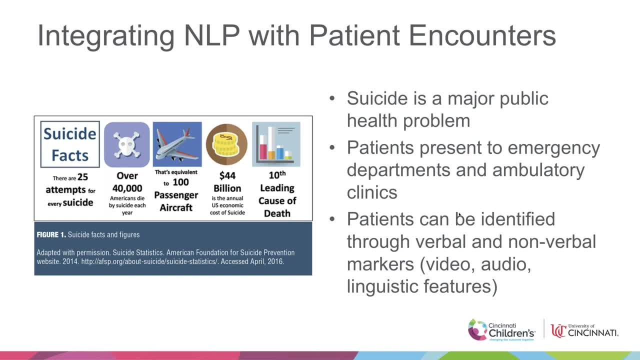 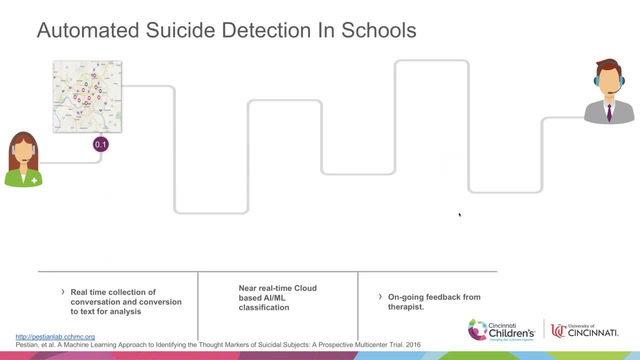 through verbal and non-verbal markers, including video, audio and linguistic features. what i have here on this side to slide to show you is an application built by dr john pestion for automated suicide detection in schools. so john is doing a large multi-center uh trial to predict repeated suicide attempts in adolescence. he uses video. 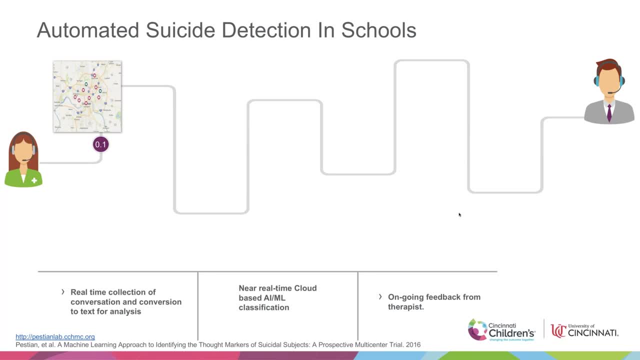 audio, linguistic and genetic features to help predict a patient who may make a repeat suicide attempt. he built a large corpus of suicide notes- about 163- and is working on this larger perspective trial, which is what's in the figure with the cincinnati public school system. so let me show you what's happening, because i don't have any results for this one yet. 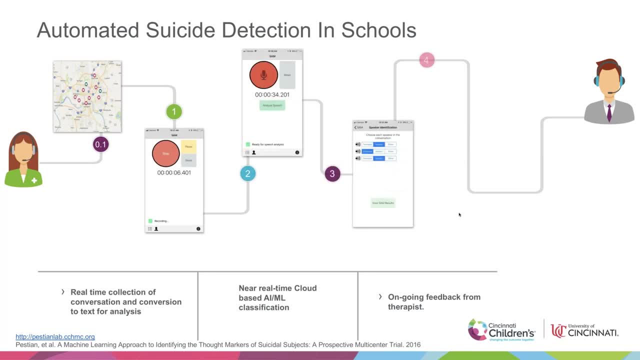 what happens is a therapist or a guidance counselor is able to interview the patient. they can sit and talk to the patient and record the interview, and they use a structured interview typically. then they can perform annotations about who was speaking at each point in time and what was said and what's important and not important in the conversation. all of these data are sent. 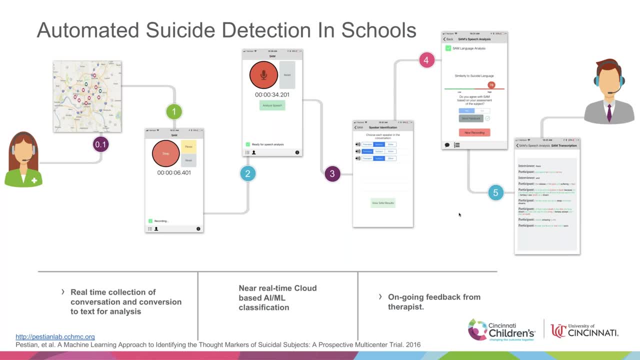 out to a cloud, processed and returned with, basically, a stop light approach to risk. so either they are high risk or they are low risk, and if they're low risk they're more likely to die. if they are high risk, what can we do to provide them? 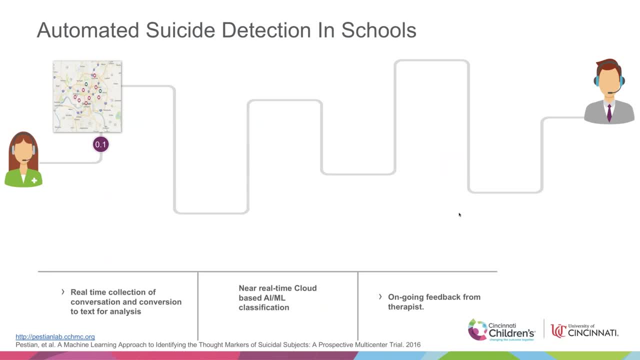 built by Dr John Pestgen for automated suicide detection in schools. So John is doing a large multi-center trial to predict repeated suicide attempts in schools And he's doing a large multi-center trial to predict repeated suicide attempts in adolescents. He uses video audio. 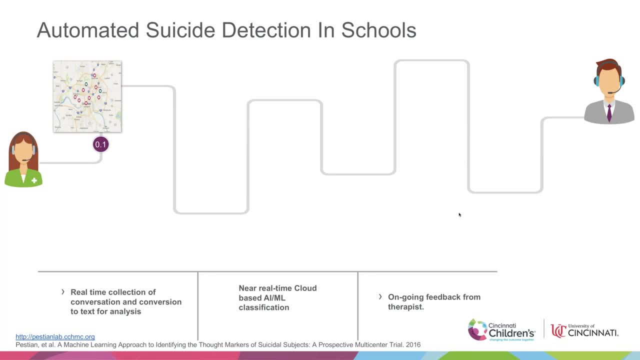 linguistic and genetic features to help predict a patient who may make a repeat suicide attempt. He built a large corpus of suicide notes- about 163, and is working on this larger perspective trial, which is what's in the figure with the Cincinnati Public School System. So let me show. 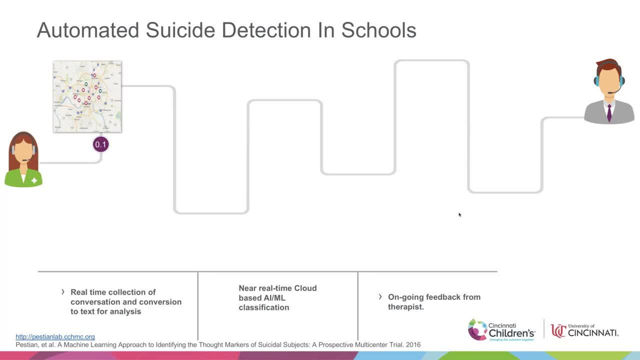 you what's happening, because I don't have any results for this one yet. What happens is a therapist or a guide, and they're trying to predict a repeat suicide attempt. And they're trying to predict a repeat suicide attempt. And they're trying to predict a repeat suicide attempt. They're. 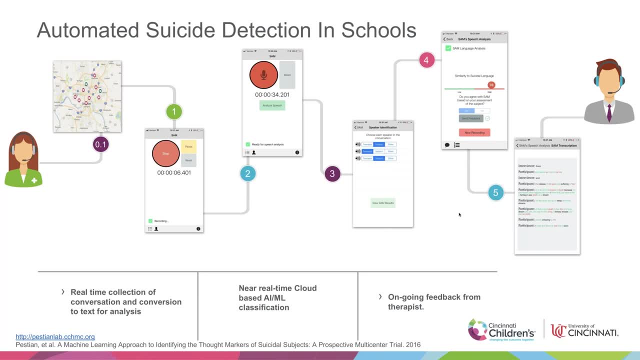 trying to predict a repeat suicide attempt And they're trying to predict a repeat suicide attempt. They could sit and talk to the patient and record the interview, and they use a structured interview Typically. then they can perform annotations about who was speaking at each. 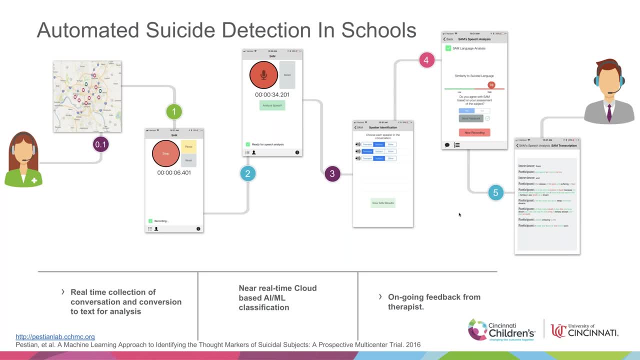 point in time and what was said and what's important and not important in the conversation. All of these data are sent out to a cloud, processed and returned with basically a stoplight approach to risk. So either they are high risk or they are low risk. and if they are high risk, 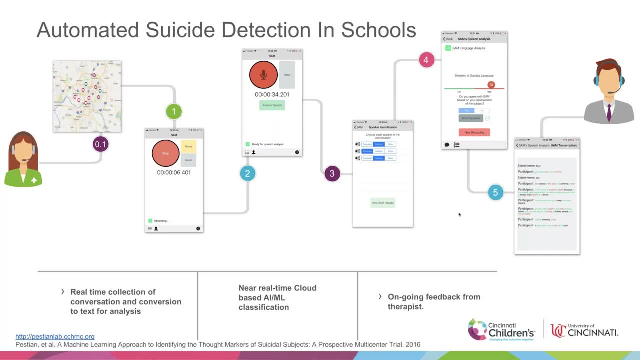 what can we do to fix it? So a lot of people have said I don't have anything to fix, but in my own to provide them with additional resources now to ensure that nothing bad ever happens. This is currently being evaluated in all of the Cincinnati public schools listed on the image. 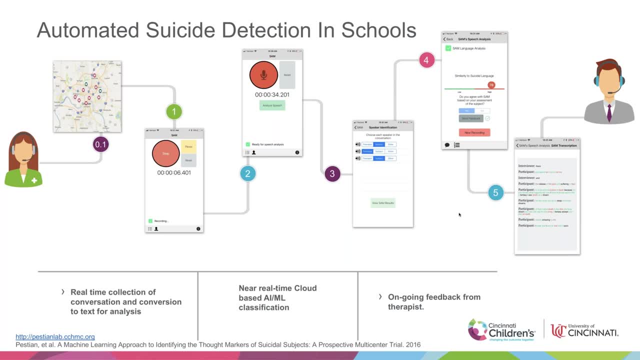 to the left hand side and is working with the guidance counselors there and hopefully we'll have great results by next year to talk about. So this is a great step in involving real-time machine learning, patients and the community all together to help improve some of the care. 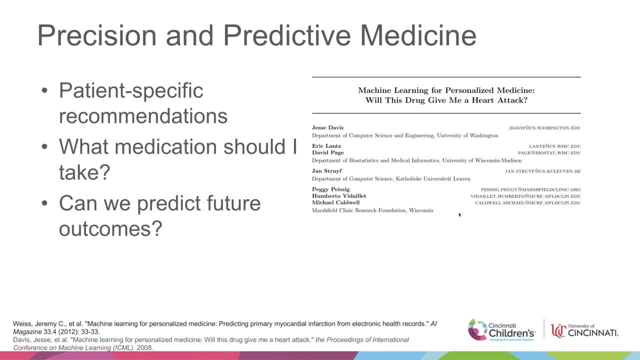 So the other item I wanted to bring up that gets us towards the future approach to the way things are happening is precision and predictive medicine. So what about patient specific recommendations? One of these is: you know, will this drug give me a heart attack? 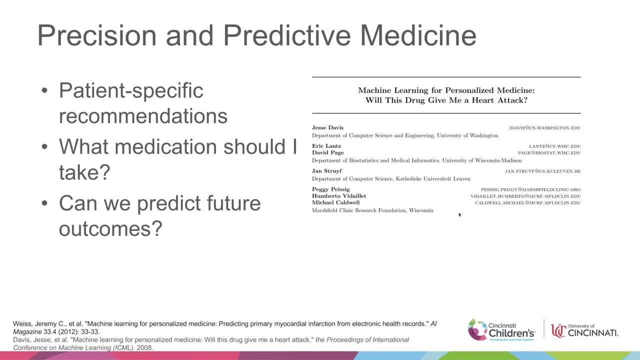 I've picked two papers here. One is from 2008,, one is from 2012.. So this isn't necessarily new research. it just needs to be expanded upon and continue to improve, and especially in pediatrics. What about the idea of what medication should I take? And so precision. 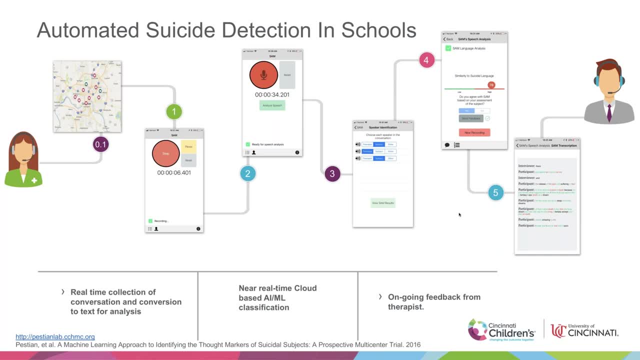 with additional resources now to ensure that nothing bad ever happens. This is currently being evaluated in all of the Cincinnati public schools listed on the image to the left hand side and is working with the guidance counselors there And hopefully we'll have great results by next year to talk about. 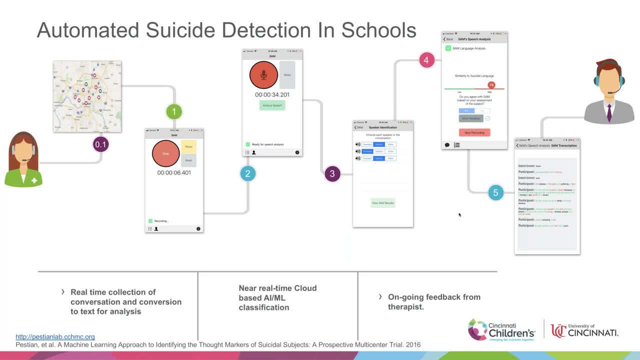 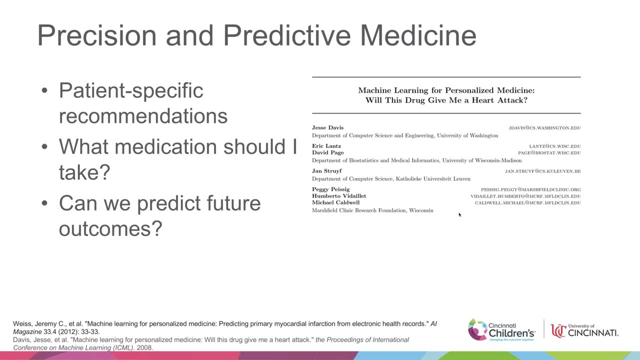 So this is a great step in involving real time machine learning, patients and the community all together to help improve some of the care. So the other item I wanted to bring up that gets us towards the future approach to the way things are happening is precision and predictive medicine. 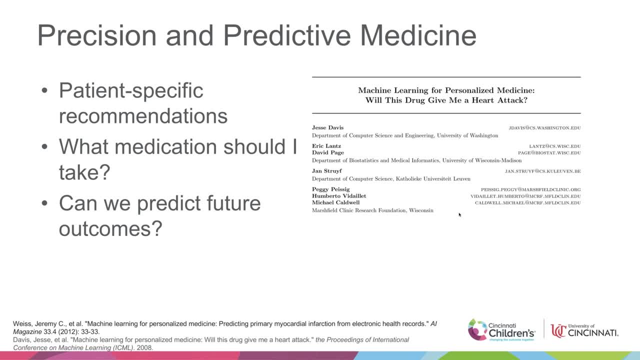 So what about patient specific recommendations? One of these is: you know, will this drug give me a heart attack? I've picked two papers here. one is from 2008,, one is from 2012.. So this isn't necessarily new research. 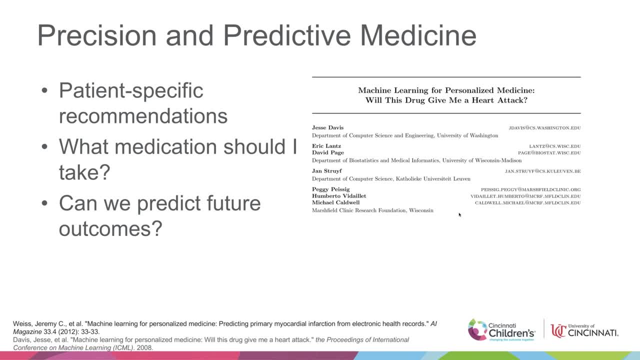 it just needs to be expanded upon and continue to improve, and especially in pediatrics. What about the idea of what medication should I take? And so precision medicine, And so this has been done too on the adult side. So this is, oh, this is the 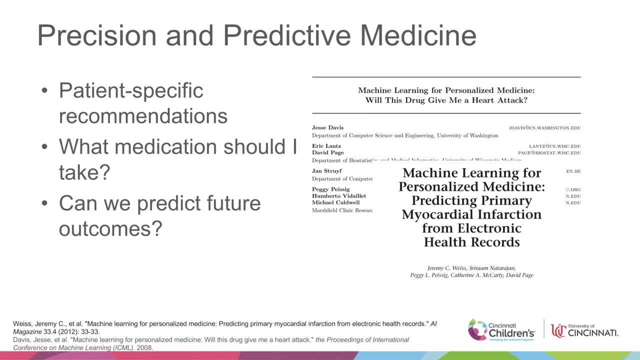 which will this drug give me a heart attack? Then what's the other one Like? can we predict future outcomes from the data we have in the EHR now? And this is the machine learning for personalized medicine predicting primary myocardial infarction? 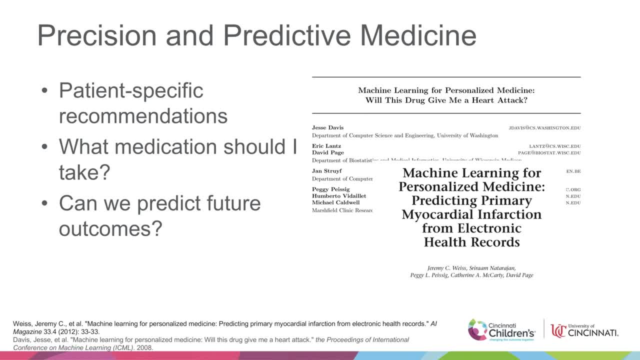 So this is the machine learning for personalized medicine predicting primary myocardial infarction from electronic health records. This particular case is not a great example for pediatrics, because there aren't a lot of MIs in pediatrics, but there are other things that we could predict as well. 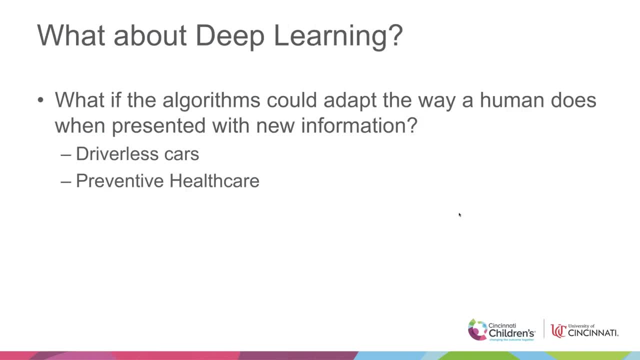 So these avenues are actually best served by something like deep learning, which does prediction and additional recommendations directly to the patient and or their provider. So the answer is: what if the algorithm could adapt to the way a human could? So what if we could do it in a more efficient way? 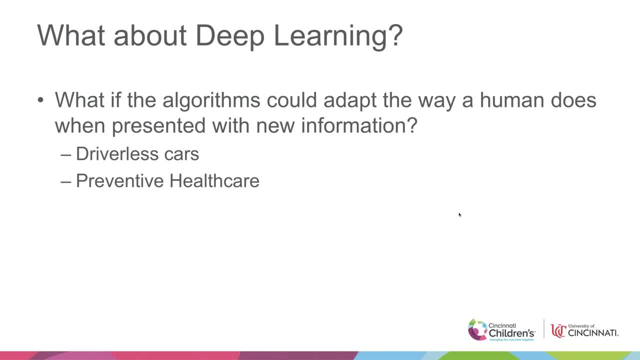 So it could be like a driverless car that can be efficient or providing preventive healthcare. based on all the previous information, What do we need to be able to do these kind of new and interesting things going forward? Well, we need data and we need computing power. 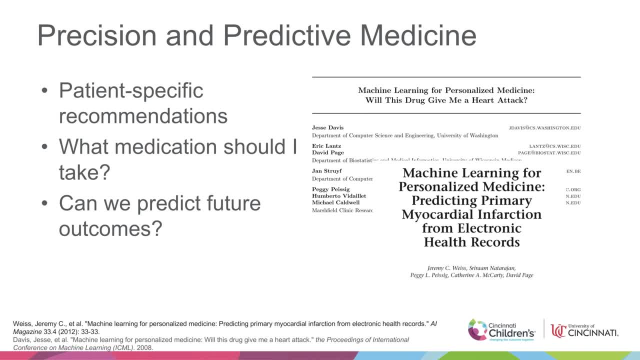 medicine, And so this has been done too on the adult side. So this is, oh, this is the which. will this drug give me a heart attack? Then what's the other one Like? can we predict future outcomes from the data we have in the EHR now? And this is the machine learning for? 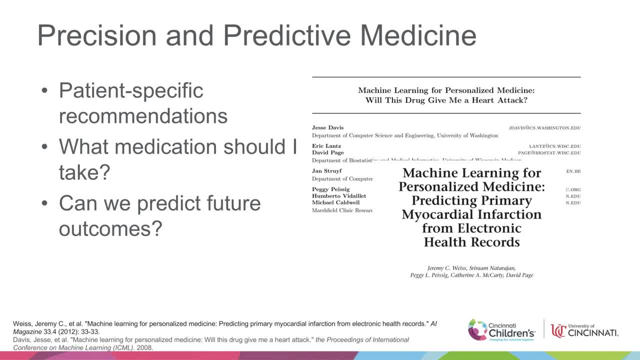 personalized medicine predicting primary myocardial infarctions from electronic health records. This particular case is not a great example for pediatrics, because there aren't a lot of MIs in pediatrics, but there are other things that we could predict as well. 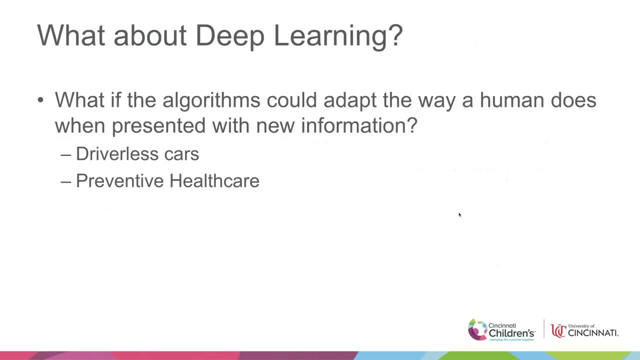 So these avenues are actually best served by something like deep learning, which does prediction and additional recommendations directly to the patient and or their provider. So the answer is: what if the algorithm could adapt the way a human could when presented with new information, So like a driverless car that can be efficient or providing preventive healthcare based on all? 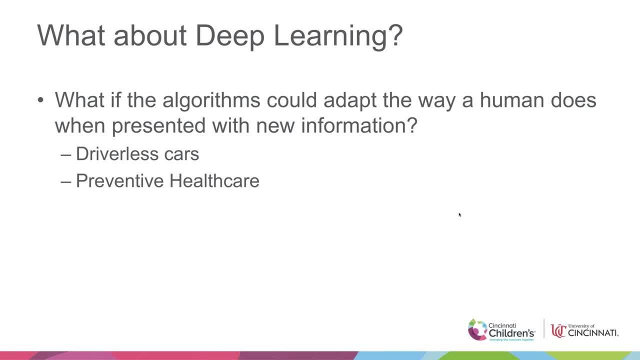 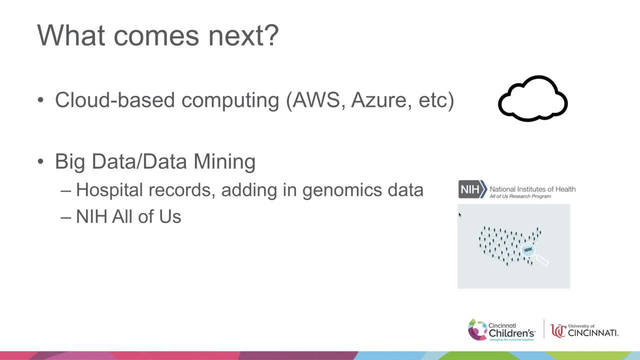 the previous information. What do we need to be able to do these kind of new and interesting things going forward? Well, we need data and we need computing power. The example I put down here was for big data and data mining. One of them is the NIH- All of Us program, which seeks to collect 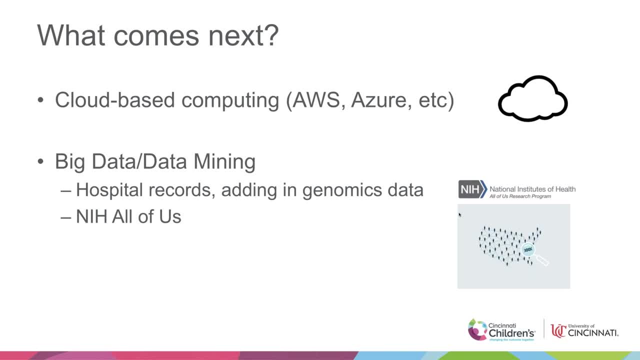 over a million patients and include lots of different pieces of information. They're hospital records, their genomics information, as well as patient surveys, And the idea is that we'll have a large, rich data source to do some of these larger pieces of evaluation and prediction in the 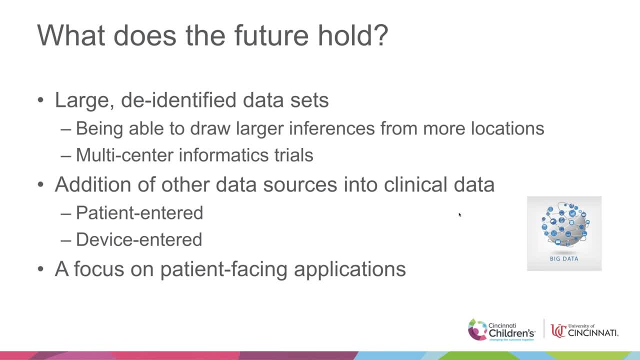 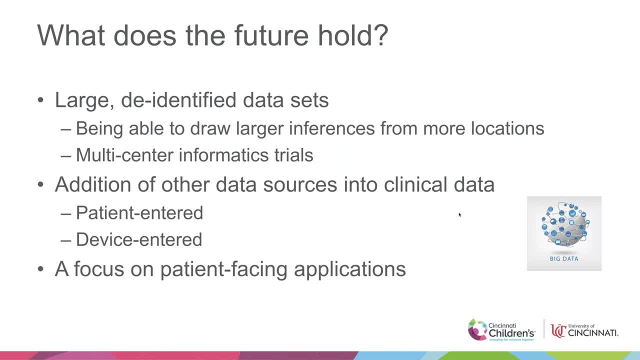 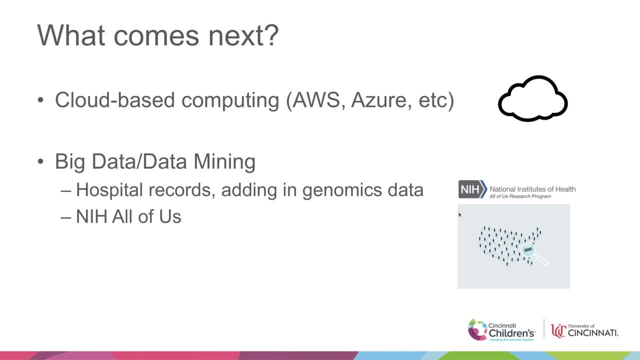 The example I put down here was for big data and data mining. one of them is the NIH All of Us Program, which seeks to collect over a million patients and include lots of different pieces of information: their hospital records, their genomics information. 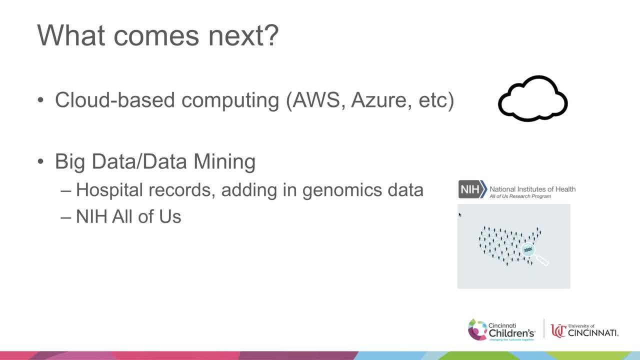 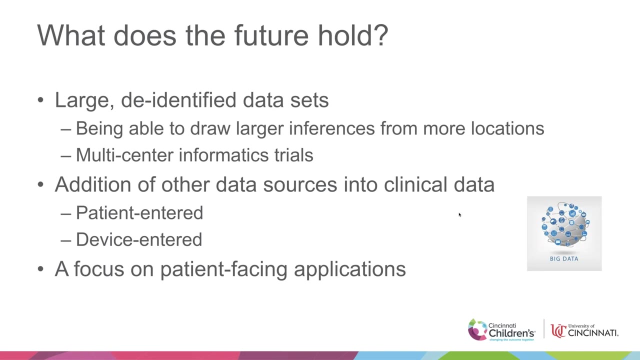 as well as patient surveys, And the idea is that we'll have a large, rich data source to do some of these larger pieces of evaluation and prediction in the future. And so what does the future hold? And, unfortunately, I only really have questions. 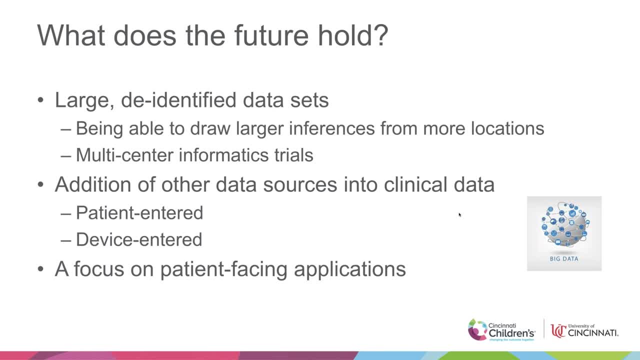 to lead with and not answers. One of these is potentially large de-identified data sets. So we could draw large de-identified data sets. We could draw larger and potentially more accurate inferences if we had larger data sets with more people that were more representative of the entire population. 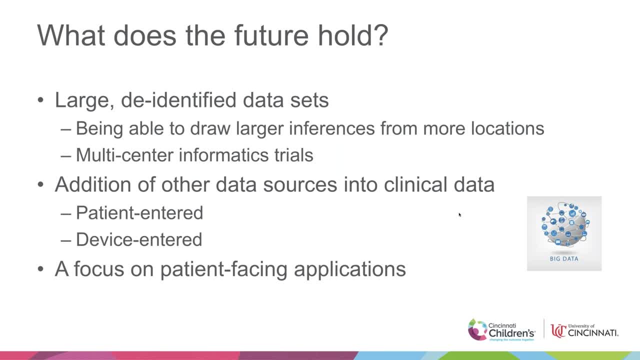 One of the goals with the epilepsy machine learning would be to take it and apply it both to adults and to other pediatric children's hospitals. We know it does a great job here, but can we make it do a great job other places and improve care everywhere? 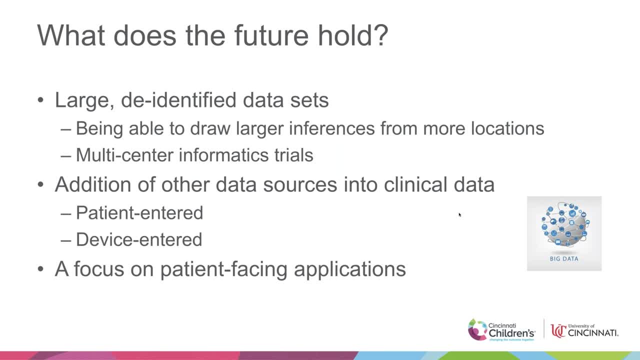 Large de-identified data sets would help us with multicenter informatics trials. They'd help us expand our reach of things we've all developed. Another would be the addition of other data sources into clinical data, so patient-entered data. So I entered a survey in before my care. 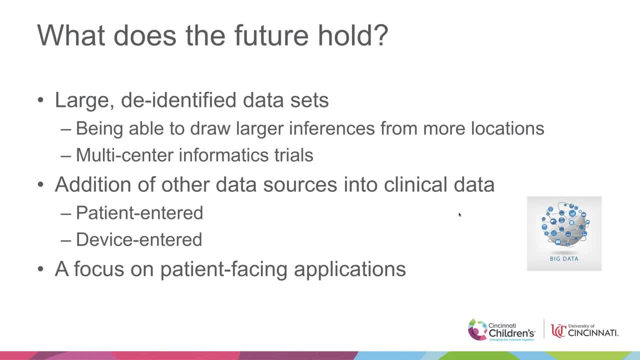 and that should be included as well. Another is device-centered. Those could be medical devices such as your glucose monitoring from your insulin pump, or they could be someone's pedometer data. Maybe these data predict something that we don't know about. 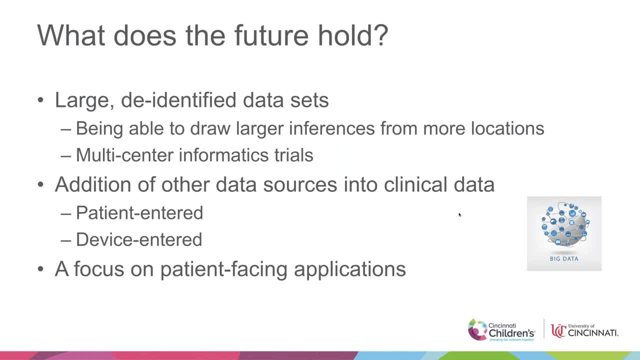 because we don't have large-scale sets of device data combined with electronic data. So that's one of the things that we're trying to do, And then the other would be electronic medical record data, And another one of these would be to focus on patient-facing applications. 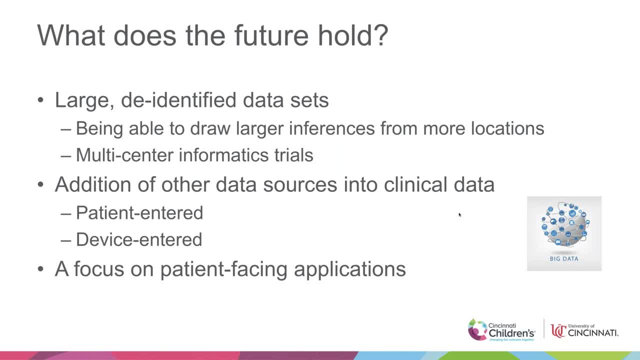 So how can we encourage patients to be participants and stewards in their care and their own health? What else could we design using these larger data sets and using these patients? for what is it that a patient wants on a general day, And how could we make use of some of these upcoming algorithms? 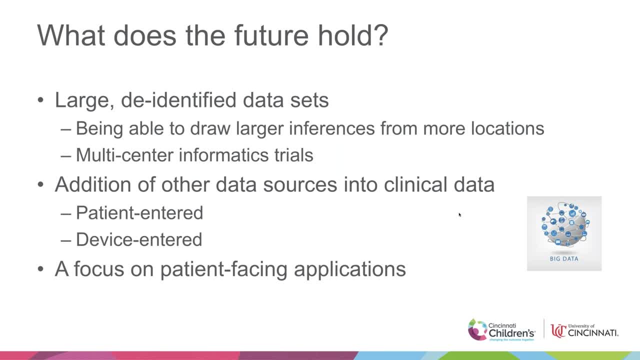 the epilepsy machine learning would be to take it and apply it both to adults and to other pediatric children's hospitals. We know it does a great job here, but can we make it do a great job other places and improve care everywhere? Large de-identified data sets would help us with. 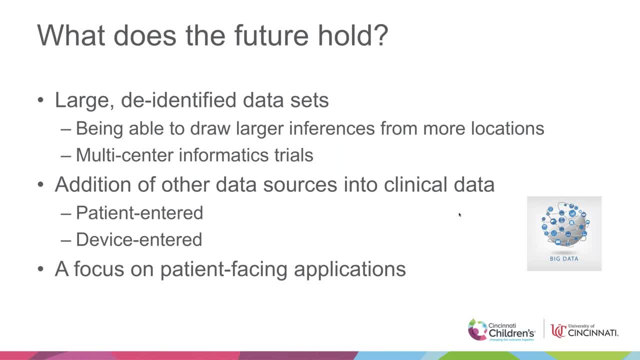 multicenter informatics trials. They'd help us expand our reach of things we've all developed. Another would be the addition of other data sources into clinical data, So patient inner data. So I entered a survey in before my care and that should be included as well. 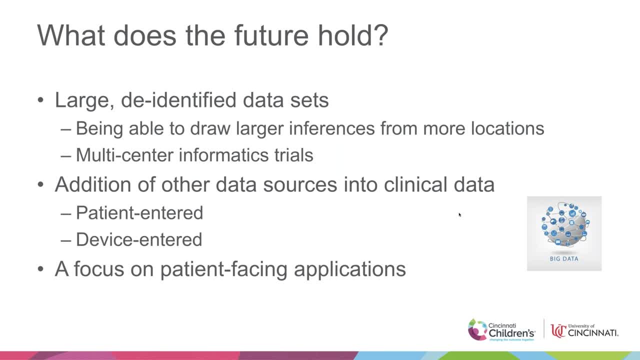 Another is device entered. Those could be medical devices, such as your glucose monitoring from your insulin pump, or they could be someone's pedometer data. Maybe these data predict something that we don't know about because we don't have large scale sets of device data. 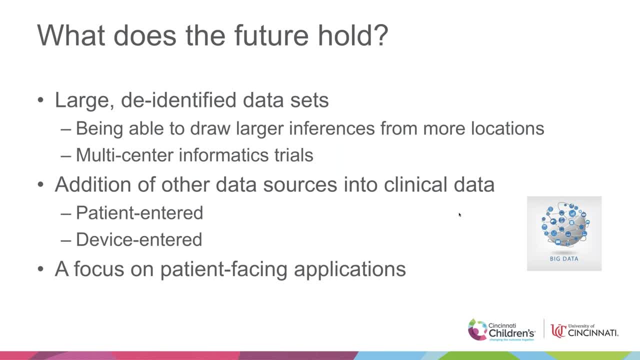 combined with electronic medical record data, And another would be any device acquired. So they look at information all over the world. there might be things that are less than the ice cream, there might be things that are less than the ice powder, and there might be things that build Sketch. 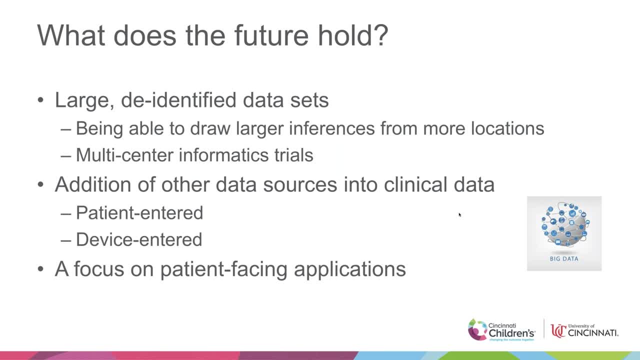 eleri, greater than somebody with a betterBefore-than-eless readings, And to come that you're. And another one of these would be to focus on patient facing applications. So how can we encourage patients to be participants and stewards in their care and their own health? 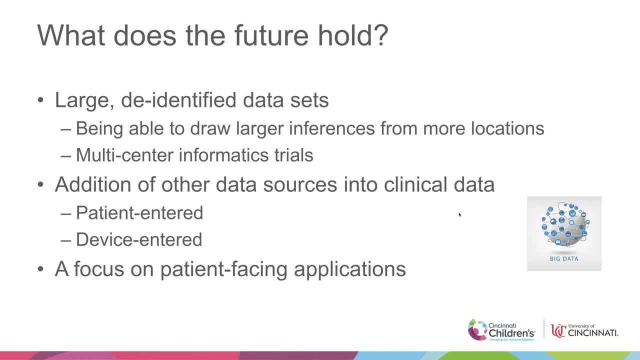 What else could we design using these larger data sets and using these patients? for what is it that a patient wants on a general day, And how can we make use of some of these upcoming algorithms and improve technologies to further clinical informatics research and, ultimately, to improve patient care and health? 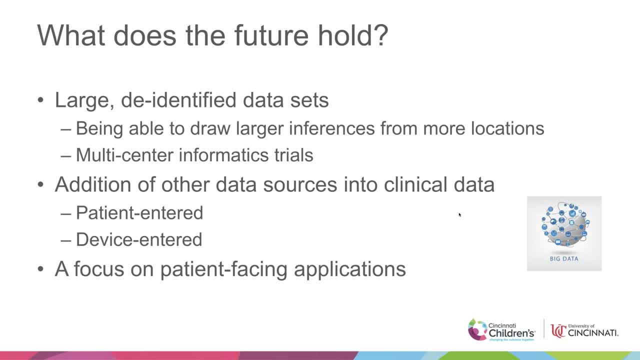 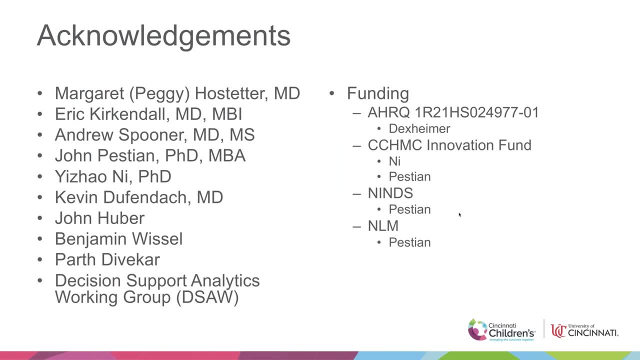 in both the pediatric side and the adult side, And so these are the questions I'm going to leave you with. One of the things I want to point out in all informatics research is that my acknowledgements here barely scratched the surface of the number of people. 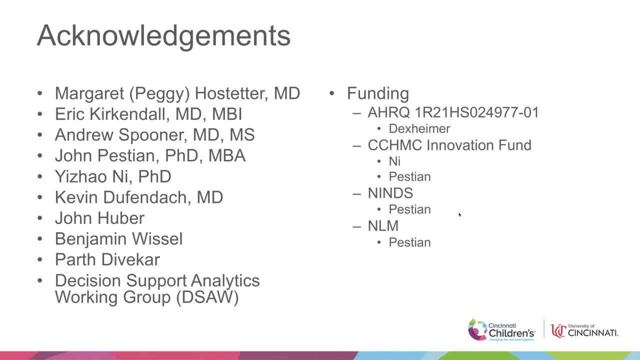 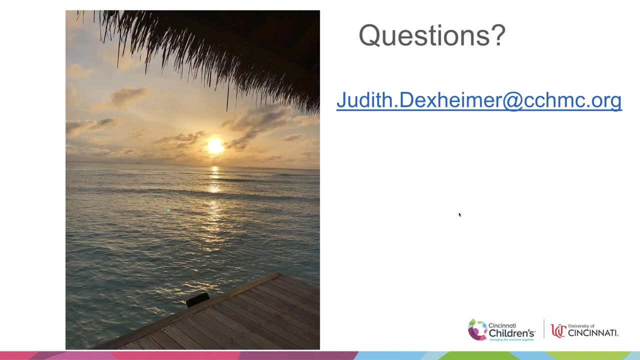 who have talked to me and have helped me with things, And also that you collaborate with across a wide variety of fields to be able to work with not just providers and application developers, but patients and the community And everybody involved, And so I'm open for any questions. 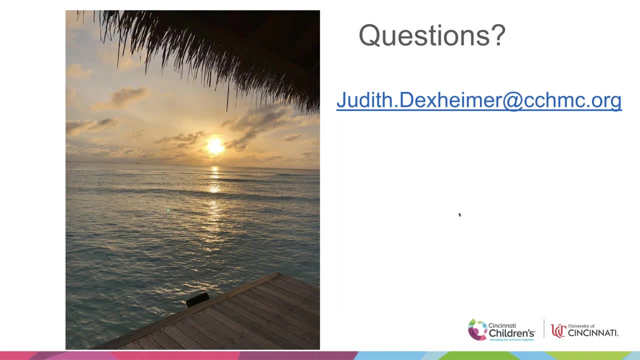 I want to point out that I thought I would be super clever with my slides and have some kind of cloudy, wonderful picture to show how great I was, But I didn't. so this is what you get. So that's it. Are there any questions? 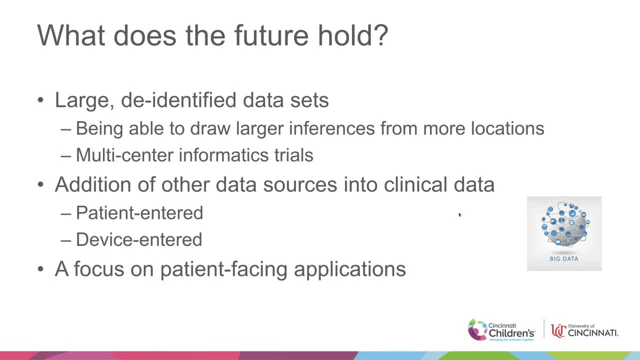 and improve technologies to further clinical informatics research, to improve patient care and health in both the pediatric side and the adult side. And so these are the questions. I'm going to leave you with One of the things I want to point out in all informatics research. 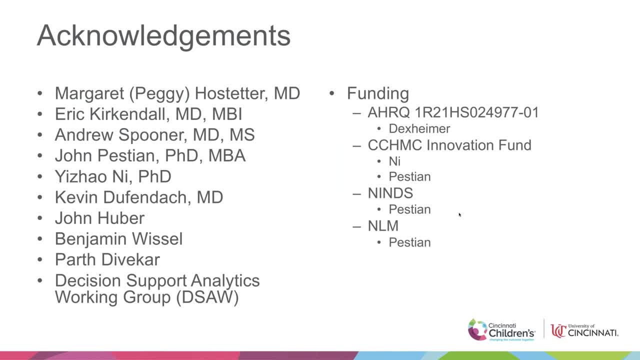 is that my acknowledgments here barely scratch the surface of the number of people who have talked to me and have helped me with things, and also that you collaborate with across a wide variety of fields to be able to work with not just providers and application developers. 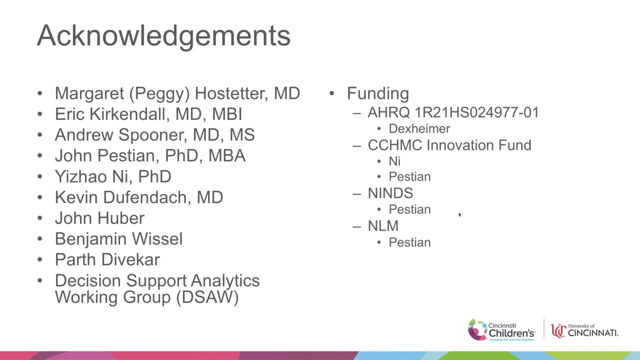 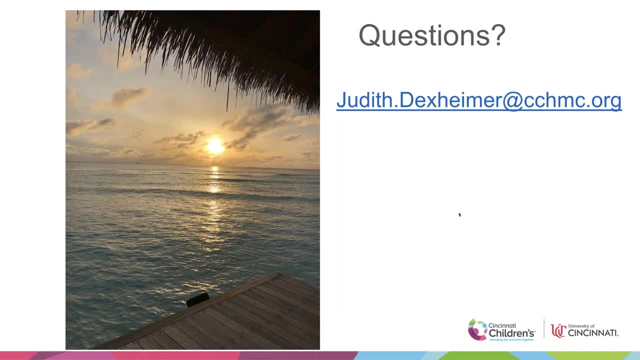 but patients and the community and everybody involved, And so I'm open for any questions. I want to point out that I thought I would be super clever with my slides and have some kind of cloudy, wonderful picture to show how great I was, but I didn't. 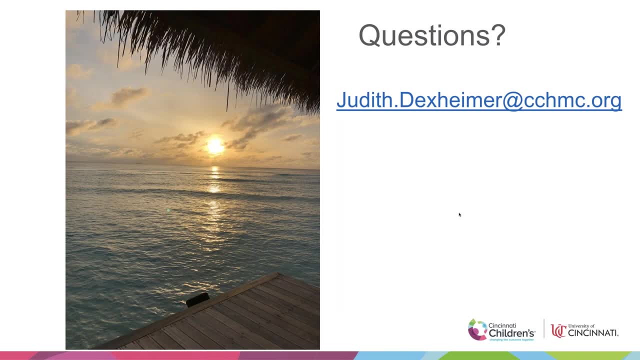 So this is what you get. So that's it. Are there any questions? Thank you, Judith. That was wonderful And yeah, if you guys have questions, please go ahead and enter them. You can always use the Q&A feature to get into the questions. 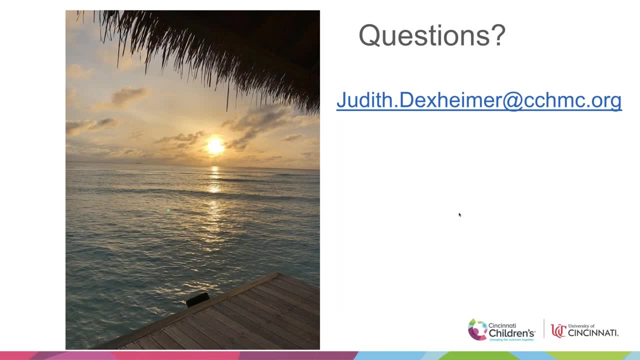 queue on the GoToWebinar control panel. We do have a couple already in the queue. I'll go ahead and read them aloud and give Judith an opportunity to answer. So, Judith, the first question we have is: what program did you write the natural language? 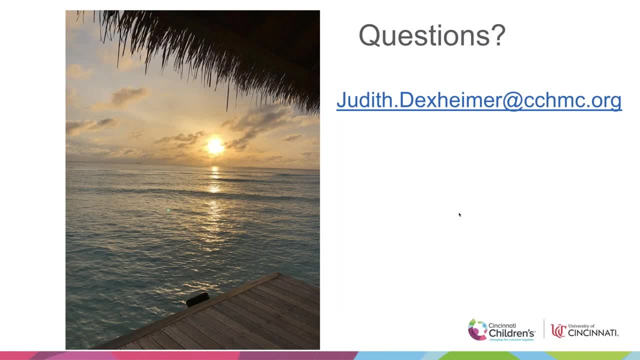 processing script in. So we are in the process of rewriting that script and I think it will end up being in Python in the end. So the answer is, I think, Python, But you can also use the traditional languages, and we're working on cleaning it up a little. 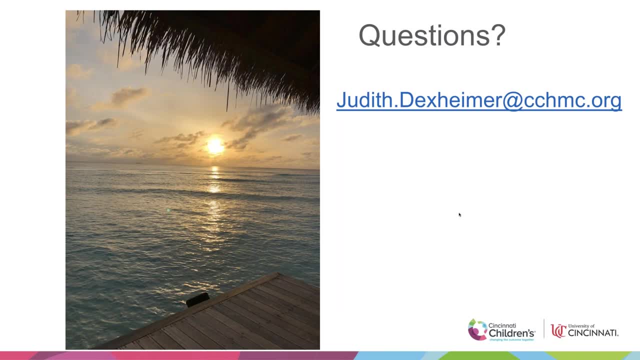 and putting it back together a little, And so the answer I'll give you will be Python Great. Second question is out of curiosity: how are recommendations, slash, predictions from machine learning typically received by physicians, slash patients- they're having a debate, say, with their recommendations from a machine learning. 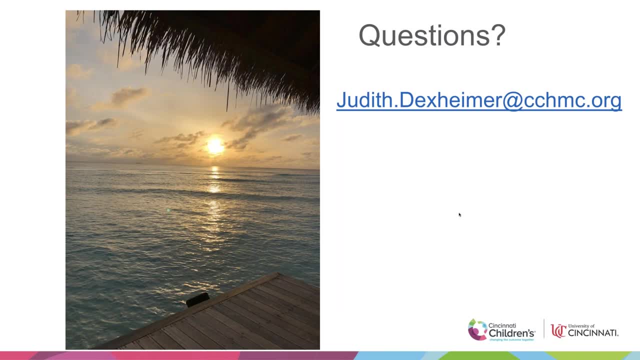 Thank you, Judith. That was wonderful. And yeah, if you guys have questions, please go ahead and enter them into the questions queue on the GoToWebinar control panel. We do have a couple already in the queue. I'll go ahead and read them aloud and give Judith 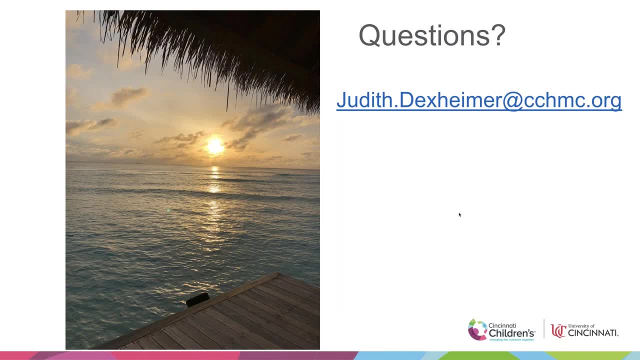 an opportunity to answer. So, Judith, the first question we have is: what program did you write the natural language processing script in? So we are in the process of rewriting that script And I think it will end up being in Python in the end. It was written in two or three different languages, And we're working on cleaning it up a little and putting it back together a little, And so the answer I'll give you will be Python Great. Second question is out of curiosity: how are recommendations slash predictions? 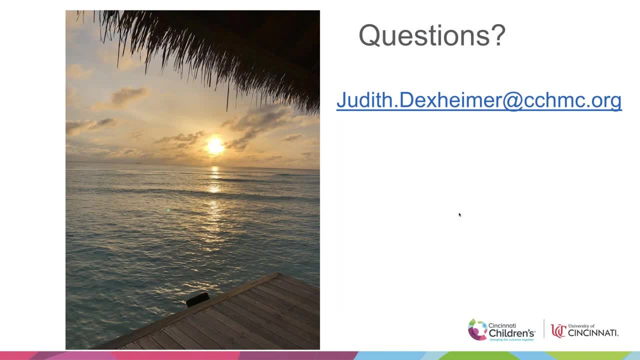 from machine learning, typically received by physicians, slash patients. So so far I have never had a problem with anyone. And they're. I have never had a problem with anyone. And I think what I would say is, having a debate say: 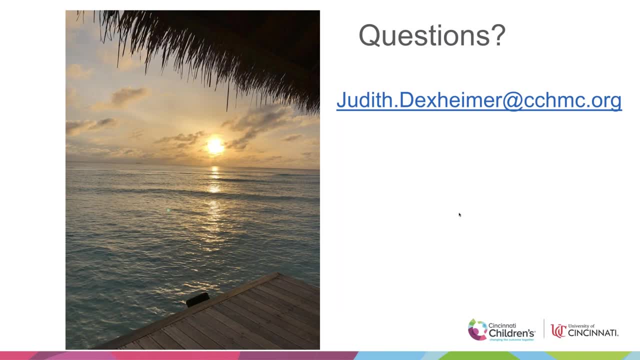 with their recommendations from a machine learning application. I am sure it's coming. I would say that they were generally received well. Frequently one of the issues we have like with the neurosurgical consult is there are other reasons why that patient hasn't. 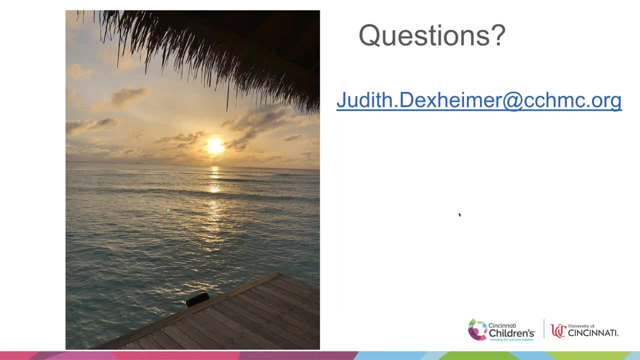 been referred for surgery and they just aren't in the EHR. So if there are social reasons that for any reason aren't there, then that's a good thing. And then there's the other thing, which is that the provider says no, I would never send them. 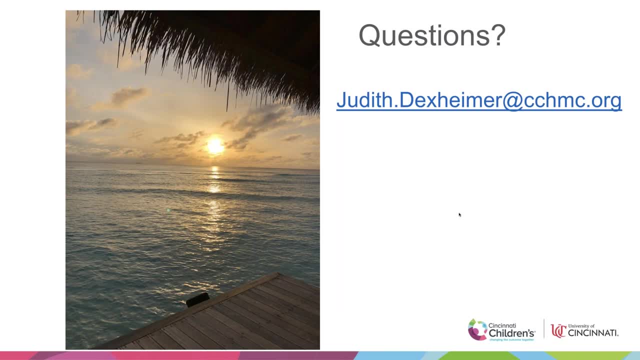 because of x, y and z, But I also might not write that down in the record. And so what we did to combat this for study purposes is we asked them to say: if you want to say no, would you please tell us why? 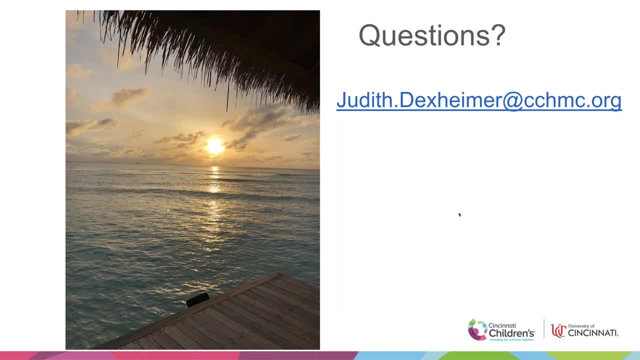 And that way we can design something better going forward. On the patient side, I have not heard of any fallback from patients either, saying I don't agree with this recommendation. The other option, of course, on the suicide application is: we are referring you and ensuring. 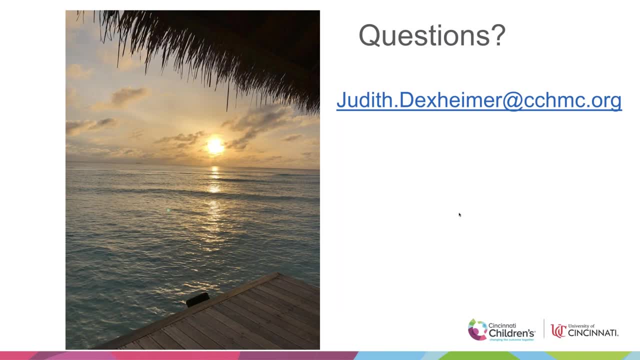 that you get additional resources And so you have a fallback. And you could talk to that therapist and say, on a more personal level, I think it's OK because of x, y and z, And we're out of the picture because all we've done 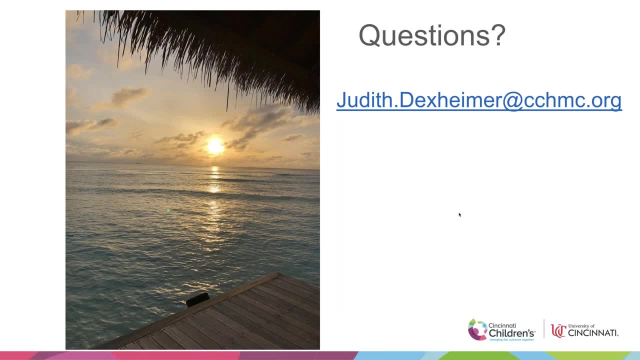 application. I am sure it's coming. I would say that they were generally received well. Frequently, one of the issues we have like with the neurosurgical consult is there are other reasons why that patient hasn't been referred for surgery and they just aren't in the EHR. 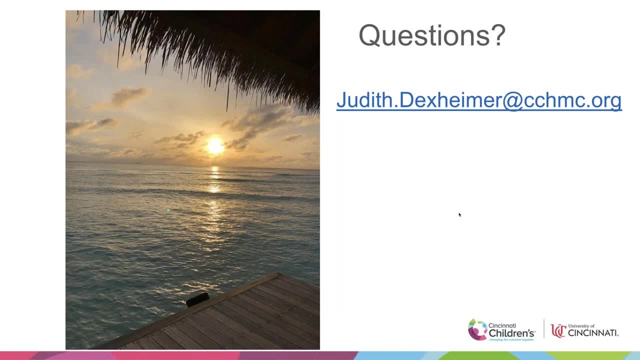 So if there are social reasons that for any reason aren't recorded, then the provider says no, I would never send them because of X, Y and Z, but I also might not write that down in the record. And so what we did to combat this for study purposes is we asked them to say: if you 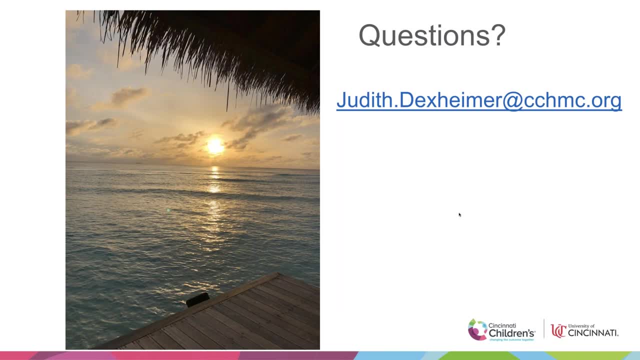 want to say no. would you please tell us why, and that way we can design something better going forward On the patient side, I have not heard of any fallback from patients' either saying you know I don't agree with this recommendation and I don't think this fits me. 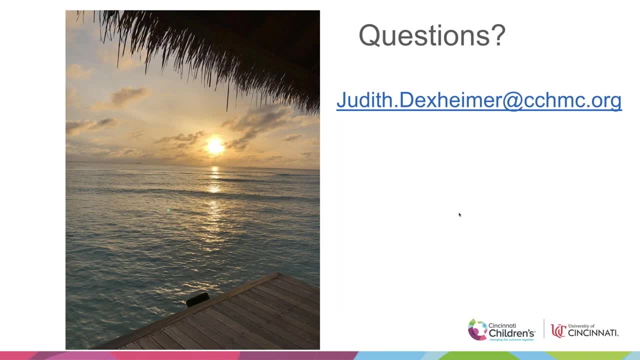 But the other option of course on the suicide application is we are referring you and ensuring that you get additional resources and so you have a fallback and you could talk to that therapist and say you know. on a more personal level, I think it's okay because of X, Y and Z and we're 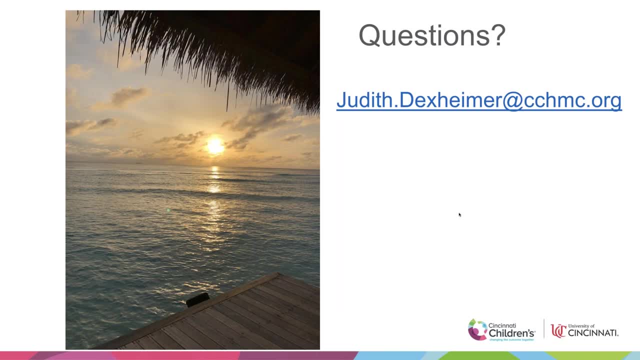 out of the picture, because all we've done is try to send you in the right direction. Great Next question. Next question is how to gather data sets. Are there any public data sets? There are some public data sets, and MIMIC is a public electronic health record. 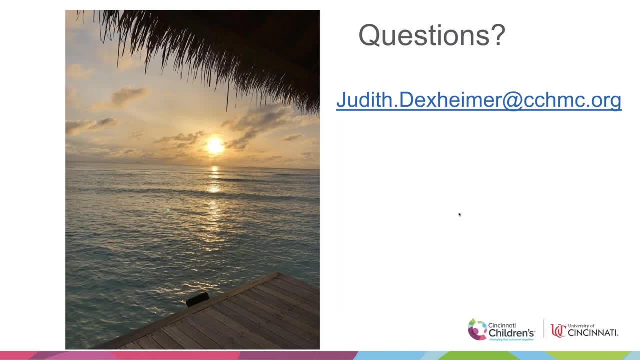 The NIH has several public data sets and there's a lot of research being done on, like the Medicare data, because you can get large amounts of billing data and so you have a great knowledge- and it's pretty accurate- about what was actually done during care. 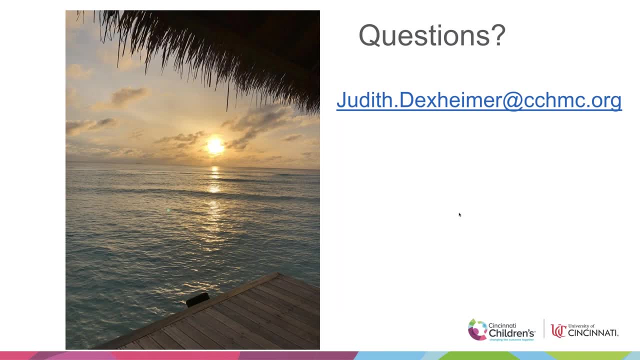 The more difficult thing about gathering large data sets, of course, is the notes, because they're difficult to de-identify, so they're difficult to share publicly. Great Next question is: how about the research on structured data? Are there any opportunities? 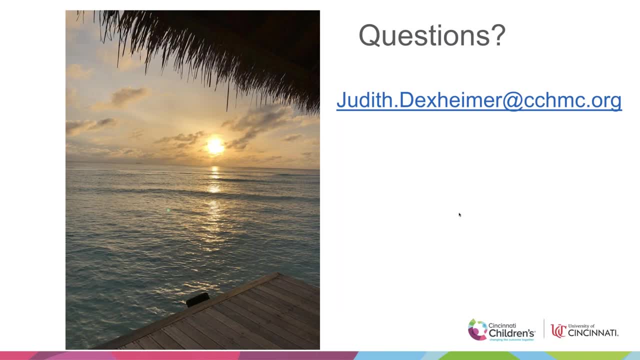 is try to send you in the right direction, Great. Next question is how to gather data sets. Are there any public data sets? There are some public data sets And MMIC is a public electronic health record. The NIH has several public data sets. 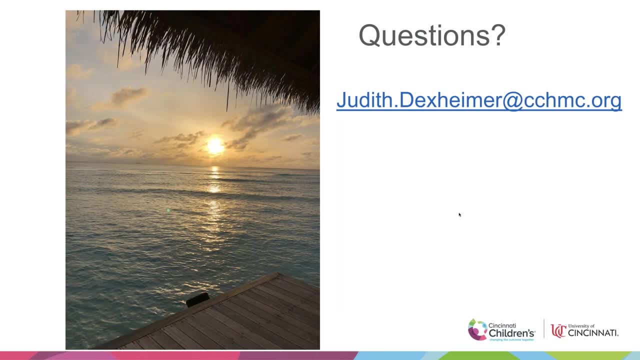 And there's a lot of research being done on the Medicare data, because you can get large amounts of billing data And so you have a great knowledge- And it's pretty accurate- about what was actually done during care. The more difficult thing about gathering large data sets 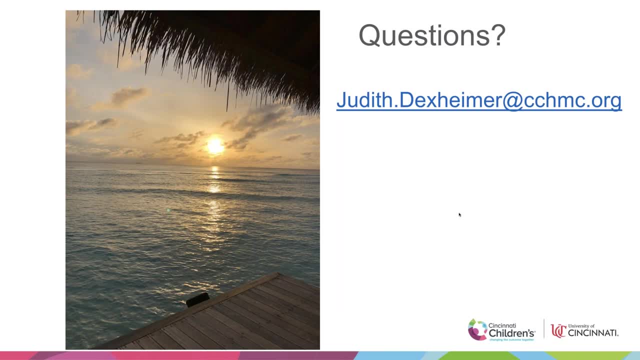 of course, is the notes, because they're difficult to see, They're difficult to identify, So they're difficult to share publicly. Great. Next question is: how about the research on structured data? Are there any opportunities? Yes, There are lots of opportunities for research. 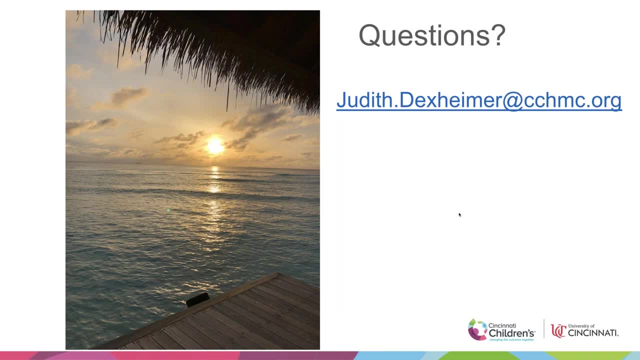 on structured data, And one of my graduate students who has done a lot of work, has also looked into some of the epilepsy pieces with purely structured information to see if it performs as well as better or worse than the natural language processing, as well as there are other published papers using only 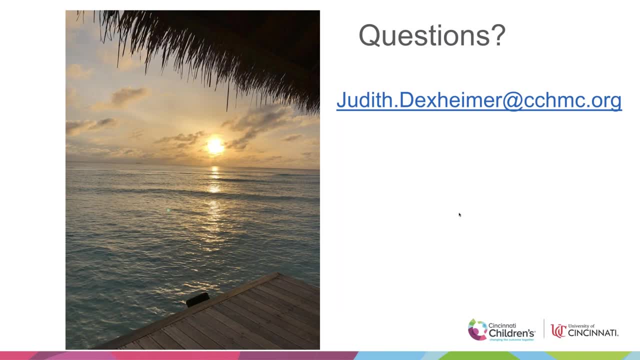 structured data, And one of the great things about structured data is almost everybody has it And almost everybody can access it. Wonderful. This next one is a little long, so bear with me. Security is a big concern today. Can you comment on what steps are being taken and what steps? you envision that need to be taken to protect information as well as to protect the workings of the system itself from attacks such as ransomware? So yes, I can do my best to answer it. One of the ways things are protected on the hospital side. 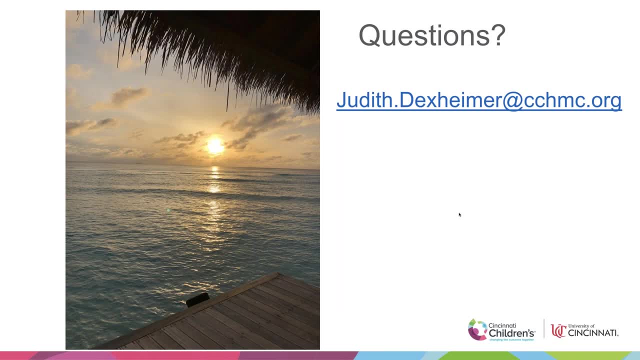 is that we run things entirely within the hospital, And so security is already taken And we're not taking care of. Security is very tight. There is, of course, always a risk. Nothing has a non-zero risk, But there aren't public-facing websites. 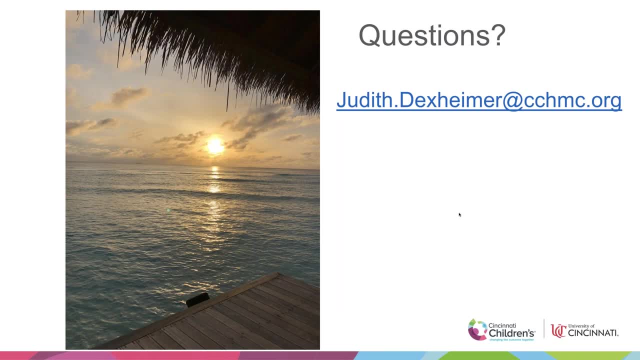 to get things back out of. This is, of course, not going to be as effective of an issue if what we want is public-facing websites to help include the patients in their care. What I can say is that what we have to do is do the best we can for authentication. 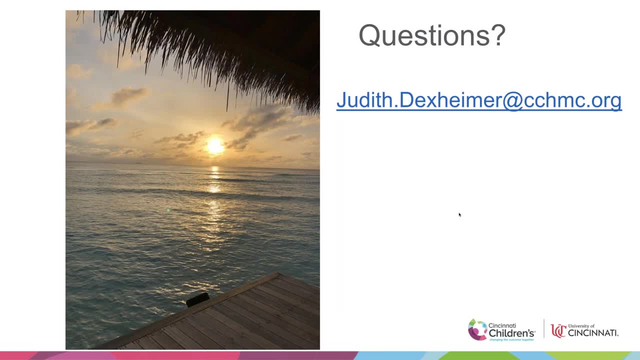 Yes, There are lots of opportunities for research on structured data and one of my graduate students who has done a lot of work has He's also looked into some of the epilepsy pieces with purely structured information to see if it performs as well as better or worse than the natural language processing, as well as there are other. 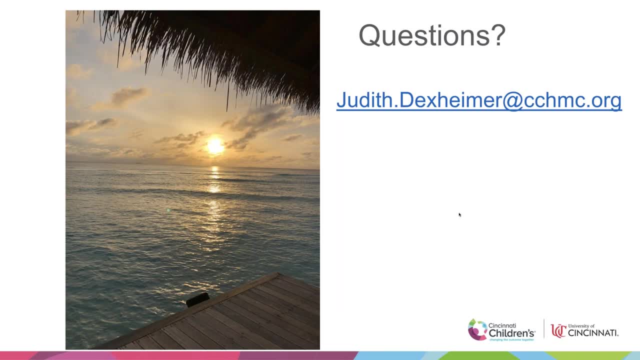 published papers using only structured data, And one of the great things about structured data is almost everybody has it and almost everybody can access it. Wonderful. This next one is a little long, so bear with me. As security is a big concern today, can you comment on what steps are being taken and 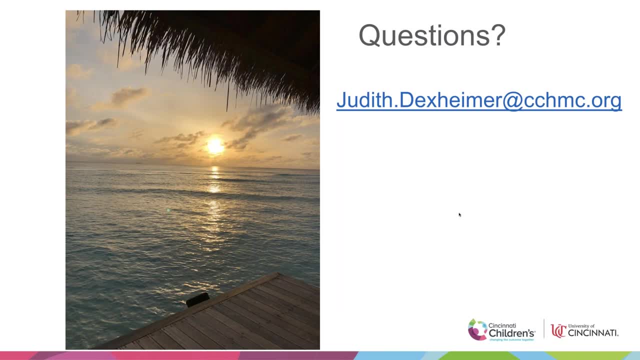 what steps you envision that need to be taken to protect information as well as to protect the workings of the system itself from attacks such as ransomware. So, yes, I can do my best to answer it. One of the ways things are protected on the hospital side is that we all 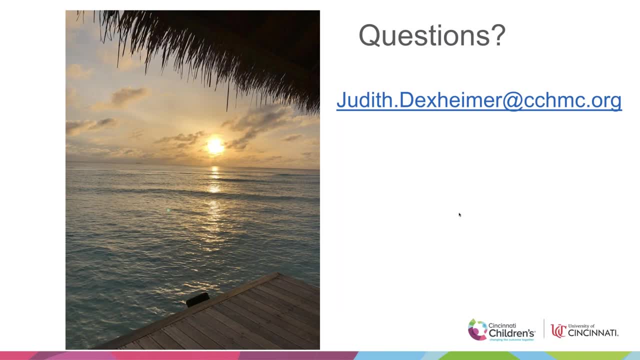 We run things entirely within the hospital, And so security is already taken care of. Security is very tight. There is, of course, always a risk. Nothing has a nonzero risk, but there aren't public-facing websites to get things back out. 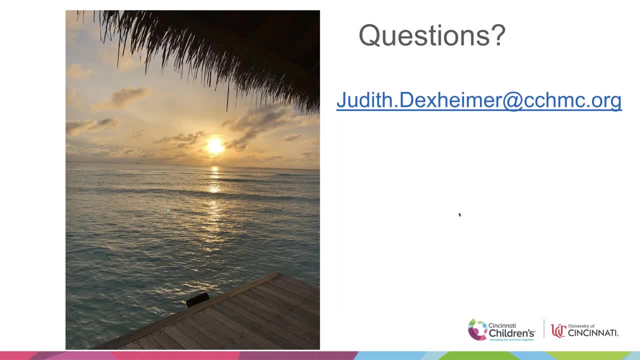 of This is, of course, not going to be as effective of an issue if what we want is public-facing websites to help include the patients in their care. What I can say is that what we have to do is Do the best we can for authentication with the patients and security, and decide what. 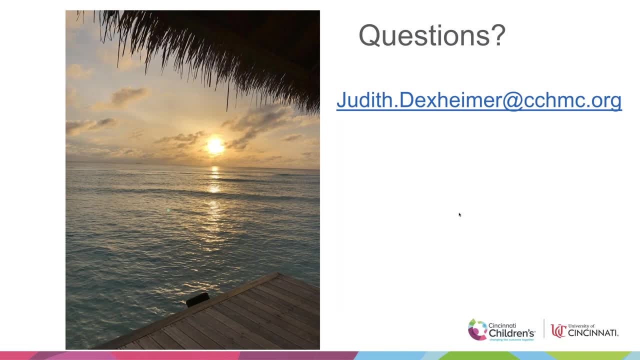 the best way is moving forward to ensure that nothing is ever accidentally shared and at least alleviate those worries. Great, How could you directly involve patients in clinical care with decision-making using algorithms, So Patients can be involved in a lot of different ways? 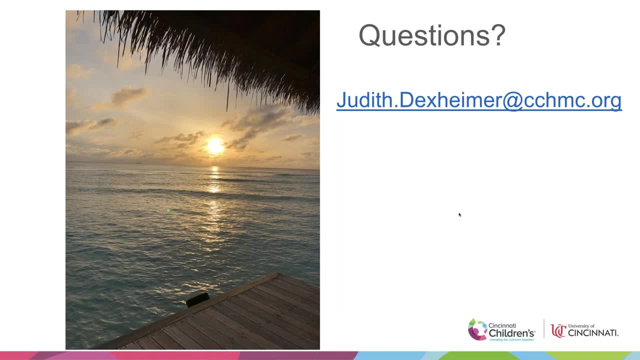 with the patients and security And decide what the best way is moving forward to ensure that nothing is ever accidentally shared and at least alleviate those worries. Great, How could you directly involve patients in clinical care with decision-making using algorithms, So patients can be involved in a lot of different ways? 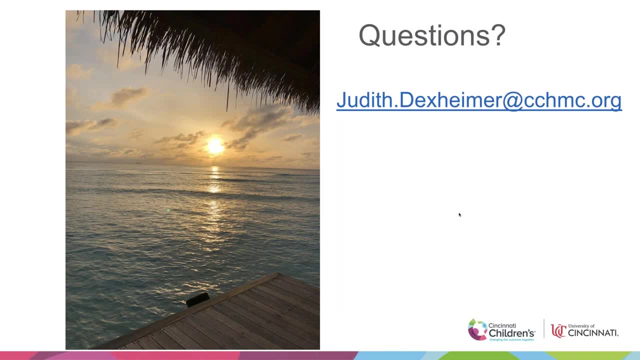 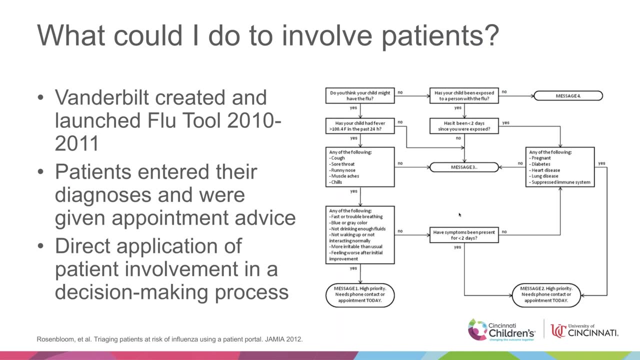 One of the ways they can do this- and I am so happy because I have a slide prepped. So Vanderbilt created this tool called the flu tool that they used in 2010 to 2011.. And they used it with their personal health record. 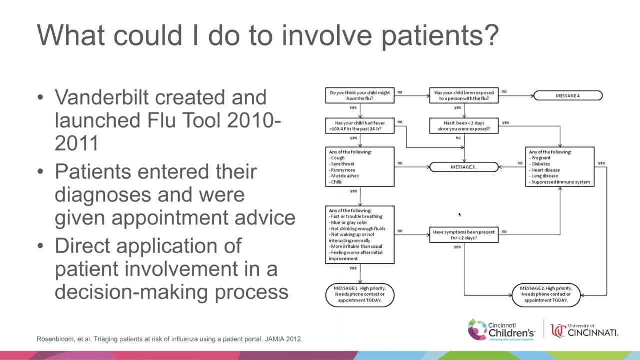 And so patients could enter their diagnoses, They could step through some questions And they could be given whether or not they needed to call and make an appointment. advice- So fairly innocuous advice in an already secure environment, And they could say: I'm having these issues. 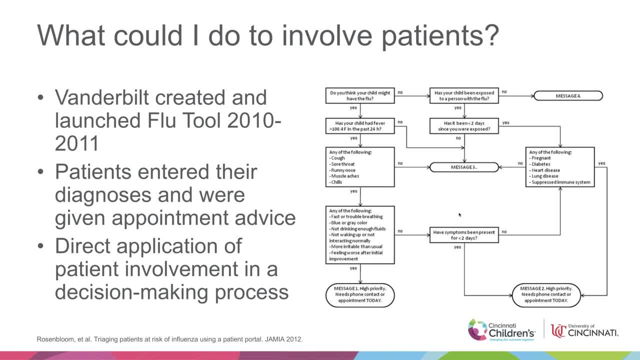 Here's what we think we should do. This is actually a direct application of patient involvement in the decision-making process, Because they also get to make a decision and they need to seek out and find what it is they need, what information they want. 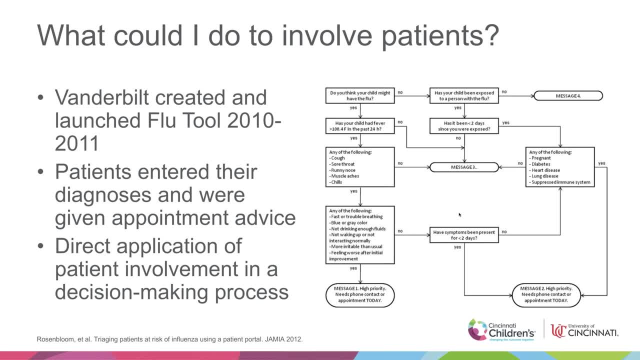 and then decide whether or not they need to call and make a phone call as well. This would be kind of a step before, say, a nurse line, Like I might go through and wanna check all of this information and say, yes, Maybe I do need to call and make an appointment. 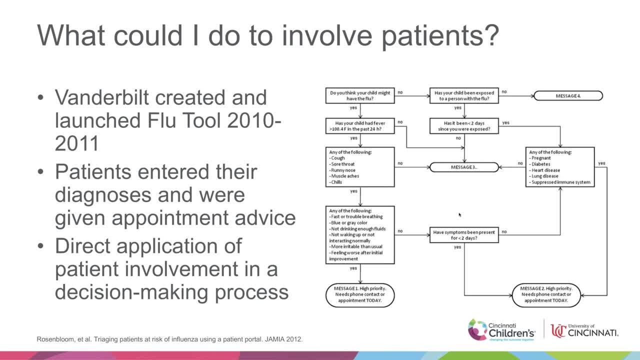 and then call the nurse line and make a decision from there. Or because all of this is Amazon-based. imagine the joy if you could ask Alexa these things And Alexa could say: do you know what? Do you want me to go ahead and call your provider? 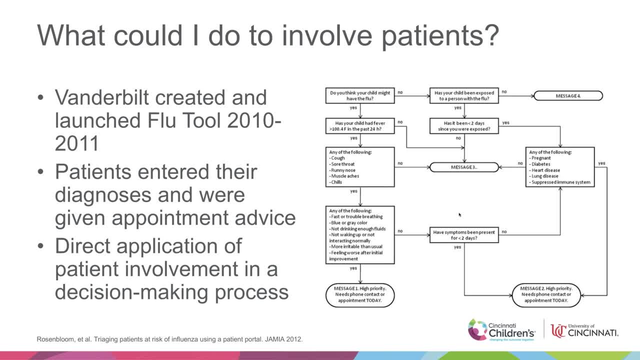 and try to set up an appointment with you And you could say, yes, Fantastic. One more final question and then we'll end the session. How could or should I go about getting into the field of informatics? We always want more people. 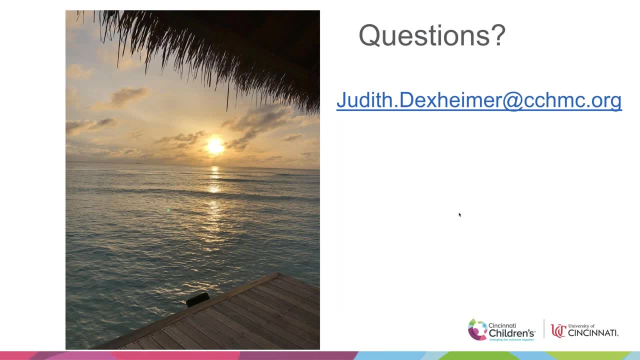 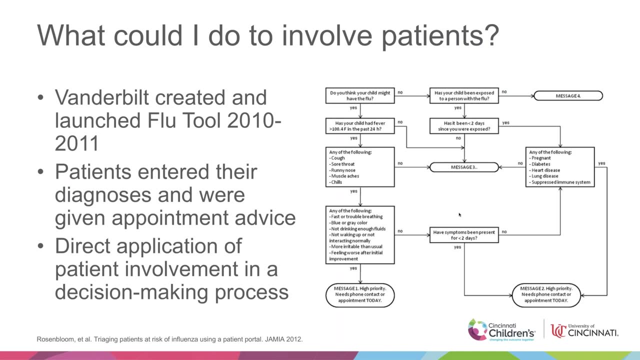 One of the ways they can do this, and I am so happy because I have a slide prepped. So Vanderbilt created this tool called the flu tool that they used in 2010 to 2011,, and they used it with their personal health record. 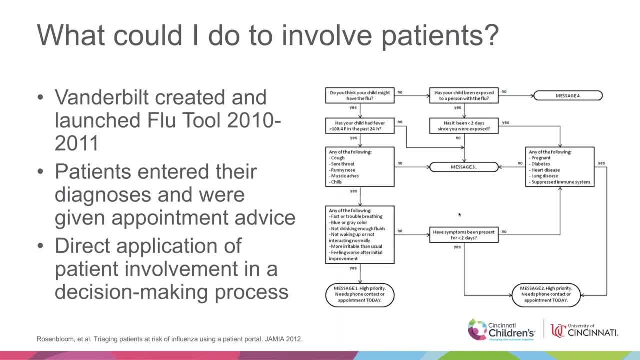 And so patients could enter their diagnoses, they could step through some questions and they could be given whether or not they needed to call and make an appointment advice. So They could have fairly innocuous advice in an already secure environment and they could. 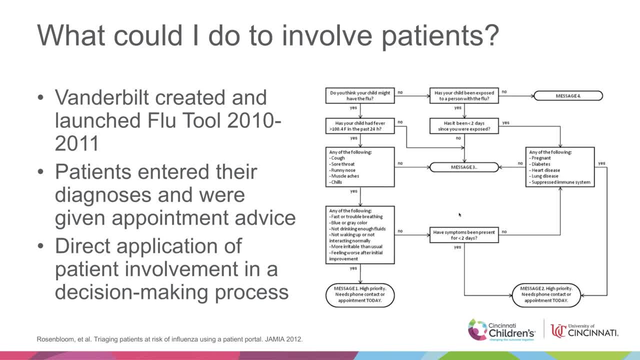 say: I'm having these issues, here's what we think we should do. This is actually a direct application of patient involvement in the decision-making process, because they also get to make a decision and they need to seek out and find what it. 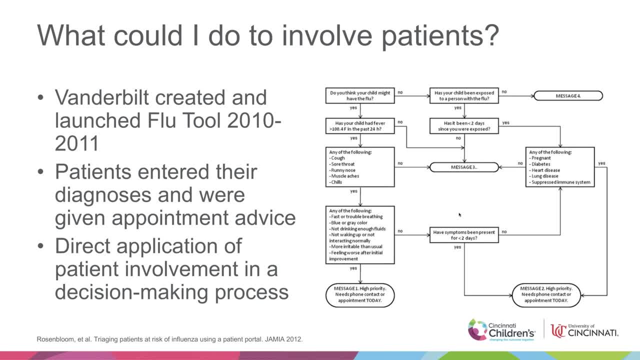 is they need what information they want and then decide whether or not they need to call and make a phone call as well. This would be kind of a step before, say, a patient would call and make a phone call. So If you have a nurse line like I, might go through and want to check all of this information. 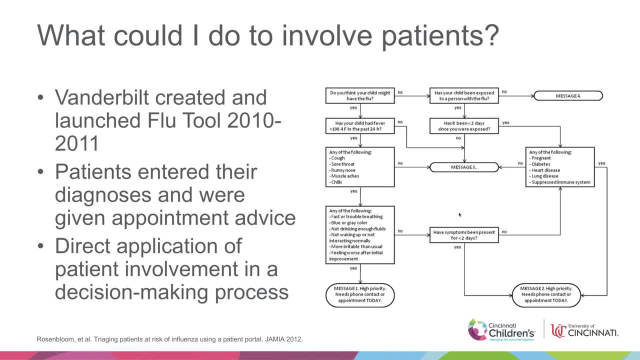 and say, yes, maybe I do need to call and make an appointment and then call the nurse line and make a decision from there. Or because all of this is Amazon based. imagine the joy if you could ask Alexa these things and Alexa could say: do you know what? do you want me to go ahead and call your provider? 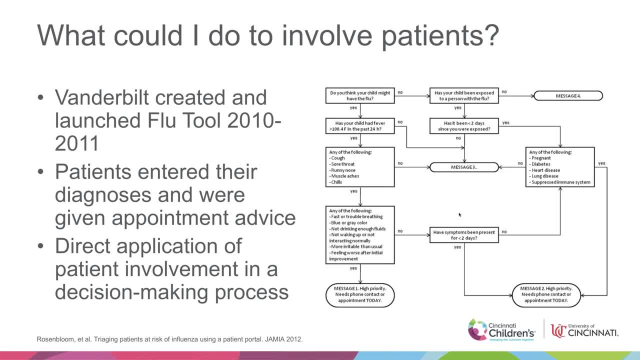 and try to set up an appointment with you And you could say, yes, Fantastic. One more final question And then we'll end the session. How could or should I go about getting into the field of informatics? We always want more people. 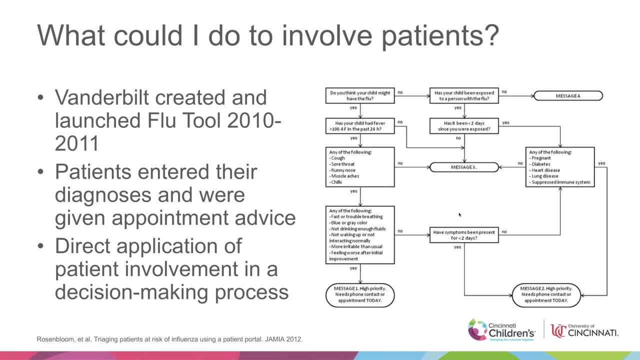 The field is only going to grow as things go, And so if you're starting from the undergrad standpoint, I would suggest looking at both computer science and some of the basic biology courses, which is, I admit, what I did to start towards informatics.